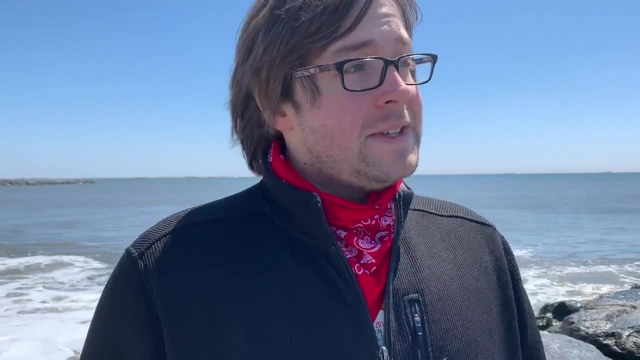 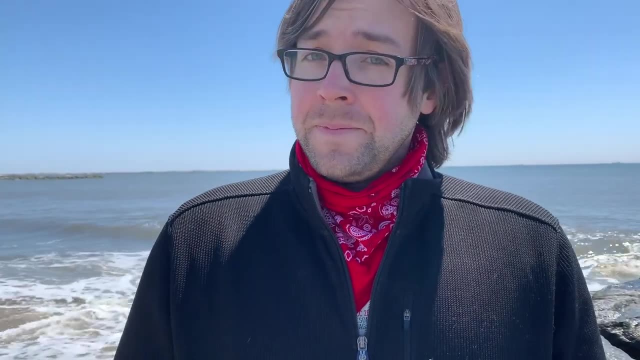 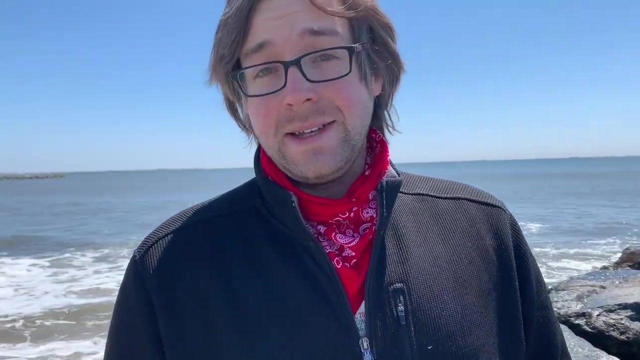 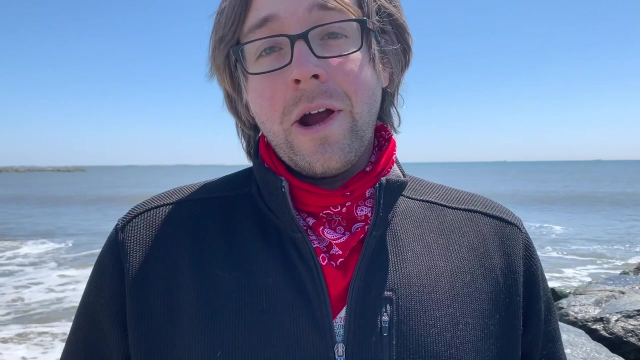 And invertebrates play a very important role in these marine ecosystems, helping to recirculate nutrients, provide food to support water, larger animals and so on. And coral reefs are an immensely important marine ecosystem, So they account for less than a tenth of a percent of marine environments, yet they contain about 25% of the biodiversity that occurs in our oceans. 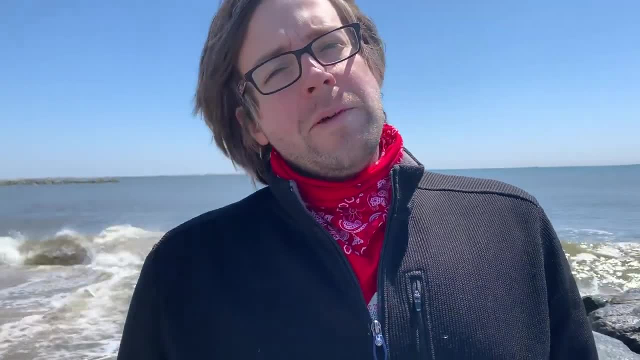 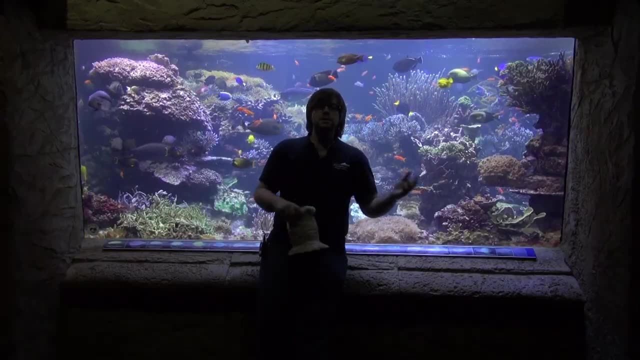 And so that's pretty crazy when you think about it And you know, before we really talk about coral reefs, I think it's kind of important to understand what a coral actually is. Let's take a look. So, in order to answer the question of 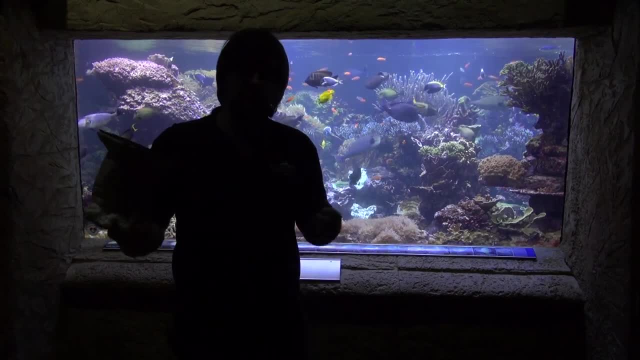 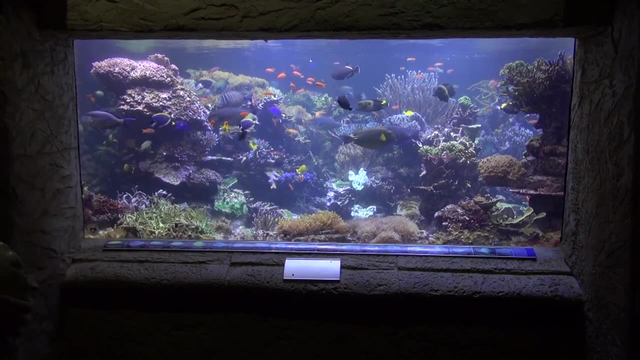 what a coral actually is. I'm here at the crowning jewel of the Long Island Aquarium's Living Collections. This is our 20,000 gallon coral reef exhibit. This habitat is home to hundreds of species of coral and fish from around the world. 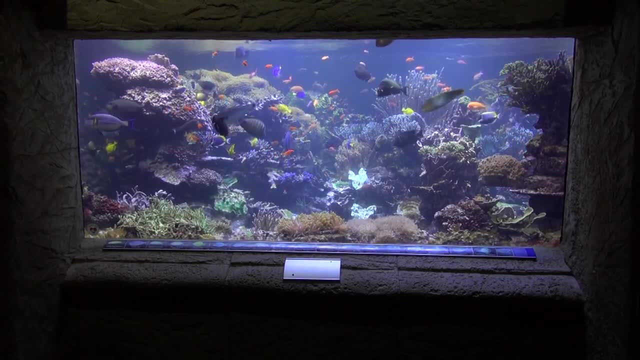 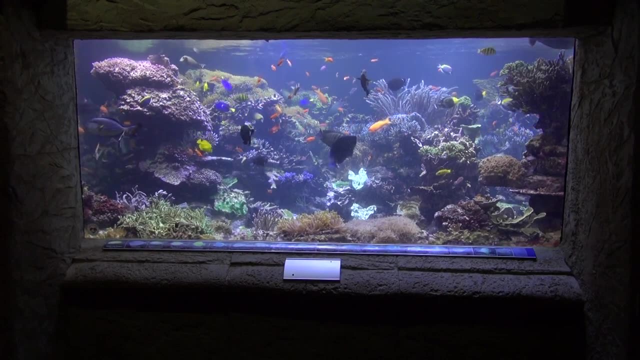 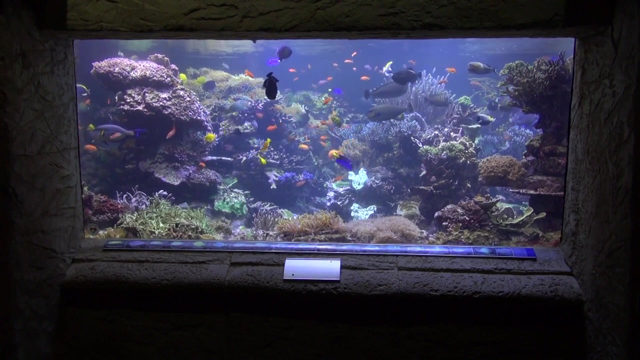 and is one of the largest living coral collections on Earth. This habitat has been maintained by our dutiful aquarists for the 20 plus years since the aquarium's inception, And it is the pride and joy of its creator and our curator and co-founder, Joe Waiulo. 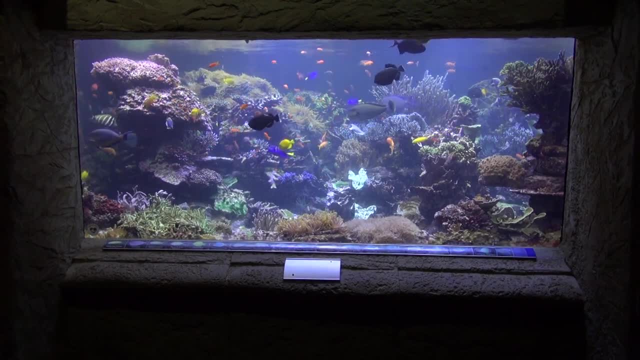 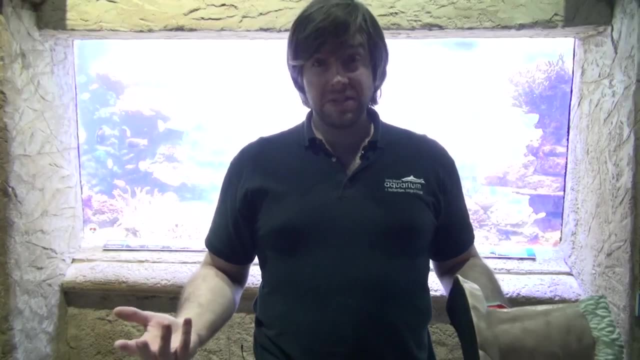 So, because of all of the coral species that are here, I thought what a perfect opportunity to talk about what corals actually are. So, believe it or not, corals are animals. Now, they don't really seem like animals, right? 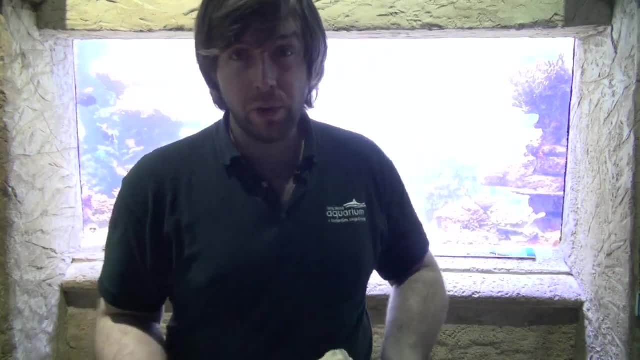 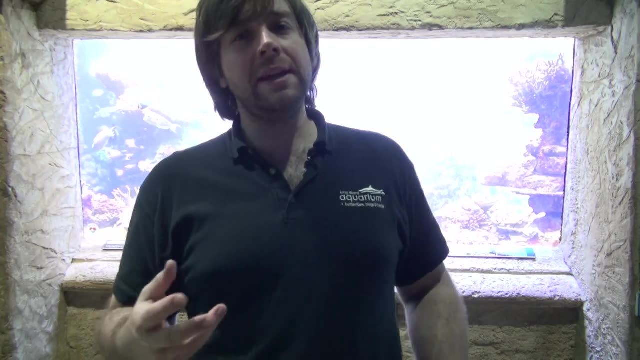 They almost look like they're like plants the way they sit on the ocean floor and they don't really move. But rest assured, they are animals. They're just a very ancient lineage. So it turns out they're pretty closely related to a group of animals you might be more familiar with. 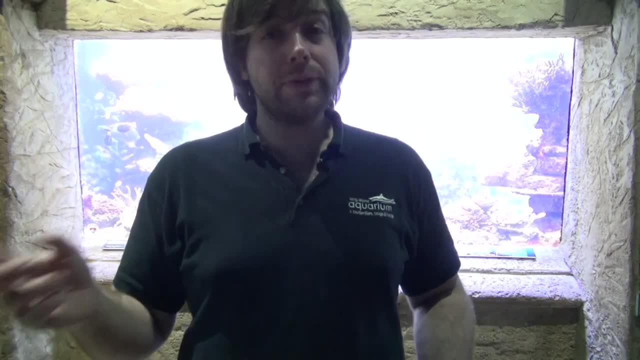 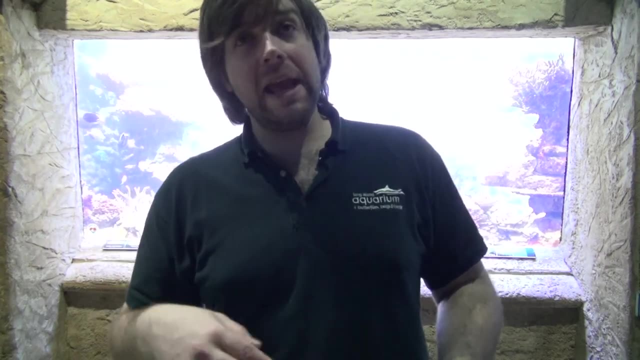 Sea jellies, or so-called jellyfish. Both sea jellies and corals belong to a group of animals known as the Cnidarians. Now, Cnidaria is one of the most ancient phyla of all groups of animals, most simple as well. 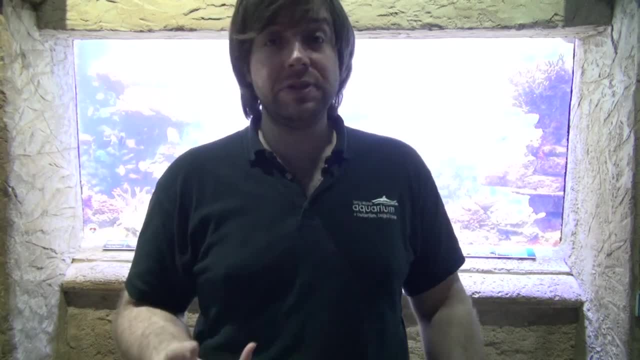 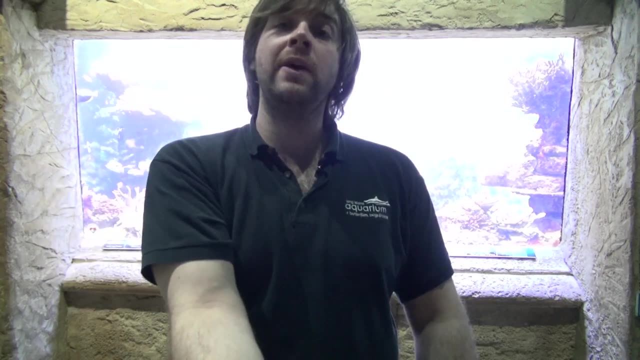 Unlike sea jellies, though, corals don't have a medusa stage. So when you think of a medusa stage, what I'm thinking of is like when you think of a jellyfish: it has that little bell with the little tentacles dangling down right. 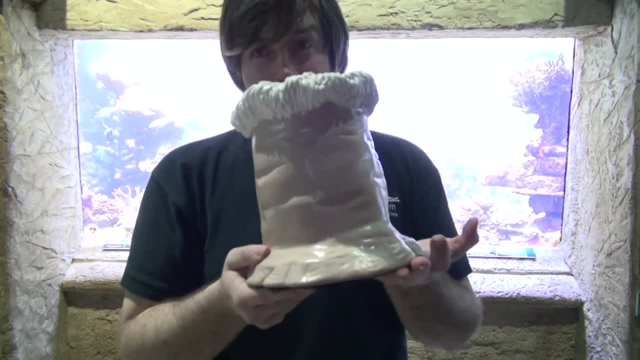 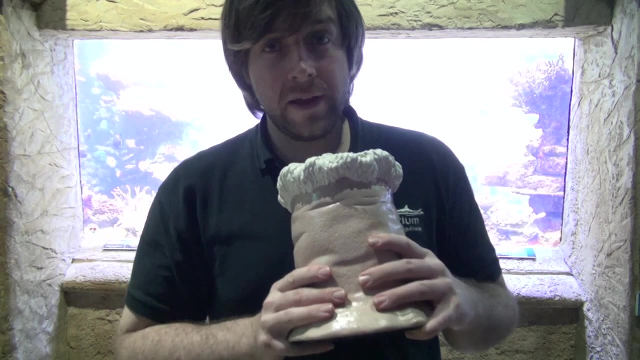 Corals don't have that, though Corals exist as this thing, So this is called a polyp And, basically, when this finds a location that it wants to settle down and situate itself in the ocean, it will remain there. It won't get up and start floating around like a jellyfish does. 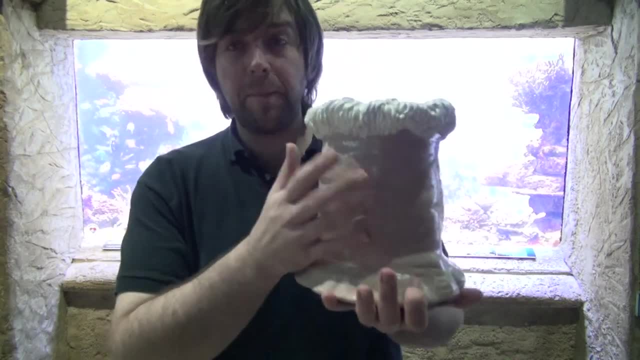 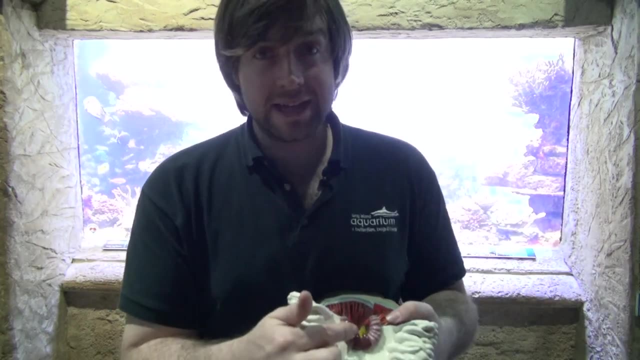 Now, polyps are basically like a. it's almost like a vase or a barrel, And they have a lot of similarities with jellies as well. So they have a single mouth that doubles as an excretory pore, which is a little gross right. 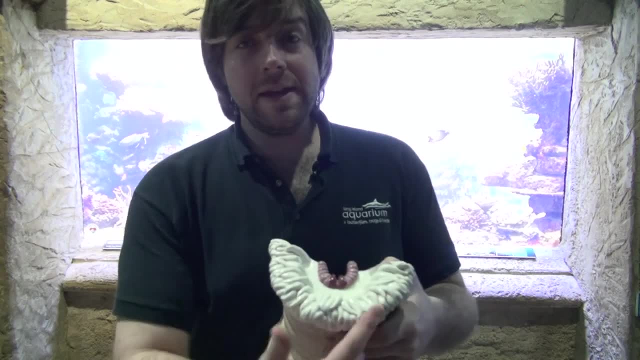 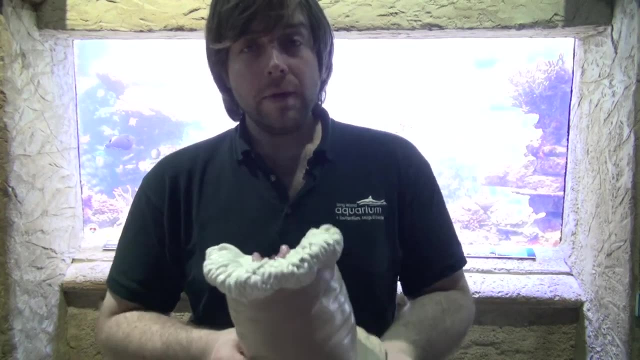 But they're simple animals. They also have tentacles surrounding them, The mouth itself, around the circumference of the polyp. Those tentacles are used for grabbing food and throwing it into their mouth. These polyps also are very small. They're only a few centimeters in diameter, usually from across the top here. 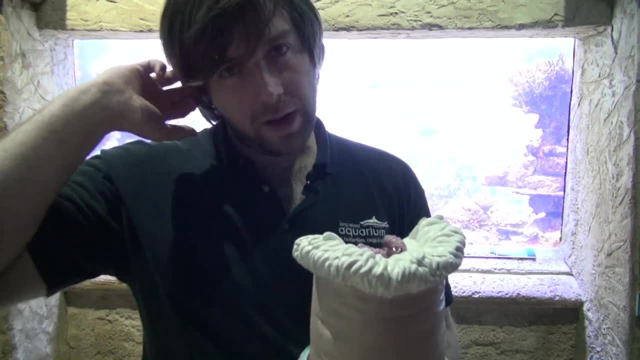 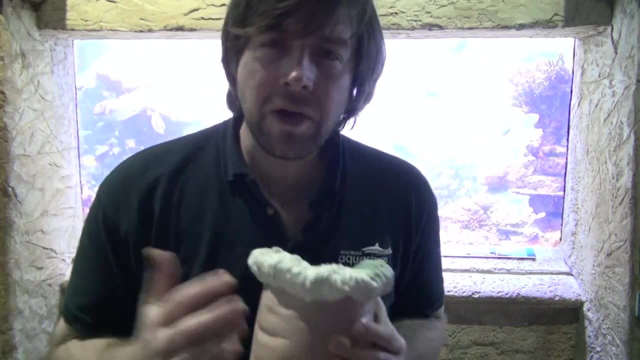 Sometimes as many as five or six inches across in some of the larger species of coral, or larger polyps, I should say, But they're usually pretty small. Now, when you think of a coral, though, I mean, I know I don't really think of this though, right, 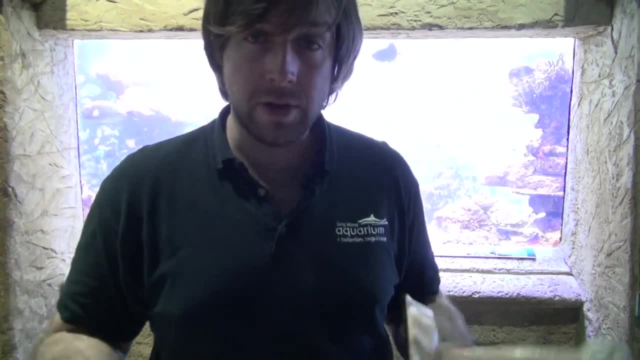 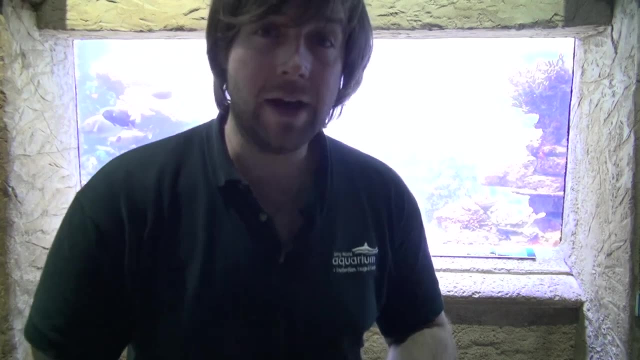 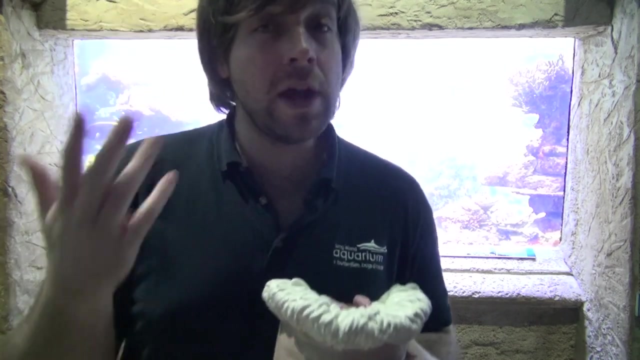 I don't really think of a polyp. I think of those branching Things that you see all over the ocean floor, right? So it turns out that those branching structures are colonies of polyps that are all genetically identical, So there's like thousands of them basically all living in a single branching structure that we know as coral. 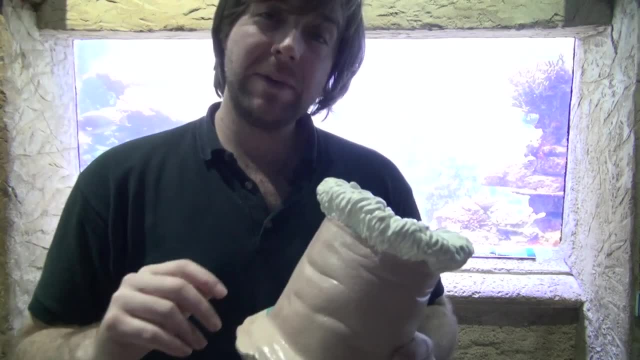 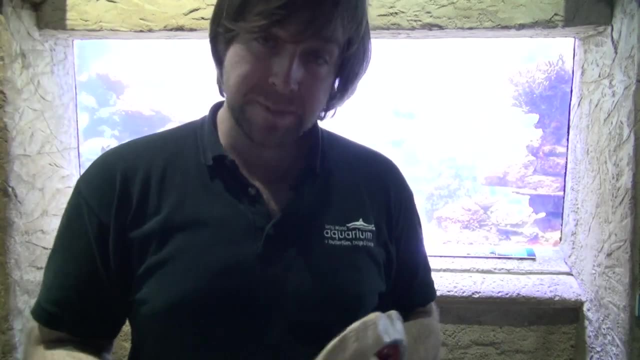 So this is the individual animal, And those branching structures that we see are colonies of polyps, of individual animals, individual corals, all living together. That's pretty crazy, right? So there are thousands of different species, There are thousands of species of coral out there. 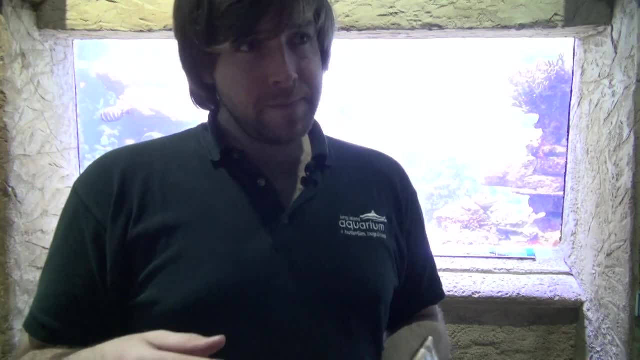 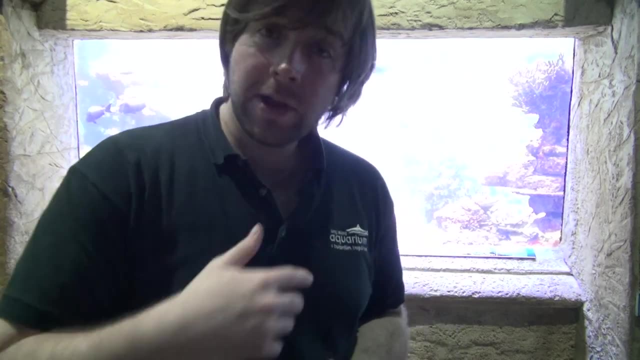 Their taxonomy is a little sketchy in some of the groups, But it's pretty easy to distinguish among a lot of the major different types of corals, And so we can take a look at our reef tank to really hammer out some of those differences. 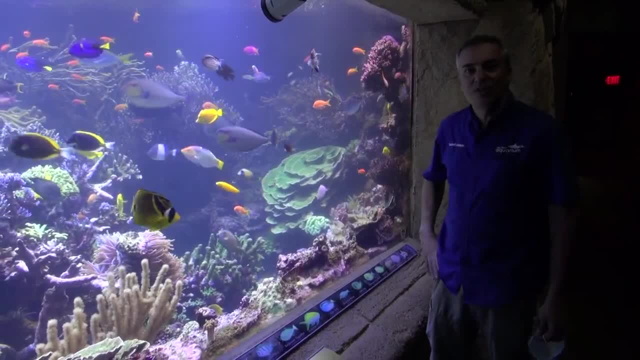 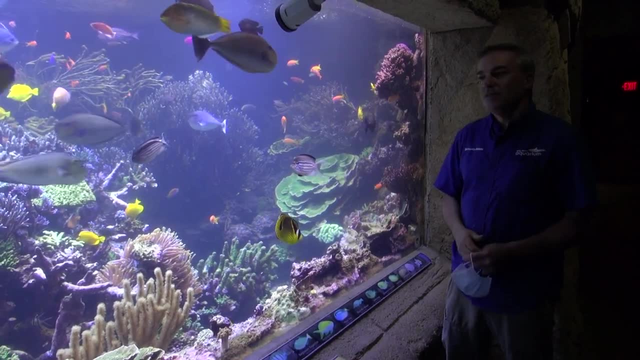 Let's take a look. So welcome. My name is Joe Waiula. I'm the curator and co-founder here of the Long Island Aquarium. Corals have been an obsession of mine for over 35 years now. There's some corals in this tank that are going to be 30 years old. 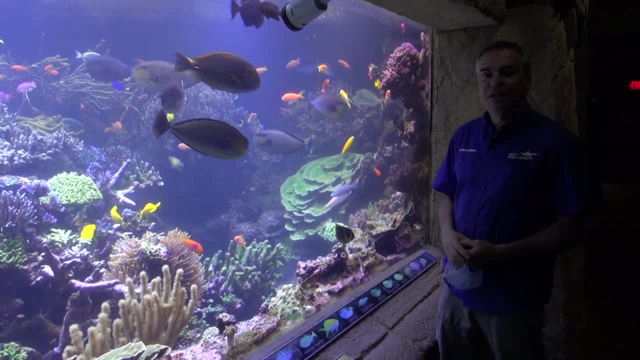 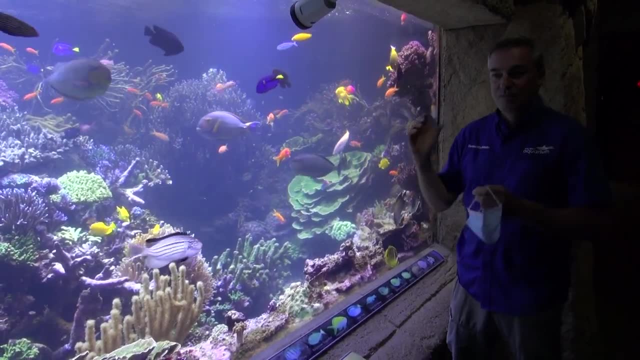 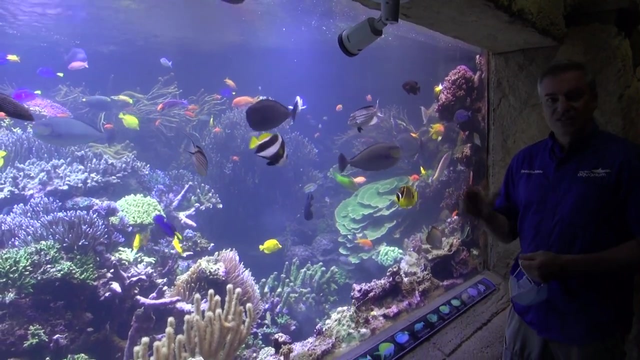 This year, Other ones date back 27 years, So there's a lot of history in this tank, And corals fascinated me. They captured and made me obsessive over them the minute I realized what they were and what they did, And I've never stopped obsessing over them. 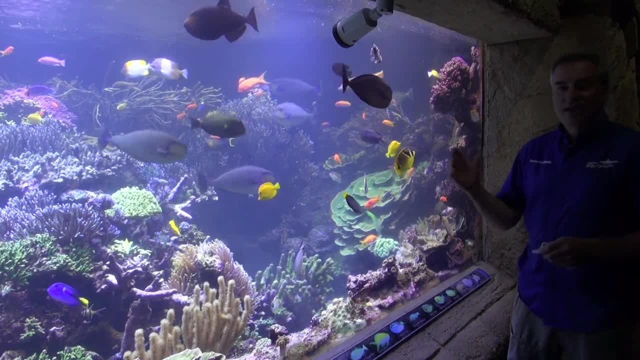 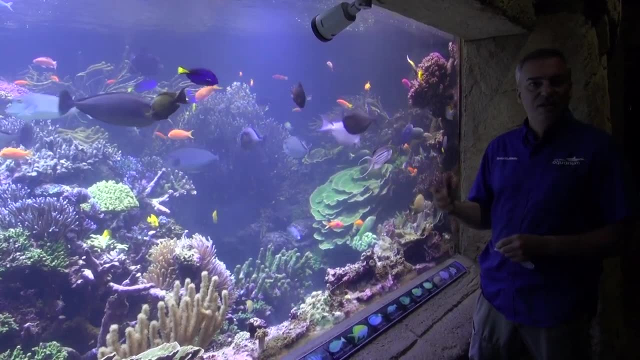 So when we first started trying to grow corals and maintain them in habitats, it was pretty difficult. It really wasn't too much well known on what was needed to take care of them Long term, So it's been quite a learning process through the years. 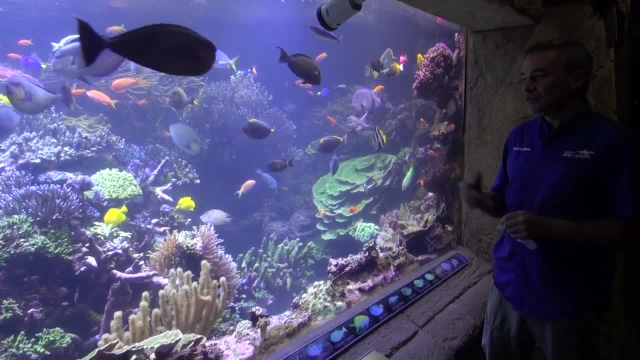 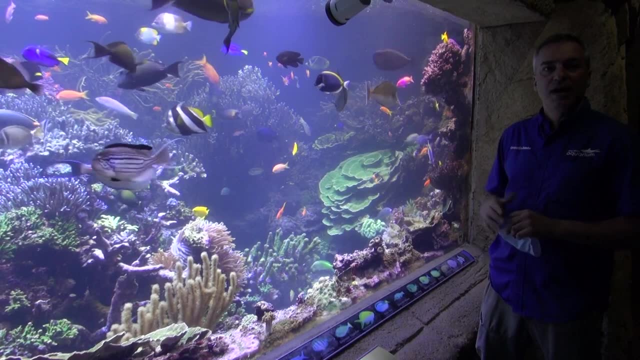 But corals are animals. There are soft corals, There are stony corals. Stony corals have a hard calcium carbonate skeleton. They're made up of thousands of polyps And we're going to get into that at different stages of the discussion today. 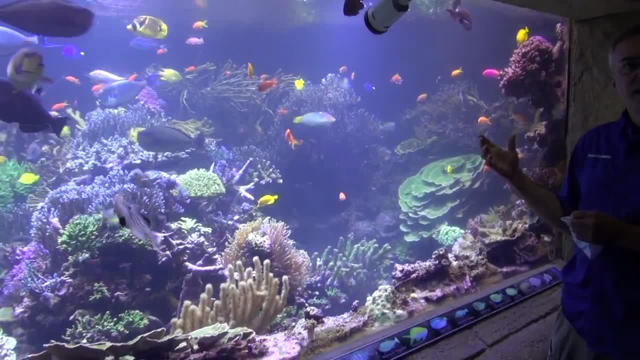 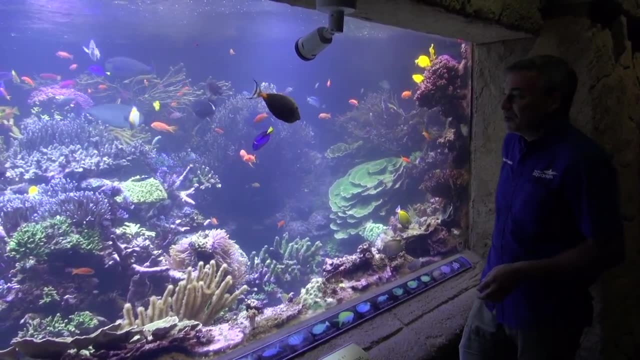 So, yeah, So within this tank, you know we're duplicating the sunlight. Corals are fascinating. They are animals, But they do have algae living in their tissue, Or reef building corals, Or hermotypic corals have algae in their tissue. 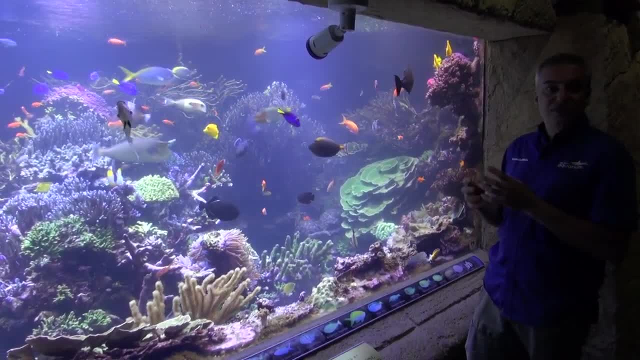 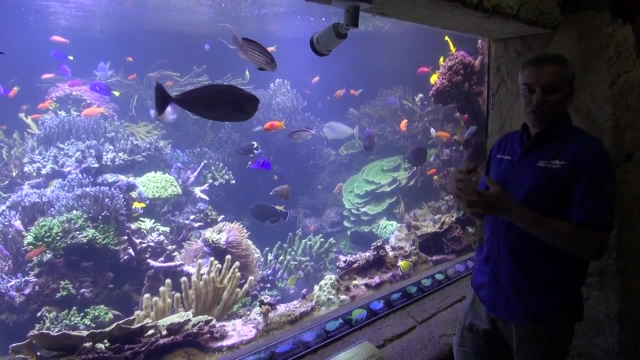 And that symbiotic relationship is pretty fascinating Because a coral can get upwards of 90% of its nutritional needs from that symbiotic algae that's growing in its tissue. So a coral is an animal. It's giving off nitrogenous wastes. 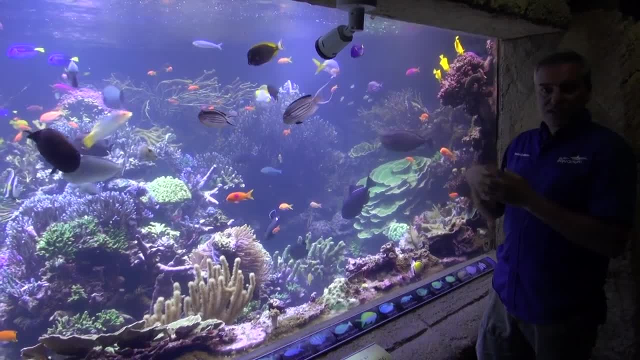 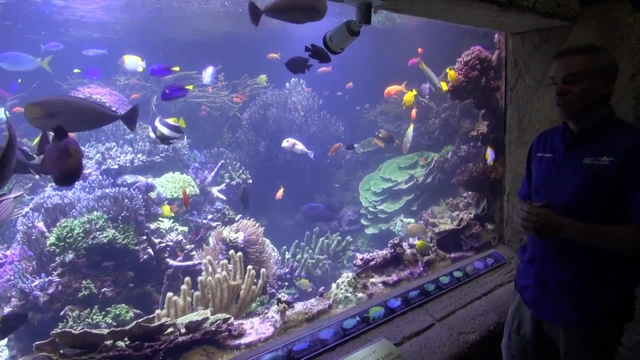 It's giving off carbon dioxide. The algae that's in the tissue takes that up directly, Just like a terrestrial plant will take up CO2 and nitrogenous wastes like fertilizers and things like that. The algae then photosynthesizes, Gives off oxygen which the coral can uptake directly. 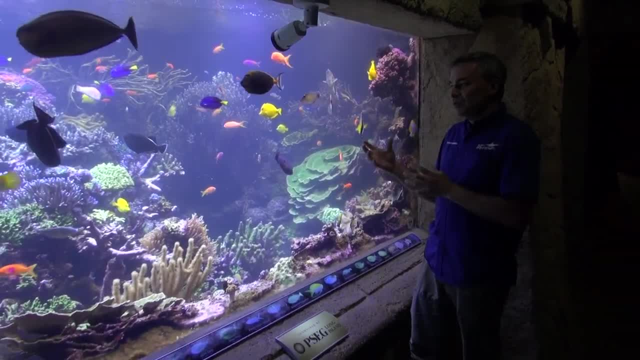 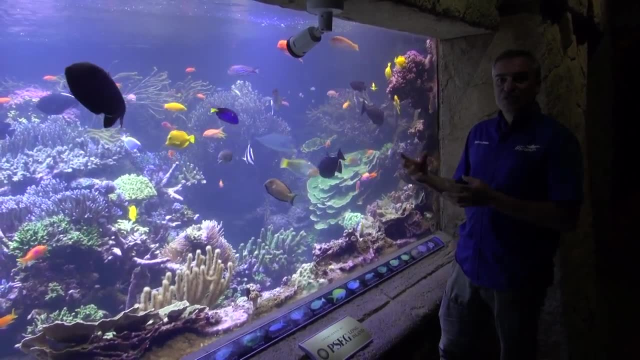 It also gives off sugars and starches and things, which is a food source for that coral. And now you're looking at the coral being able to maintain upwards of 90% of its nutritional needs just from the algae that lives in its tissue. 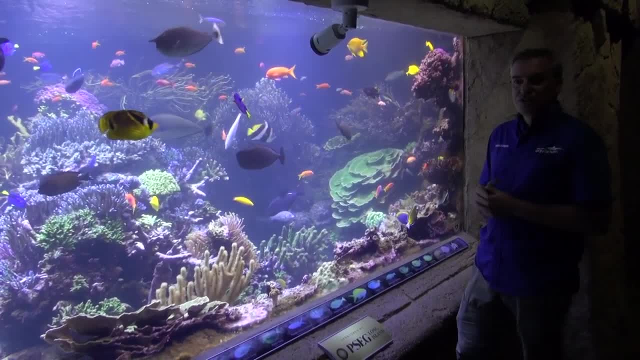 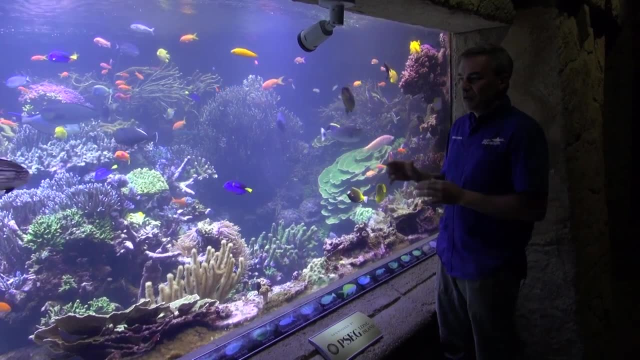 So not all corals have algae in their tissue. There's very few absolutes in the animal kingdom So you can't say all corals or none. But most reef building corals are going to have algae in their tissue And rely on that symbiotic relationship. 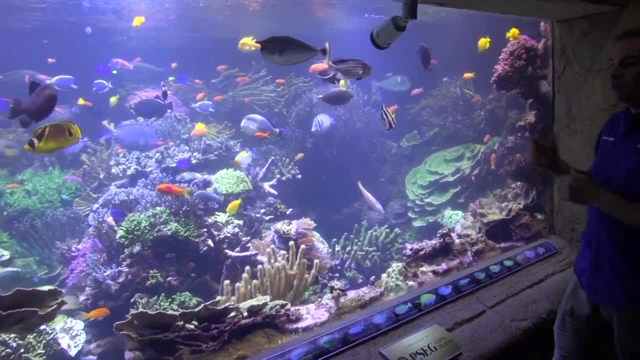 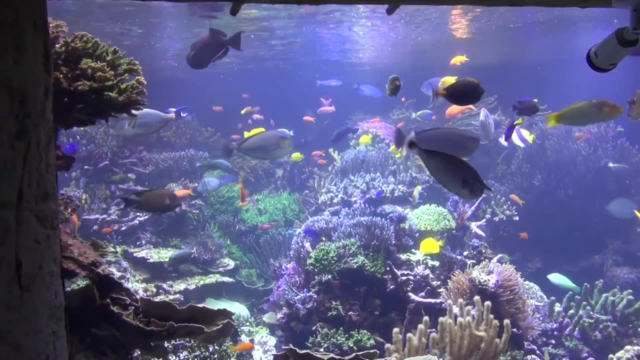 And that's why this tank is so brightly lit. with 26,000 watts of light, We're duplicating that sunlight. That sunlight is fueling that algae in the coral tissue And that algae in the coral tissue is fueling the coral itself. 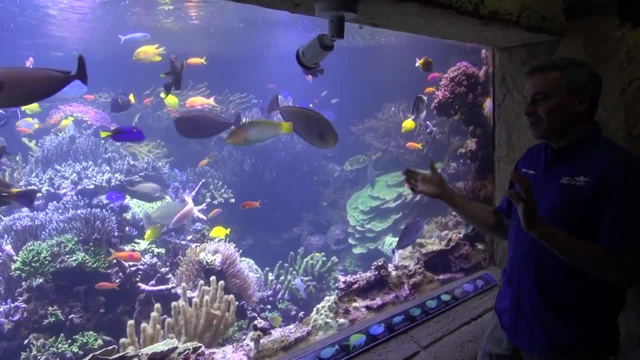 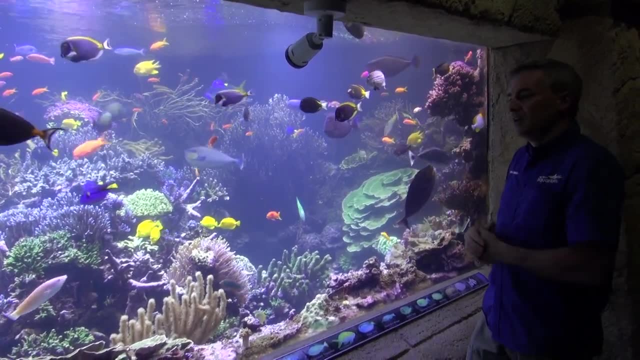 So most reef building corals you're going to find basically 30 degrees north and south of the equator. They need that really clear water for that light to penetrate, to grow the algae. But there are corals in basically every ocean at every depth. 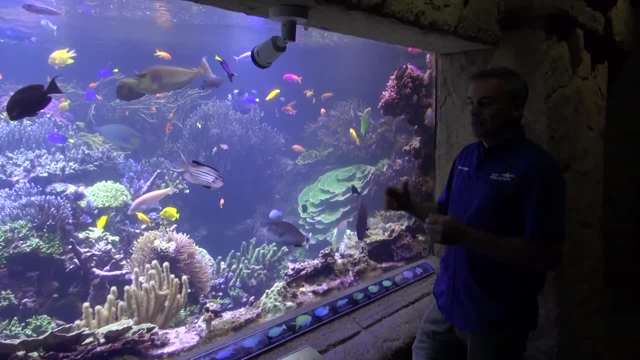 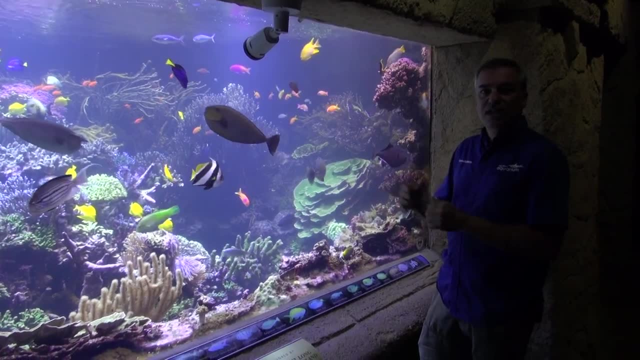 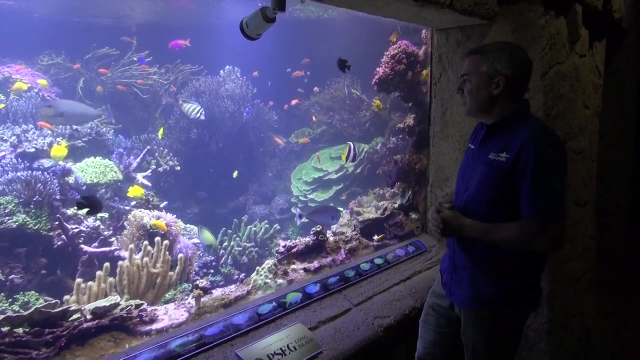 So they're quite diverse, quite adaptable. Their morphology, their shapes will change depending on the lighting and the water flow and the currents and things like that. So the same species of coral can look very different depending on its location. The tank here, like I said, has been up and running 20 years now. 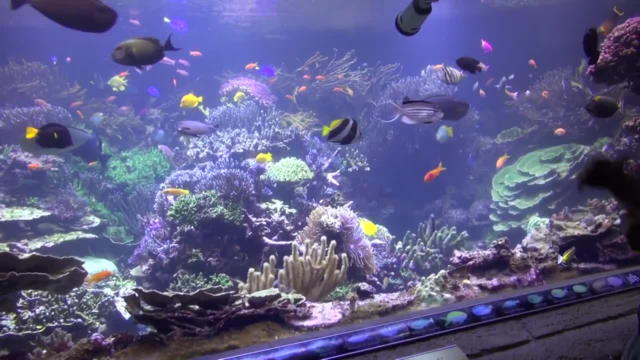 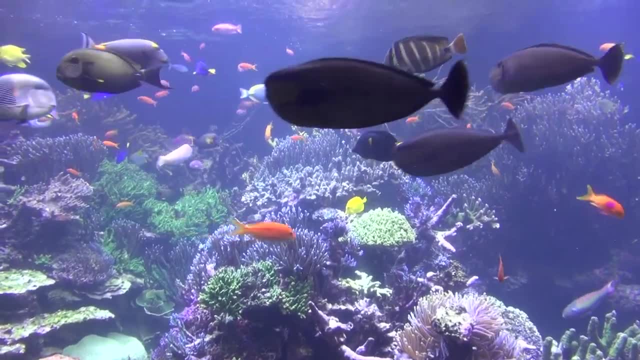 It's hard to believe If you're looking at the corals, especially like the Acroporas, those branching corals, those blue tips and those white tips. that's the growth region of the coral. That axial polyp is the growth polyp. That polyp grows straight out. And as that polyp grows straight out, the radial polyps grow in around it And then those branches split. And as they split then they keep growing, So they can grow pretty quickly. There's a lot of misnomers about corals: are slow growing. Some are, some aren't. Those Acroporas, if the conditions are really good, can grow a millimeter every other day, And then when they start branching and splitting, then they're going to grow a millimeter every other day, cubically. 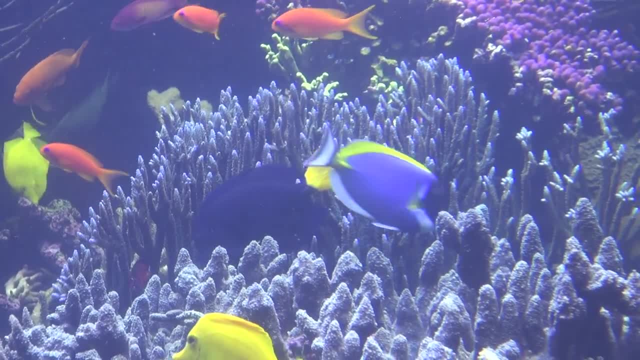 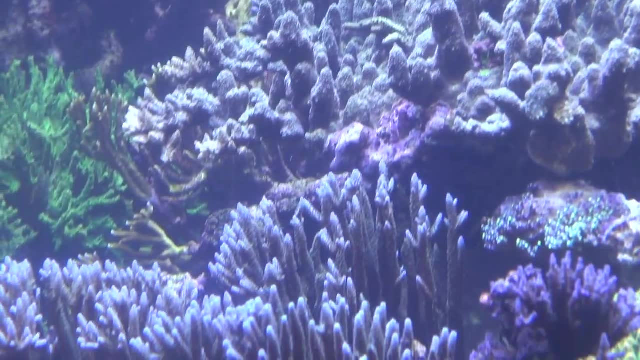 So their volume can increase tremendously, But they tend to be a little more fragile, So if a bigger storm comes through they will get broken and fragmented, versus something like a brain, coral or something that's a little more solid can withstand those storms. 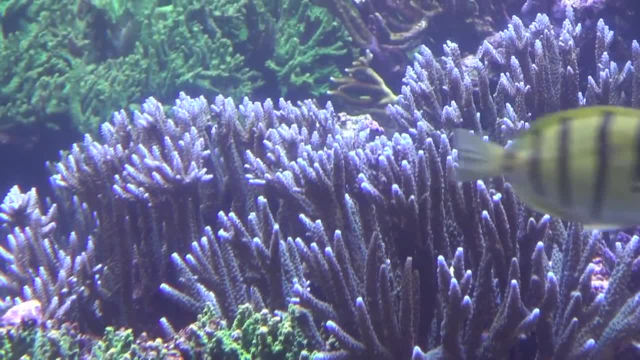 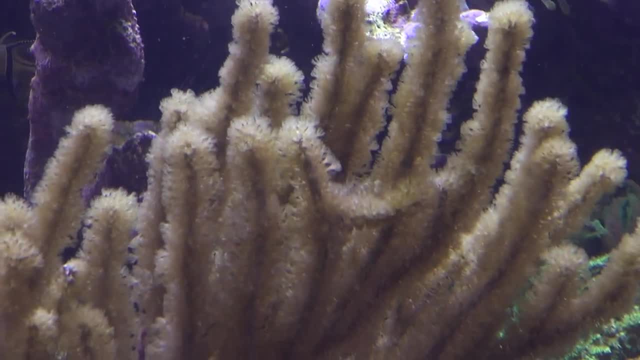 But those might be slower growing. A lot of the soft corals don't have that rigid cavity. They have a calcium carbonate skeleton, The Gorgonia down here. you can see it waving in the current. It has a soft, flexible skeleton. 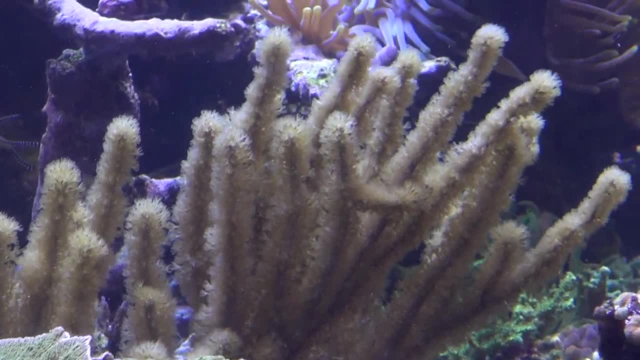 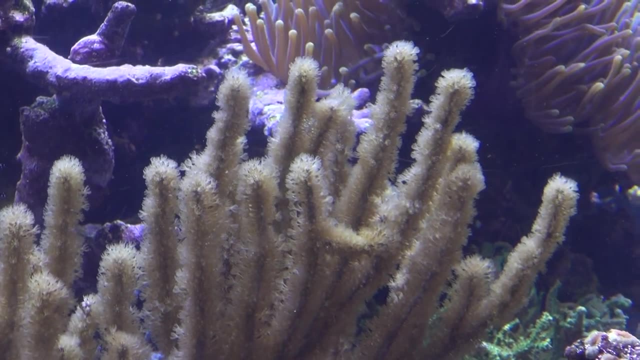 And that's going to go to and fro with the waves. It can withstand maybe those stronger storm surges and things like that. A lot of soft corals, a lot of the Gorgonia, are filter feeders. They don't have algae in their tissue. 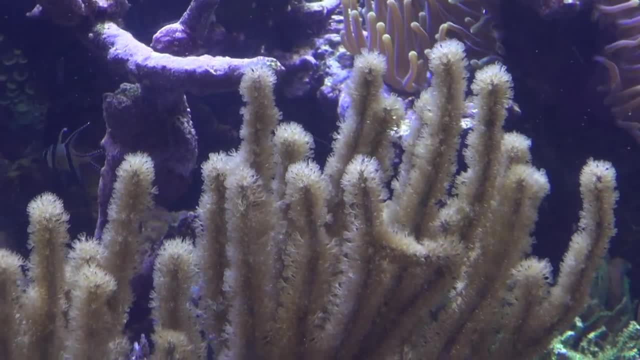 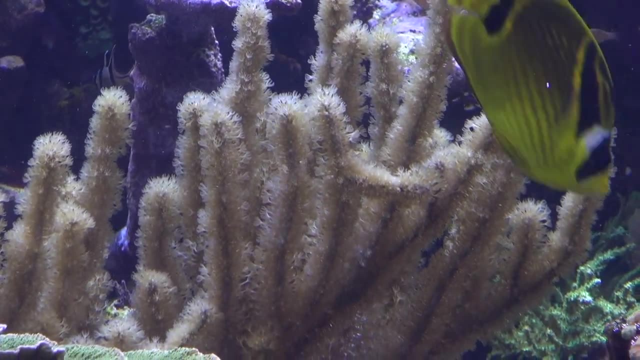 and are going to be feeding off of plankton and things in the water. The Gorgonia here is an Atlantic soft coral that will do both. Those polyps are great at capturing food, but they also have algae in their tissue and are photosynthetic as well. 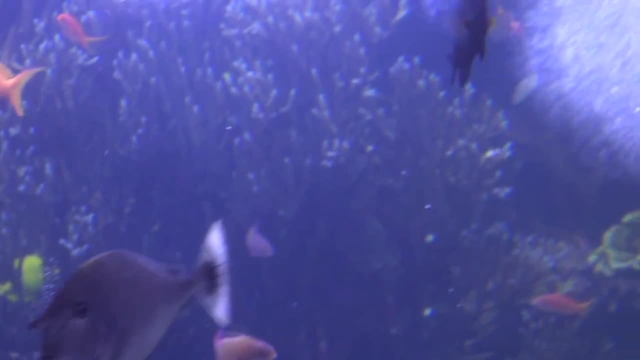 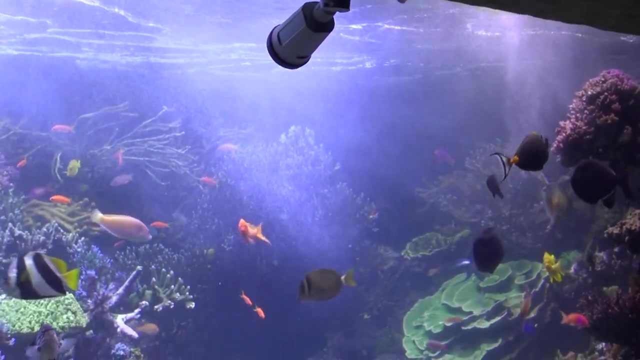 And there is a surge mechanism on the tank right now, So water flow is really critical. So this is dumping about 300 gallons of water in about 35 seconds And that creates a really nice surge of water. Corals are sessile invertebrates. 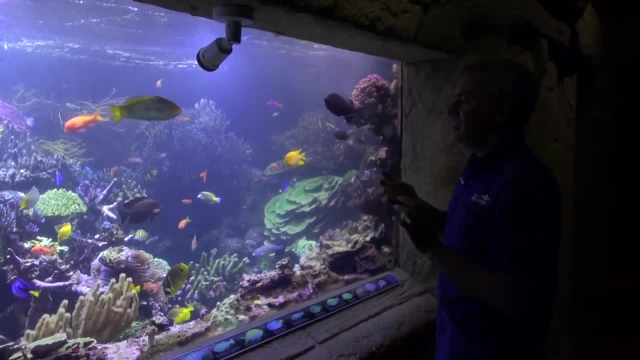 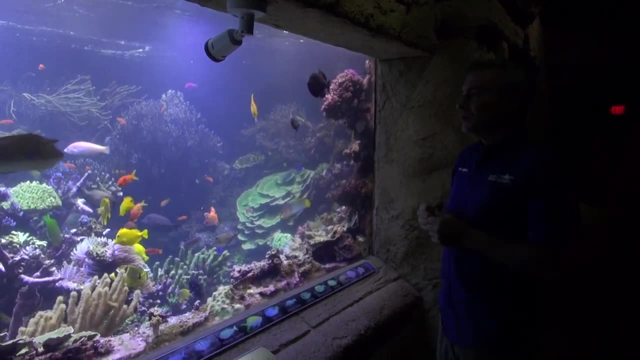 They need nutrients brought to them and they need the, the wastes removed from them. So they're going to be in- a lot of them are going to be in a high energy zone, So we're duplicating that here in this habitat. 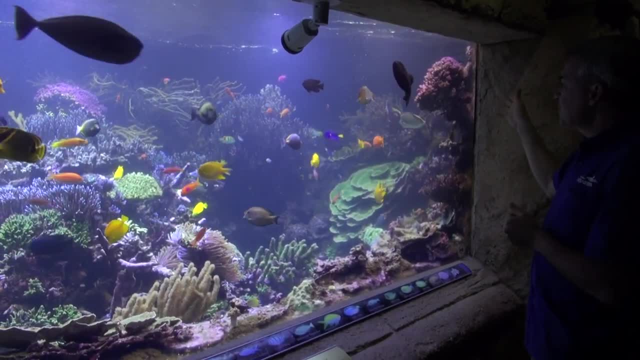 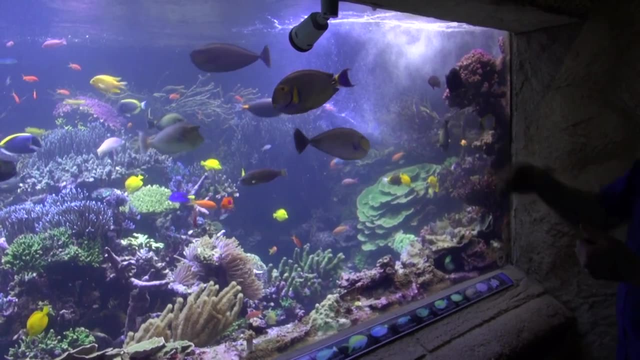 with that surge device. It's called a Carlson surge device. It's going to stop shortly. It's going to refill back up in about eight minutes It'll do it again. So that's a lot of energy: 300 gallons in 35 seconds. 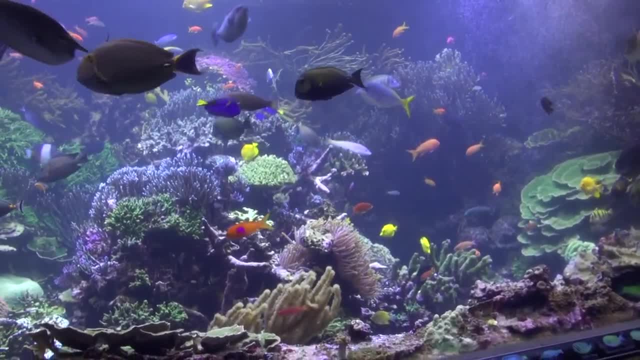 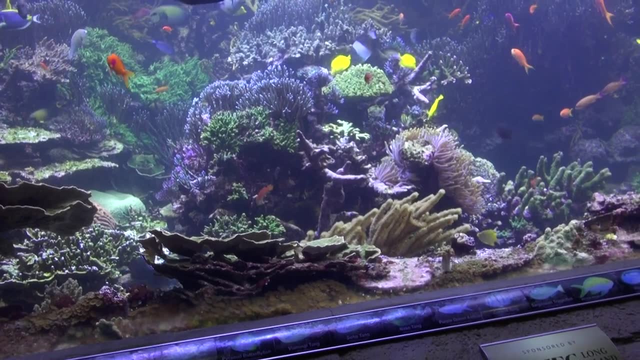 There's lots of other random water flow on the tank to keep the corals moving, A lot more than you would have on a standard, say, fish only tank, Because, again, these corals need need lots of water flow, especially as they grow and they get bigger. 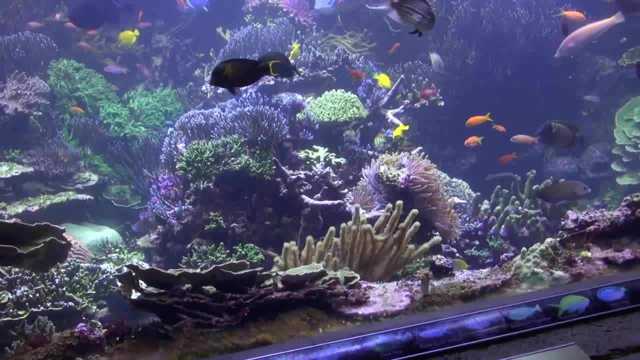 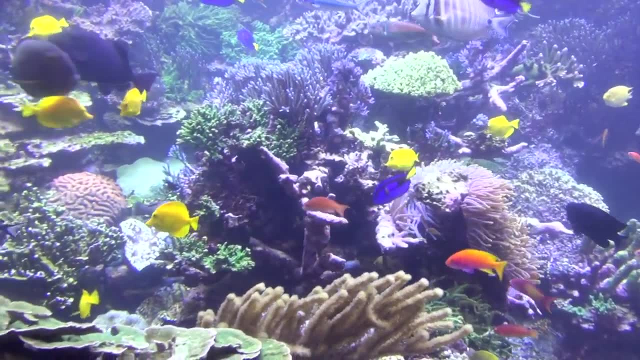 They're going to block the water flow, So then you have to increase the water flow. This habitat is home to hundreds of different corals and fish from around the world. Now, we're not going to be talking about the fish, for the most part, today. 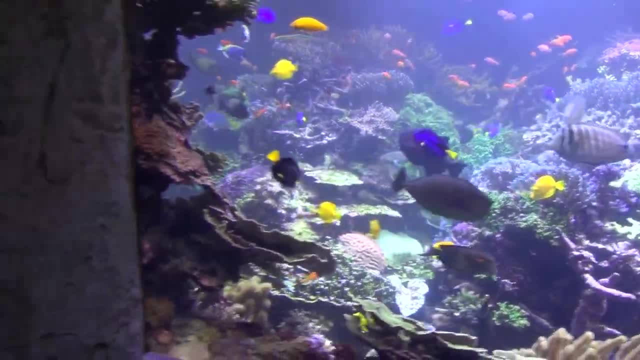 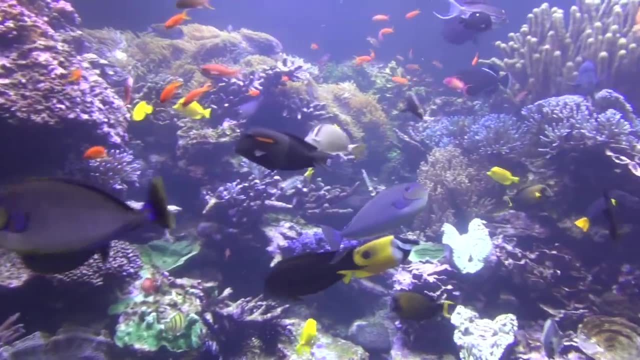 just because we are focusing on invertebrates, But I want you to notice that, as you take a look at this habitat, what you should see is that the corals, which are all laid out at multiple different heights, almost look like flowers. 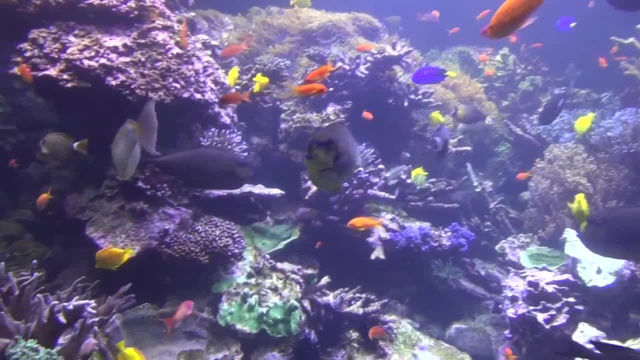 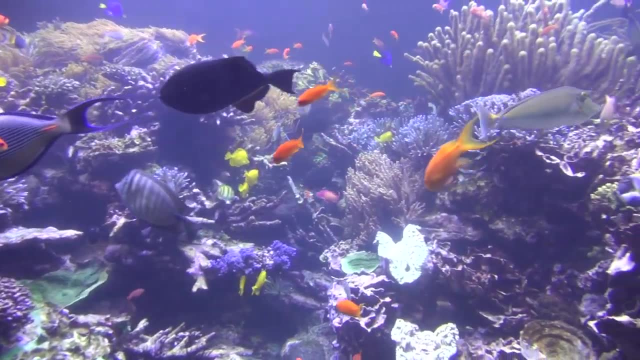 It kind of reminds me of looking at an underwater garden, And so that's actually where corals get their official scientific names. So within the Cnidaria, corals belong to the class Anthozoa, which basically means flower animal. 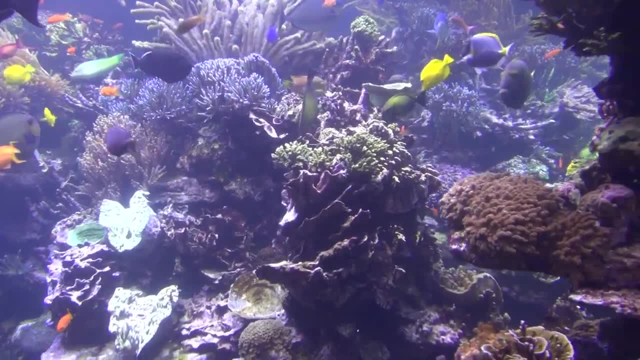 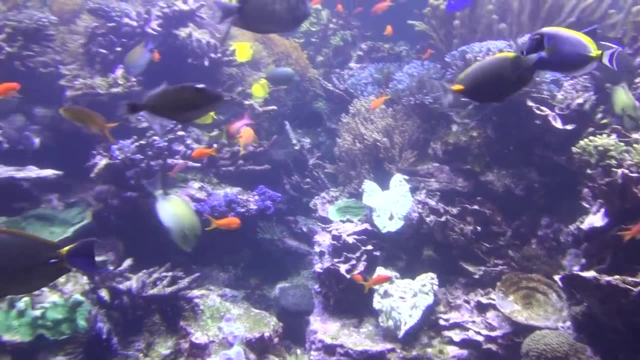 So again, even though they superficially resemble plants, they're not plants. But in Greek, antho means flower and zoa means animal. So that's what they look like. That's where they're getting their classification from. Now the Anthozoa is broken into two major groups. 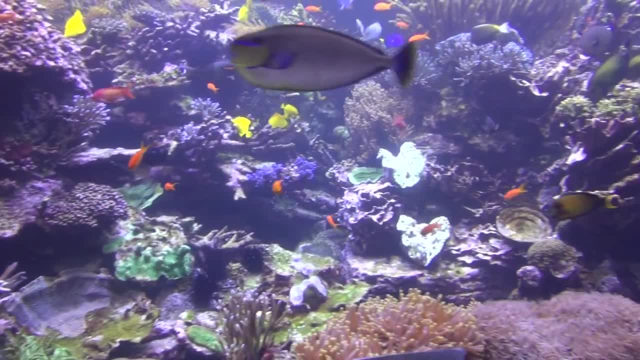 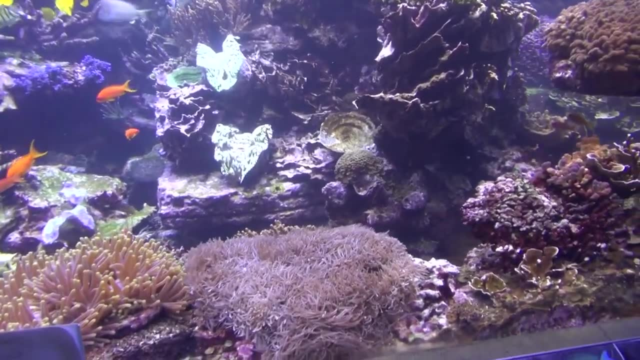 the so-called hexachorallia and the octochorallia. Now they are distinguished by their type of symmetry. So, for example, if we take a look at this soft coral right here, So soft corals all belong to a single order. 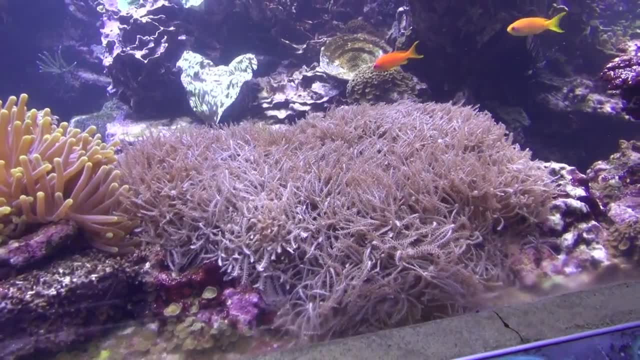 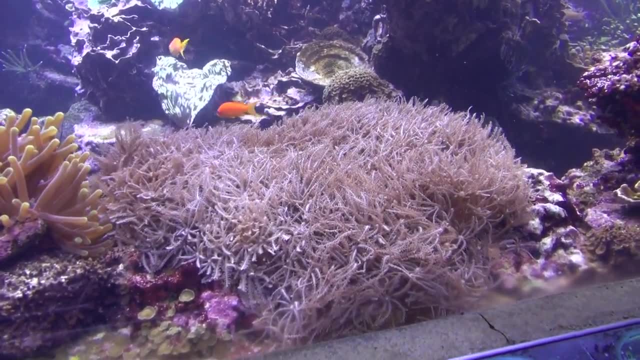 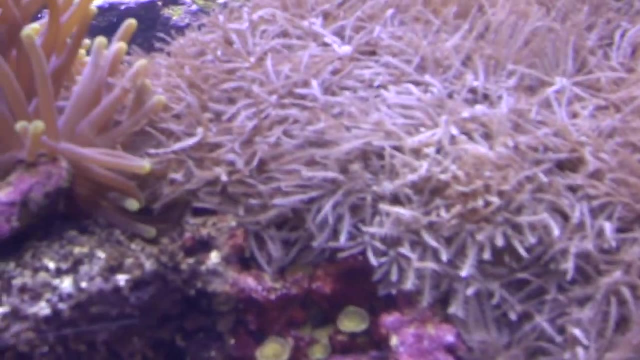 within the octochorallia known as the Alcyanacea. Now, what makes them be placed into the octochorallia is their type of symmetry. So if we take a look at a single animal in this colony, so basically one singular polyp. 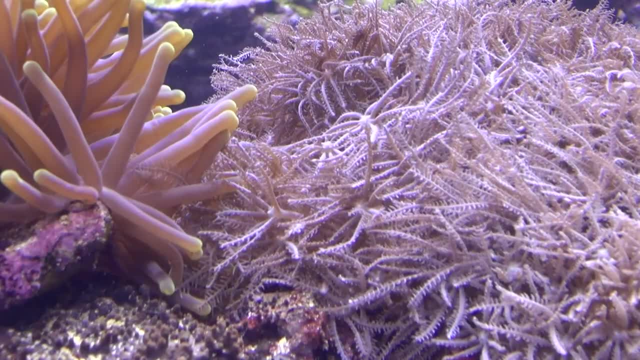 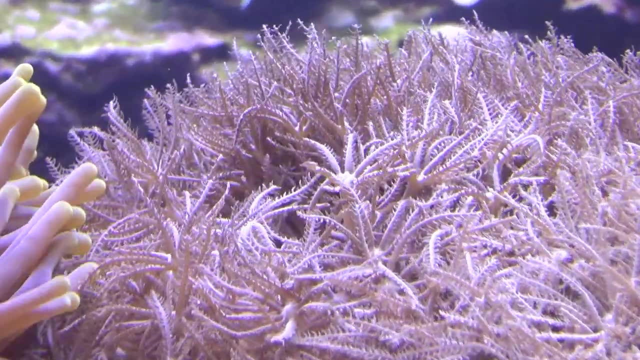 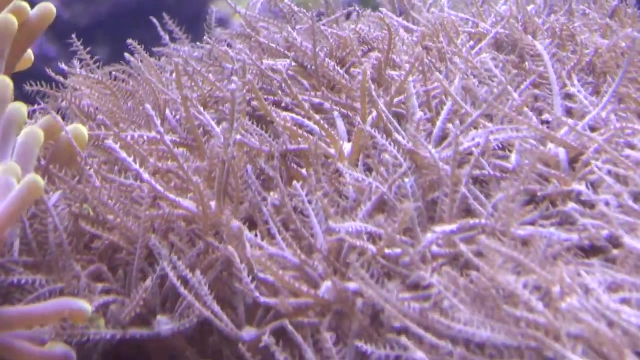 Let's see if we can find one here. So there we go. There's one sort of blowing around up there in the current. So what you should notice is that each one of these polyps, first of all the little white dot, that's all the way in the middle. 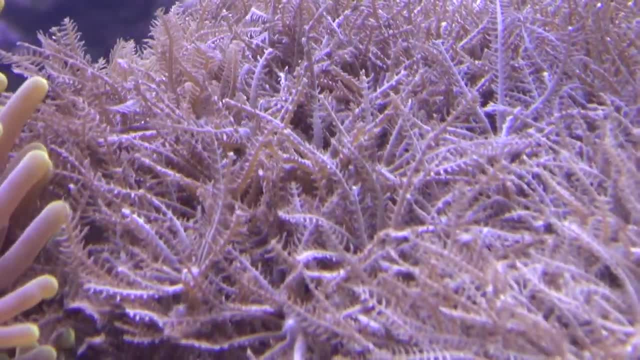 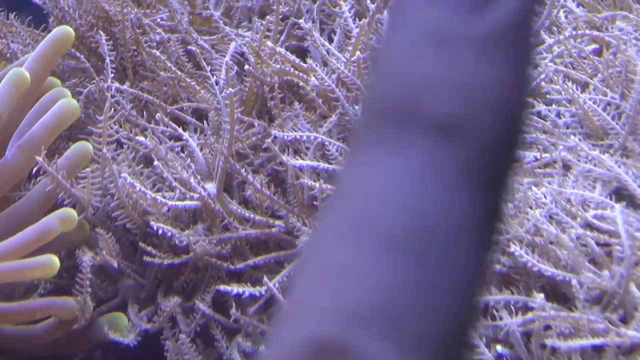 of all the tentacles is the mouth. So, for instance, right there- let me point it out to you guys, there we go, right there, that little white dot that's in the middle of that polyp, that's the mouth. 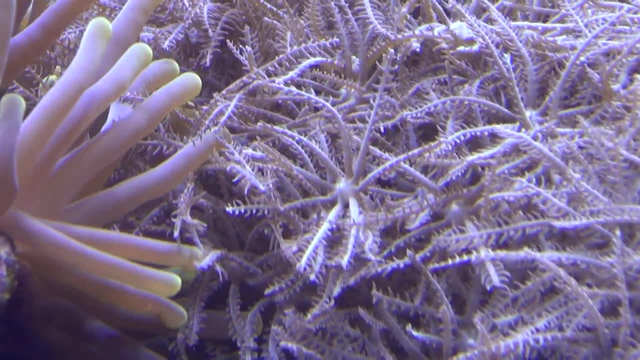 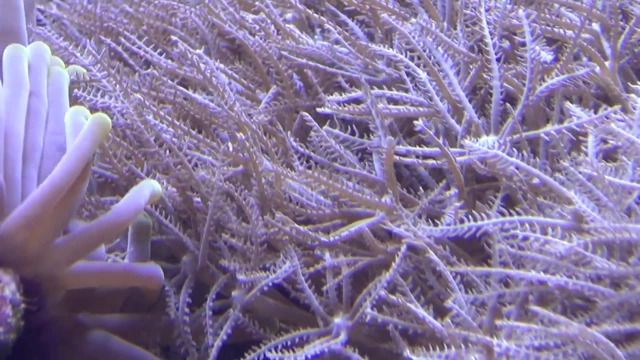 And if you look at a polyp from the top, notice that it has one, two, three, four, five, six, seven, eight tentacles, And so we call this eight tentacles, we call this eight-fold symmetry. 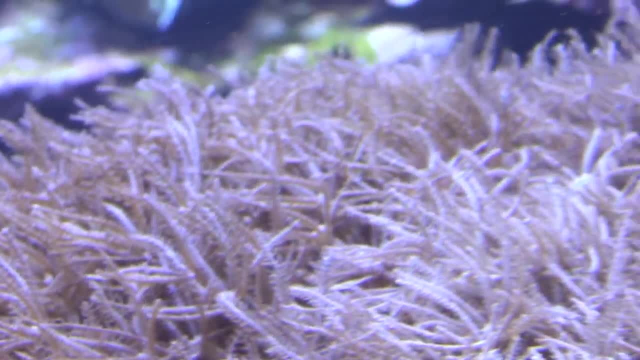 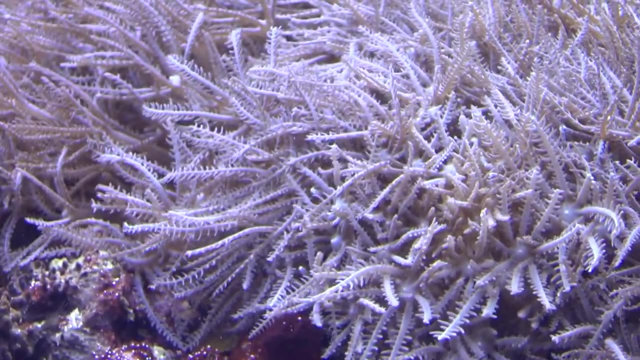 So if we looked at it face down, we could divide it radially up into eight pieces, So kind of like a pizza with eight slices. That's what makes this an octochorallium, So all of those soft corals belong to octochorallia. 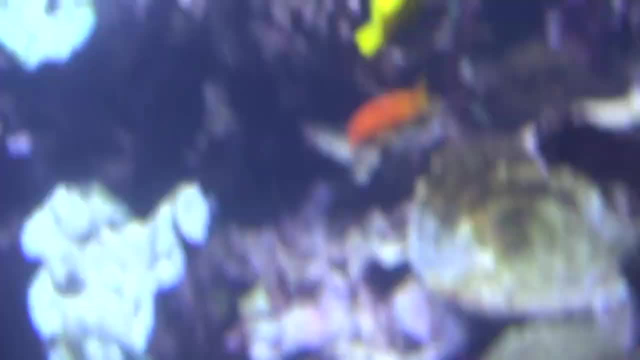 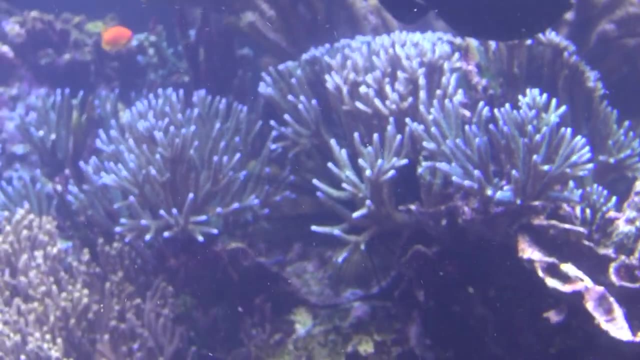 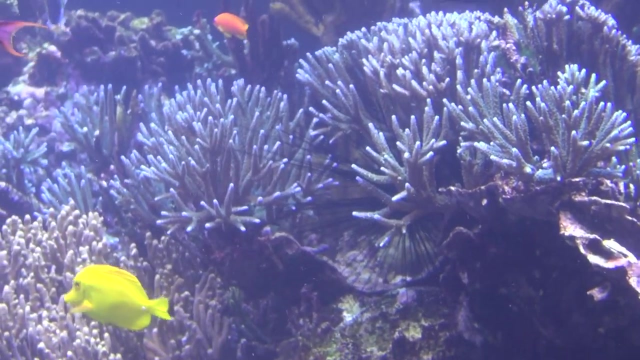 The hexachorallia includes the stony corals, And stony corals literally have a hard calcium carbonate skeleton. So, for instance, we can take a look at these acropora or acros right up here. Those guys are a little bit more rigid. 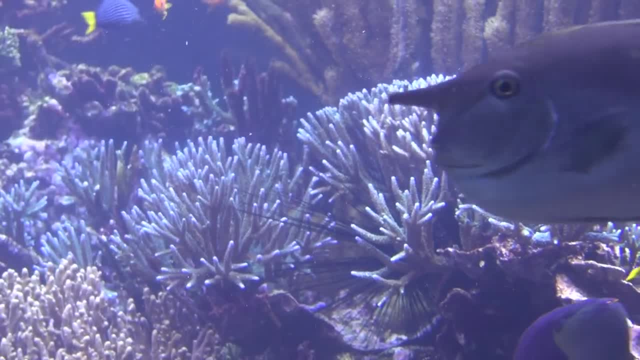 Their polyps are actually retracted at the moment, but they're a little more rigid. So because of that calcium carbonate skeleton we call those stony or hard corals Now the octochorallians, the soft corals. 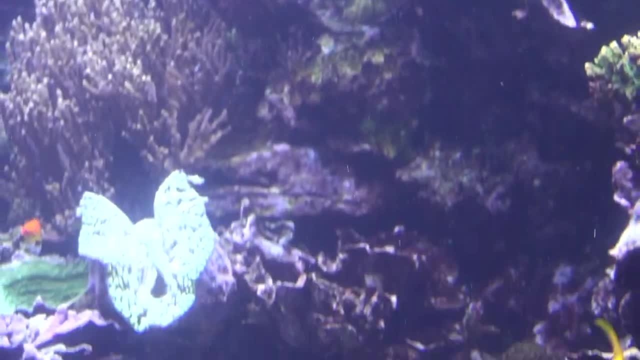 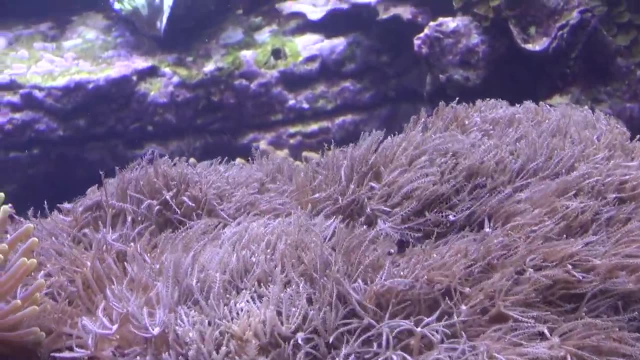 they still do produce, almost some of them do produce a skeleton, but they have little pieces called sclerites, little calcified pieces called sclerites which give them support and structure. They're not quite as intricate as a stony coral. 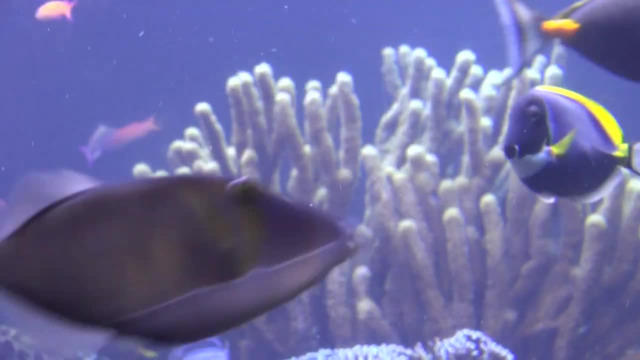 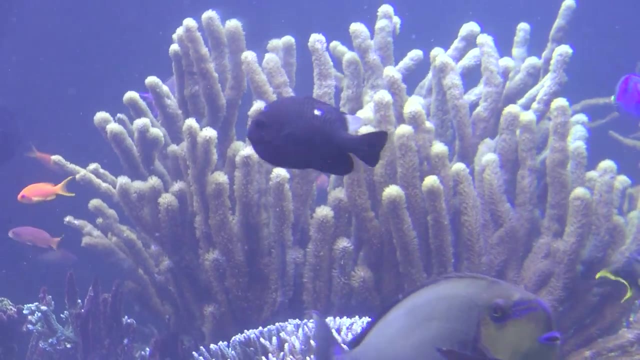 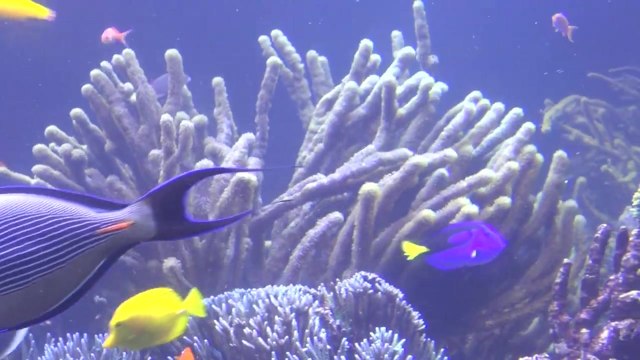 Some of the soft corals, like this gorgonia up here, contain a flexible protein known as gorgonin, which makes their skeleton a little bit more swishy, giving them the name sea whip, because they tend to drift in the current. 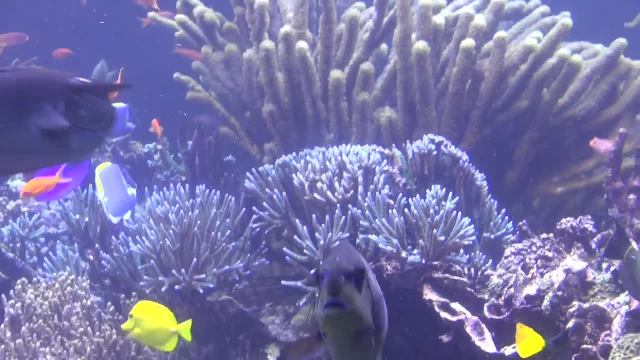 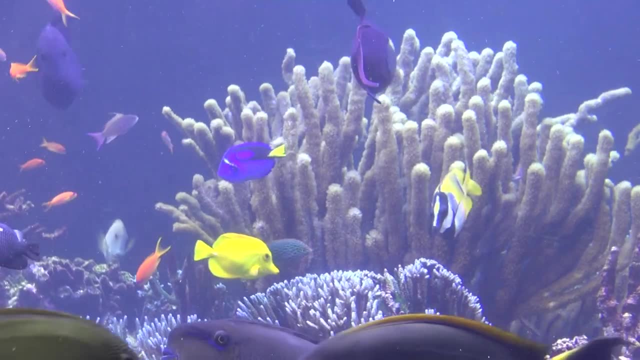 But let's go to our curator, Joe Waiulo, for him to tell us a little bit more about the differences between stony corals, because there are a lot of those out there and there are some pretty distinct differences that people in aquariums, professionals in aquariums- 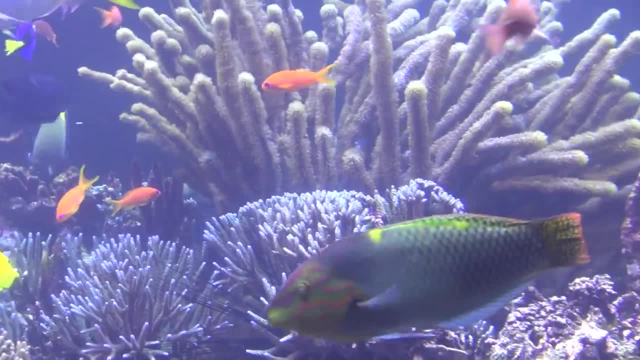 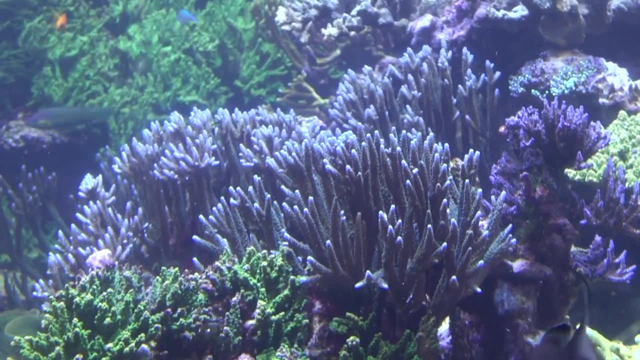 as well as in the hobbyist trade, tend to use to distinguish them. So let's take a look. So corals are made up of polyps, thousands of polyps in general. So there's SPS. we call some small polyp stony corals. 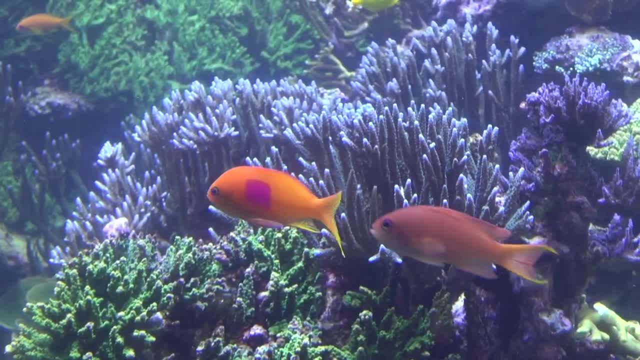 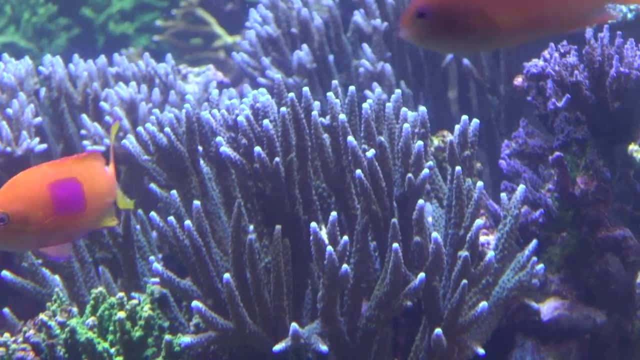 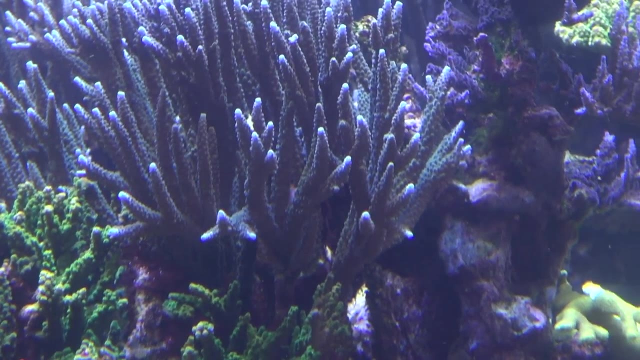 like the Acropora here. Each little bump that you see on there is an individual animal and then they're cloning themselves. So that's a colony of thousands of animals, just that one colony, And the polyps are tiny, but the polyps can get quite large. Right now a lot of those polyps are retracted. They can pull within their skeleton for protection, Often stony corals. the polyps will be drawn in during the day. That's not to say all. Again, we have to stay away from absolutes. 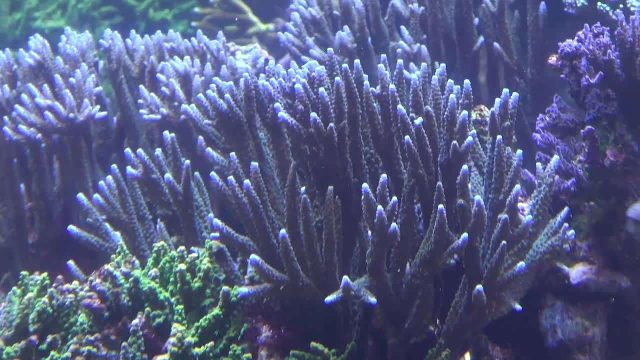 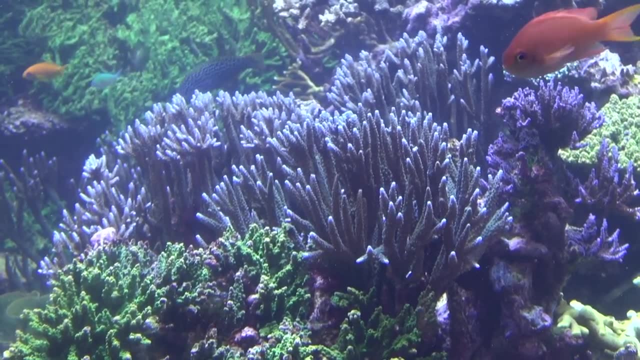 But for the most part a lot of the polyps are closed during the day and will come out at night to feed when there's more food available and less predation from different fishes and things. So right now those polyps are retracted. 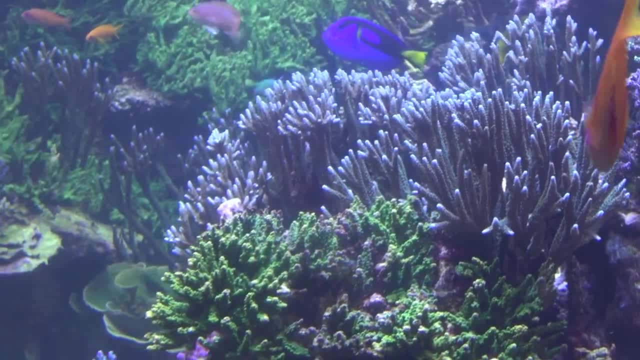 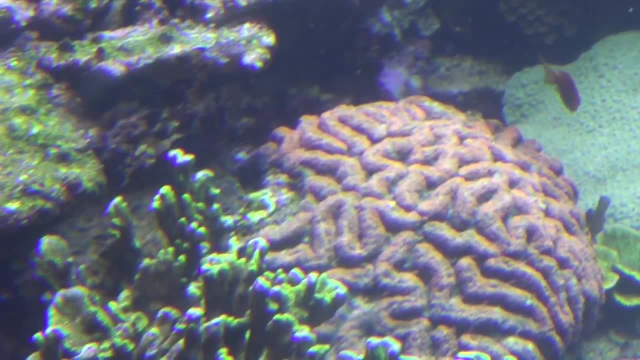 within the skeleton, within the polyp. Then you have large polyp stony corals or LPS, like this Symphylia. It looks like a brain, so we pretty simply call them brain coral. That's a colony of large polyps. 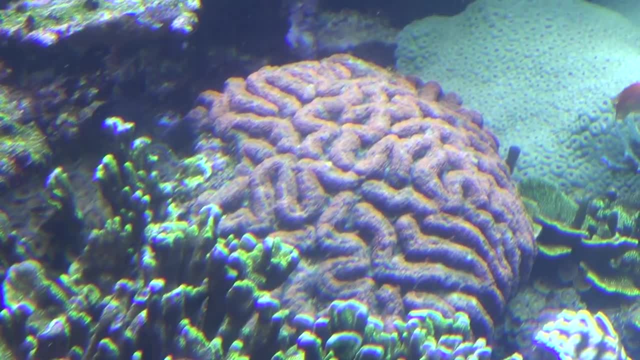 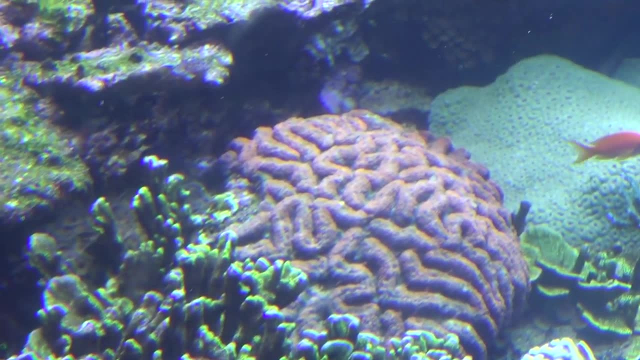 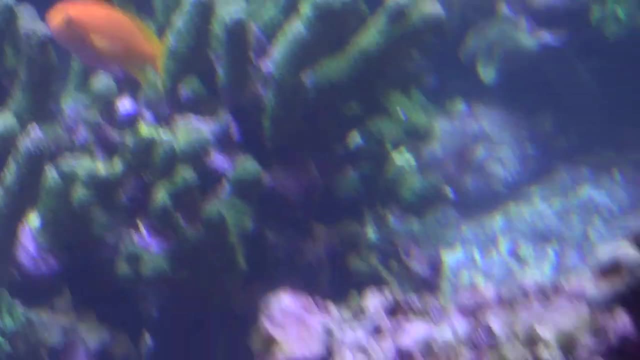 growing in a colony, So polyps can really range from barely a millimeter or even less across, Something like that. Symphylia has large polyps, And then there's other species called lobophilia. Come in on that one circle there. 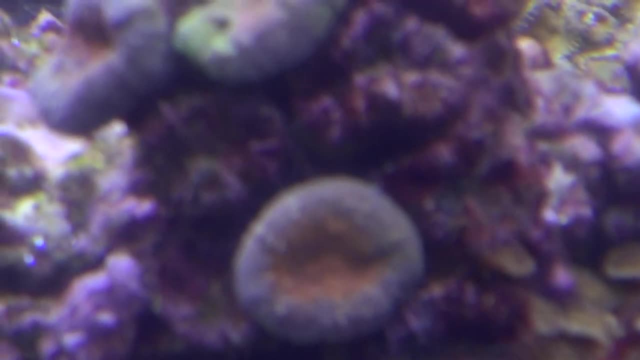 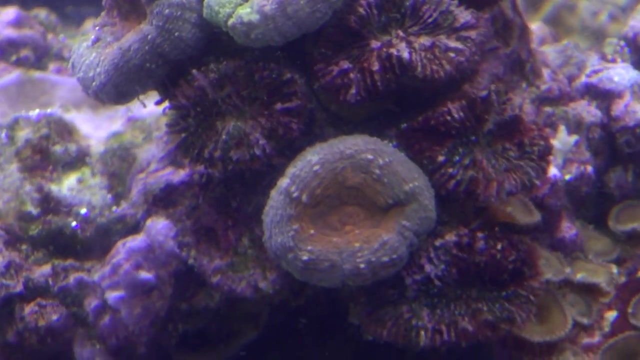 So that one, some of the other polyps have died off. So then they have individual large polyps like the lobophilia here, That is, a single polyp, And then other free-living corals. some of these other polyps can easily get to be. 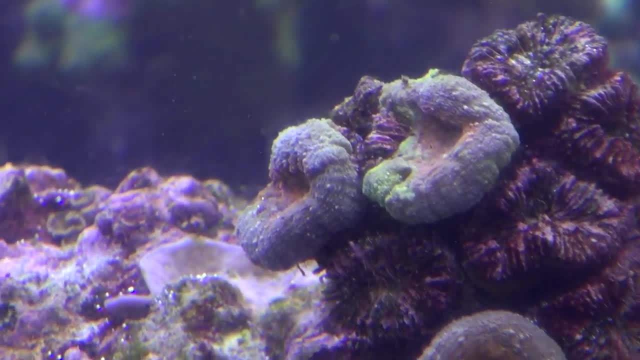 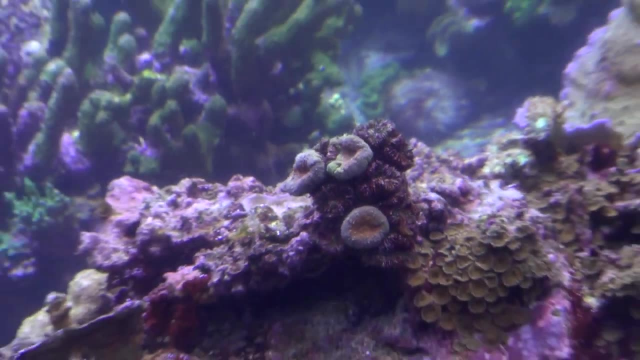 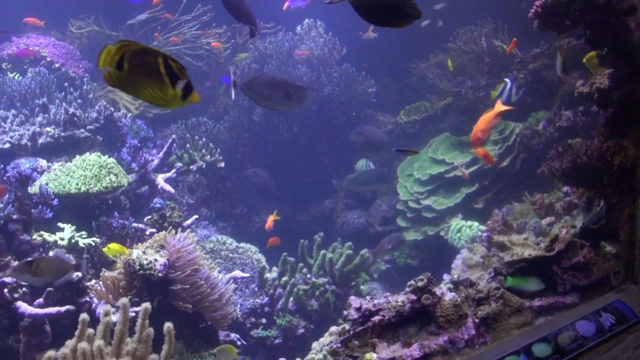 five, six inches in diameter, with it being one polyp, one individual animal. So, again, it varies a great deal And when these guys, especially at night, will open up and they'll have a lot of tentacles surrounding that mouth and grabbing a lot of food. 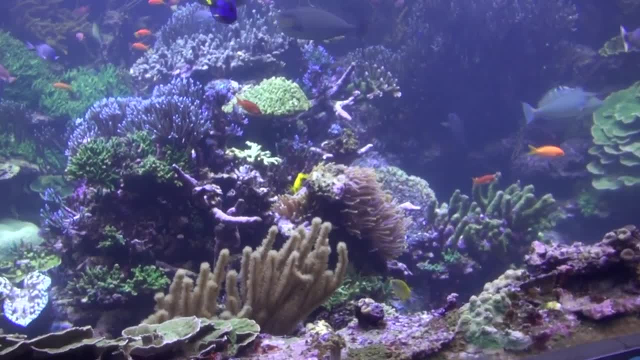 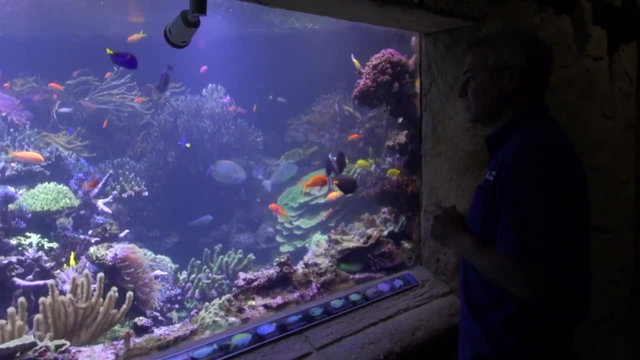 during the evening hours, But they also have the algae in their tissue, so their algae is photosynthetic. So they're photosynthesizing during the day and the coral is getting a lot of nutrition from that as well. Now just to clarify the points that polyps 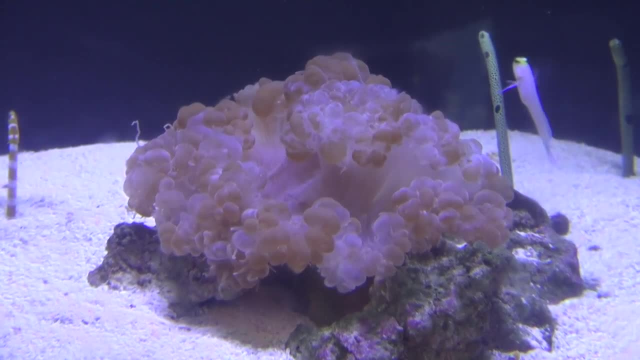 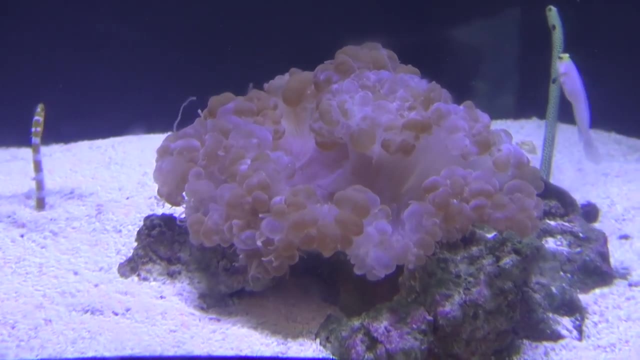 are not always small. This is an example of a large polyp, stony coral. This is known as a bubble coral And it's pretty cool. You can actually see the polyps are extended right now and they have these beautiful sack-like bubbles. 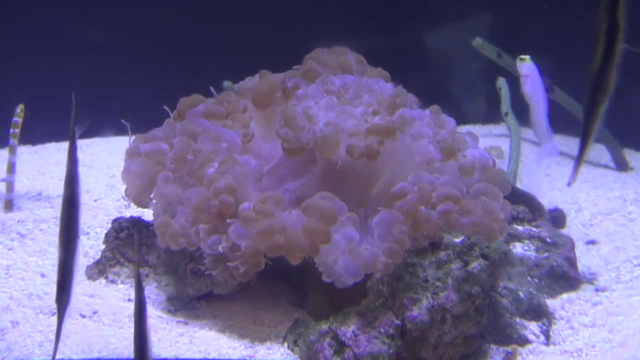 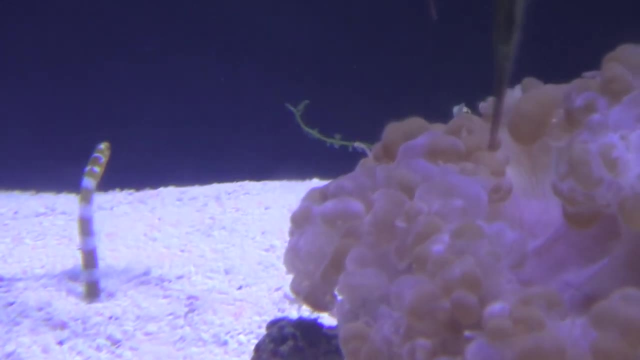 coming off of them, from which we can see tentacles sort of flailing around, And you can see those right there. These guys are reaching out for food. So this is our form and function tank, by the way. So you'll notice the little garden eels poking up. 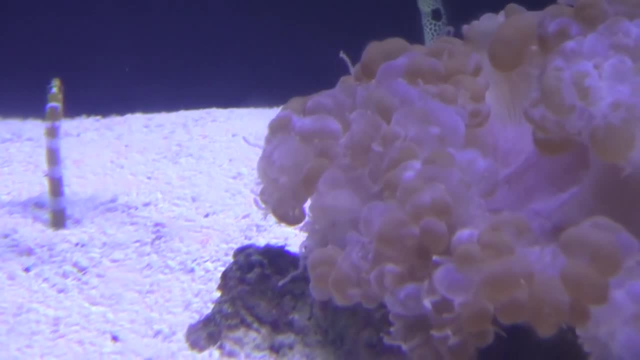 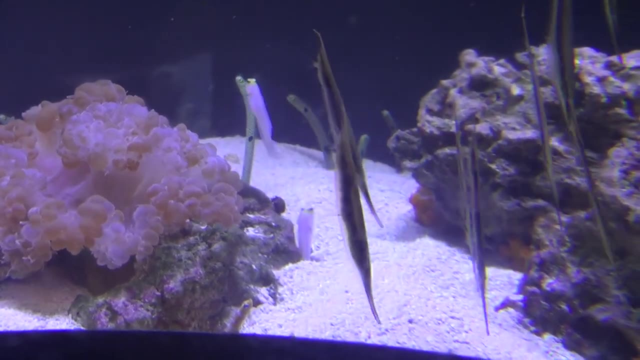 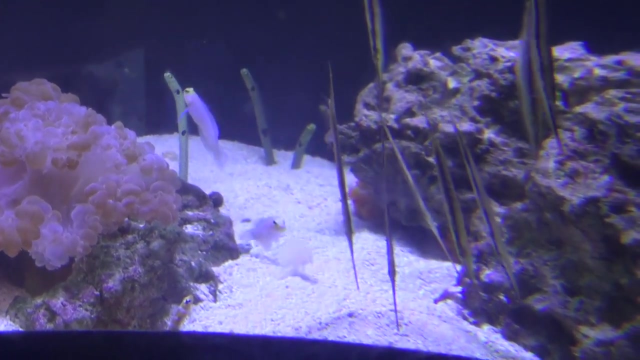 in the back there. We also have the shrimp fish up here in the forefront. These guys are adapted to living with corals as well, And specifically they're meant to resemble the spines and the branches of a staghorn coral In Southeast Asia, from which they hail. 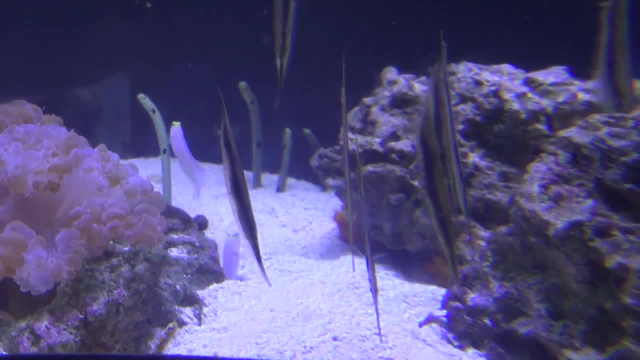 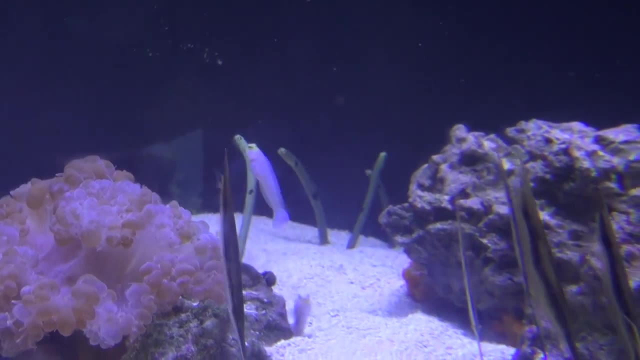 And these guys would blend in with those diadema corals and essentially camouflage themselves against the reef. But there's another coral in here as well, And this is one of the last groups that we really didn't touch on, or neither myself or Joe touched on. 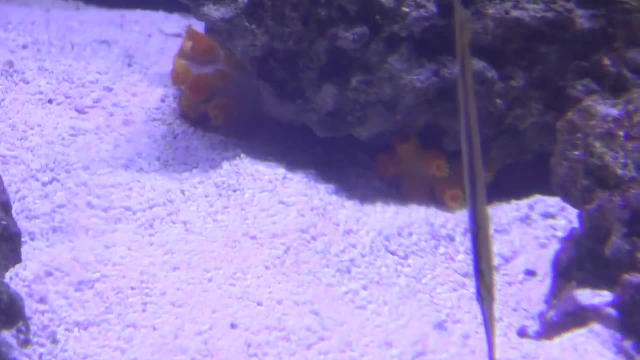 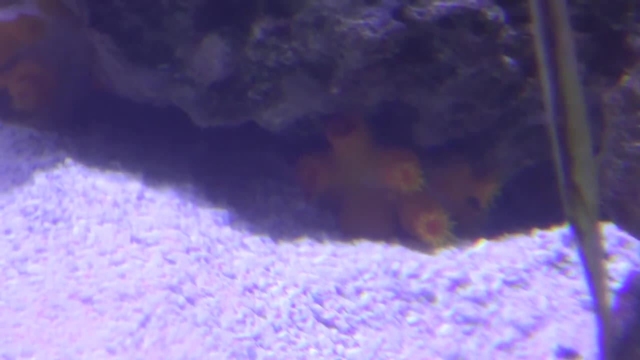 And the orange polyps that you see underneath over here. Excuse me, Mr Shrimp Fish- He's in the way- But those little orange polyps are known as sun corals And specifically these are the last major group of stony corals. 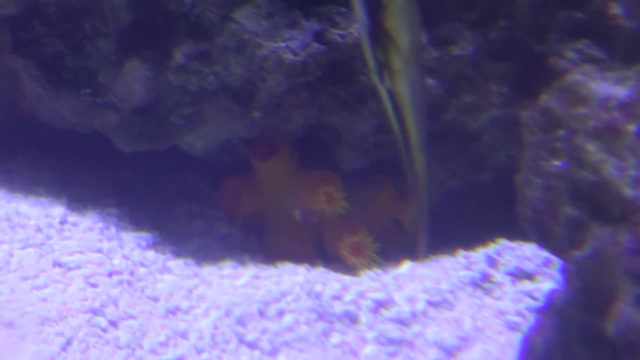 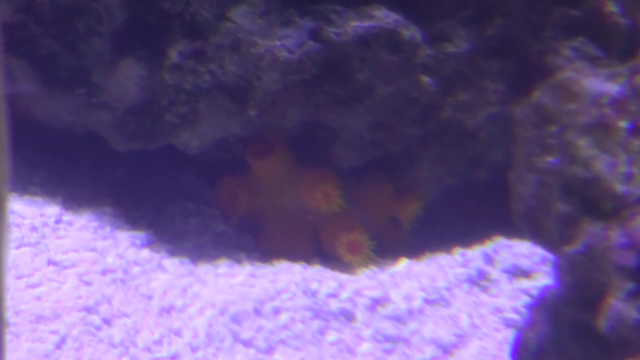 that we really didn't touch on too much. These are referred to as NPS in the hobby for non-photosynthetic corals. So these guys, while they are stony corals, they tend to occur at lower depths And they're not really as photosynthetic. 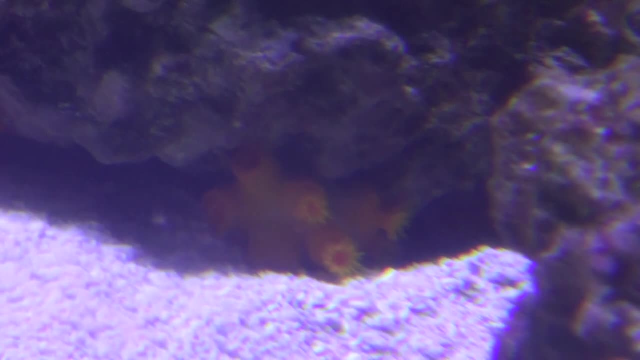 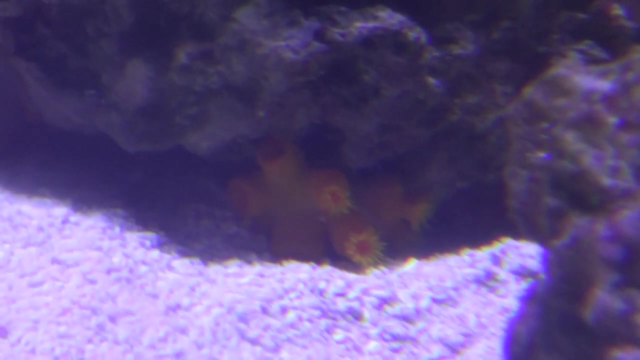 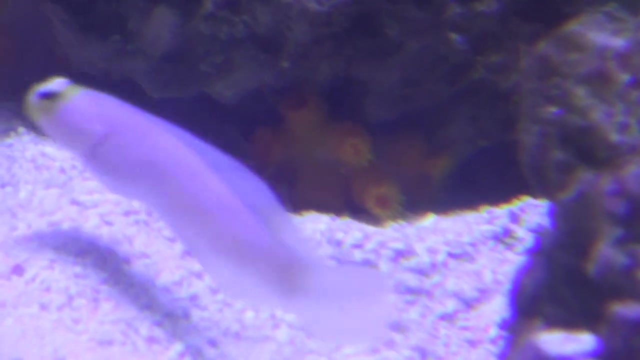 They don't have as many of those zooxanthellae that Joe mentioned earlier, And so therefore they can habitate at lower depths And they'll feed a lot more on phytoplankton and things like that. So now that we've learned many of the major types of coral, 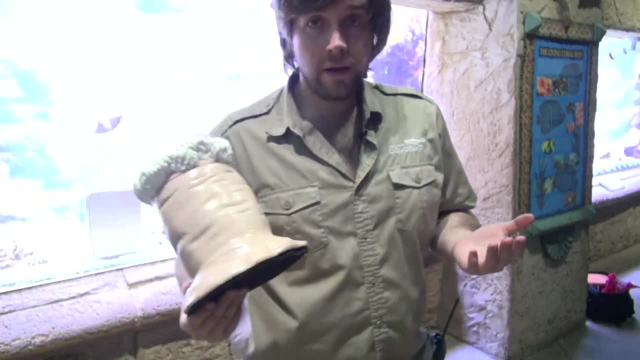 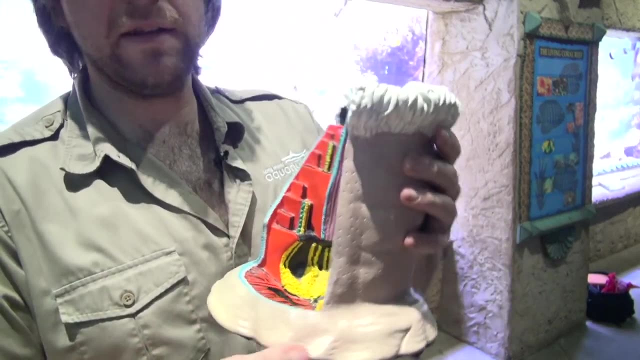 I thought it would be a good idea to review the anatomy of a coral polyp. So here's our model of the polyp once again, And notice that if I spin it around like this, we can get a better look on the inside of the polyp. 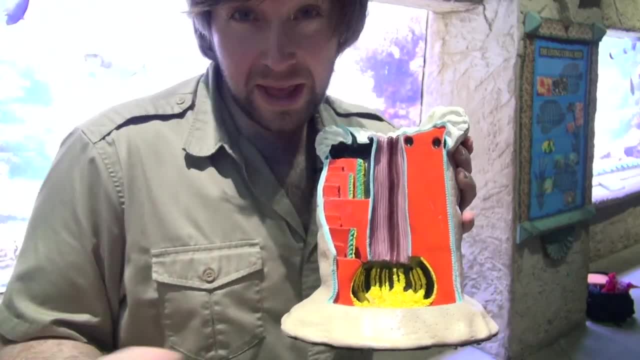 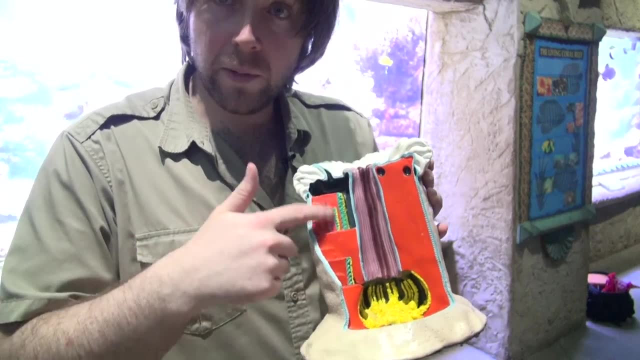 Now each polyp. they're pretty simple animals. They only have three tissue layers. There is the outer layer, known as the epidermis. There's this sort of middle part in here which is known as the mesoglia, And then there is the internal tissue layer. 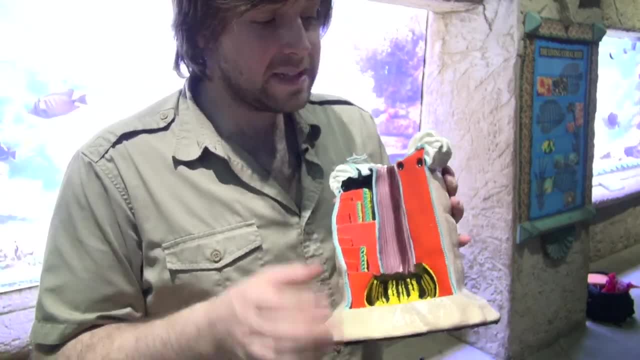 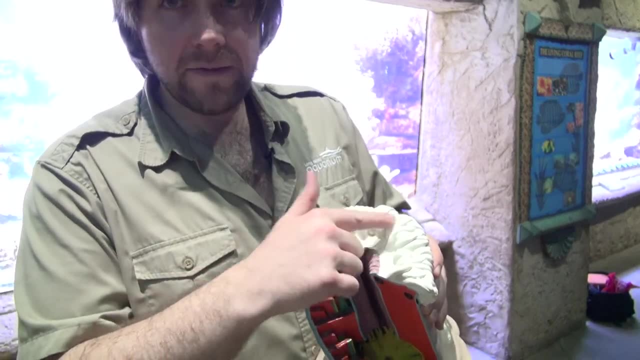 known as the gastrodermis. Now, the gastrodermis contains little tissue folds known as mesenteries, And this is where all digestion takes place. So up on the top here we have tentacles surrounding the mouth of the polyp, And these tentacles contain stinging cells. 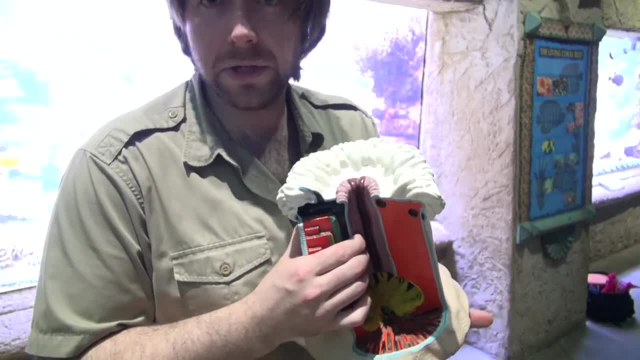 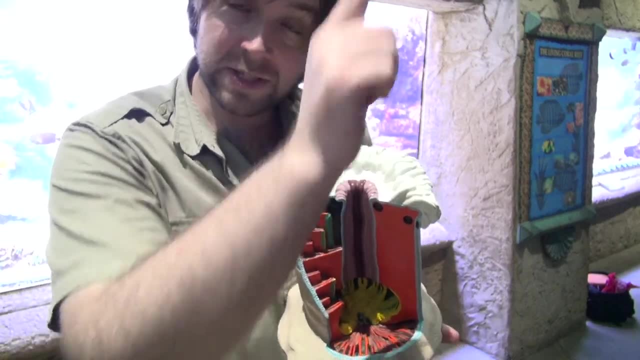 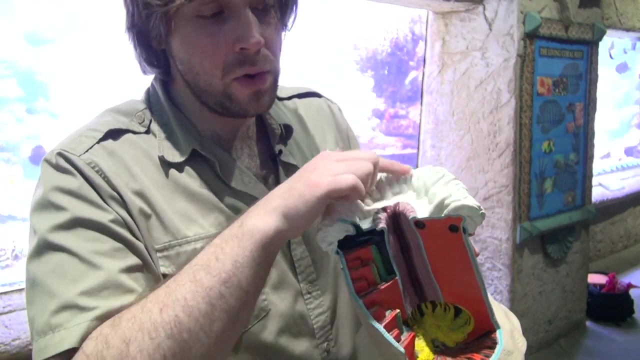 which are activated via touch. So there's actually a little receptor, a little hair that, when triggered, it will trigger the shooting out of one of these little nematocyst barbs which contains venom, which will paralyze prey And then the tentacles can work to move that prey item. 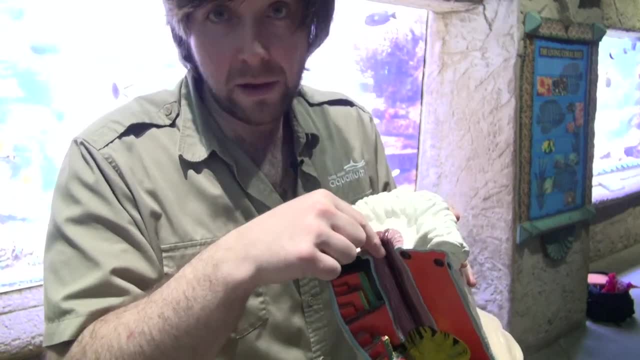 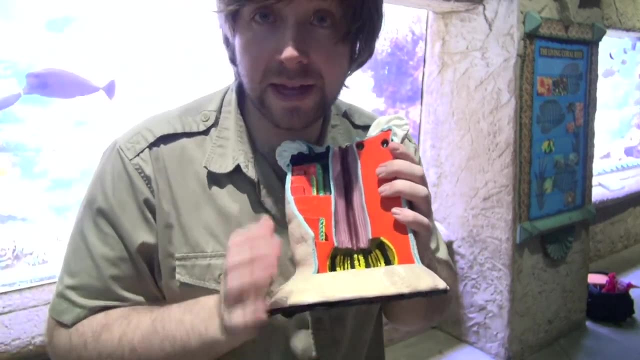 or that food item whatever, into the mouth here, which again doubles as mouth and excretory pore. The food will pass into the mouth and will enter into the salenteron, So that's the digestive body cavity, essentially of the polyp. 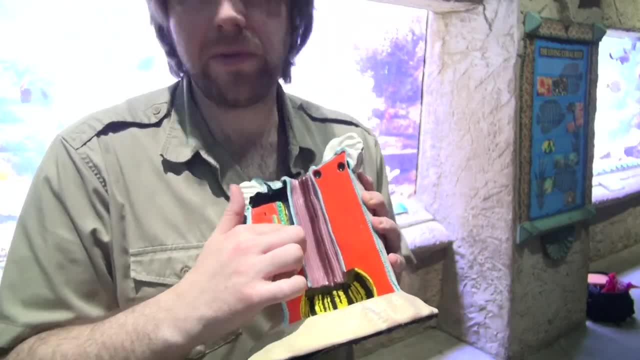 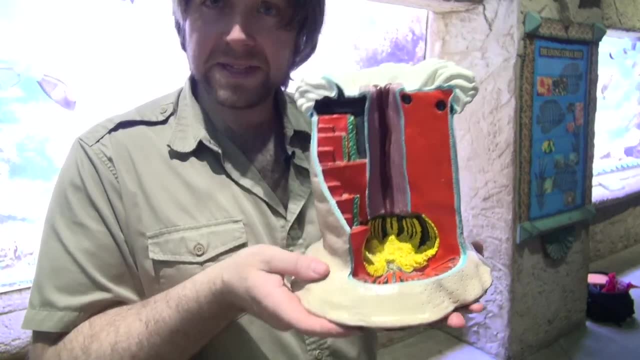 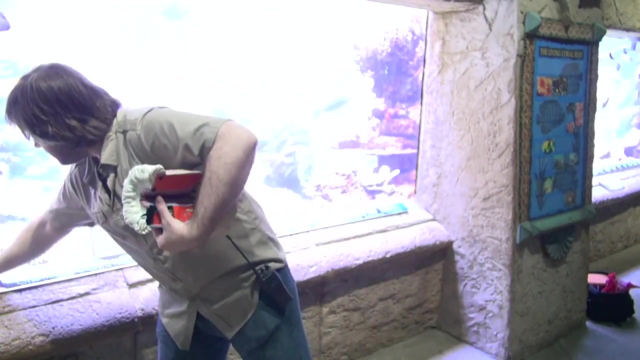 And nutrient absorption and digestion takes place with the help of the gastrodermis, that tissue layer on the inside. here Now, each one of these polyps lives on a colony, in a structure known as a corallite, And so I have an actual endoskeleton here of a coral. 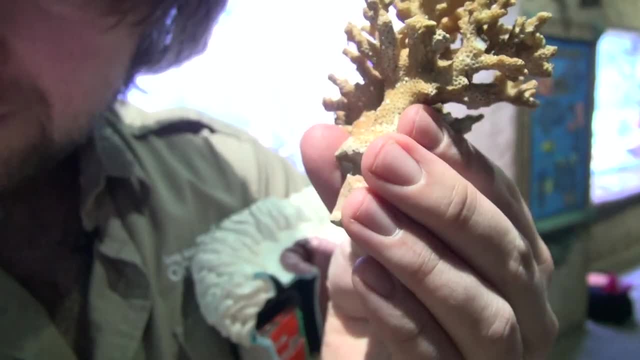 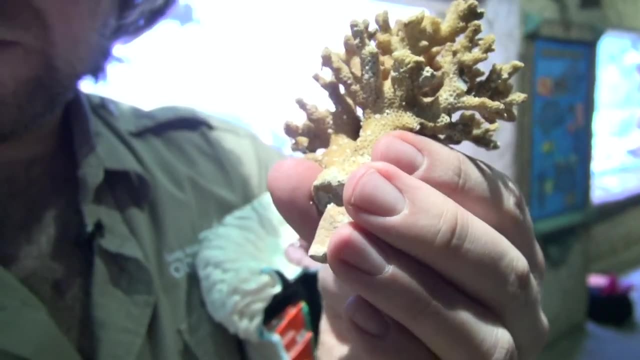 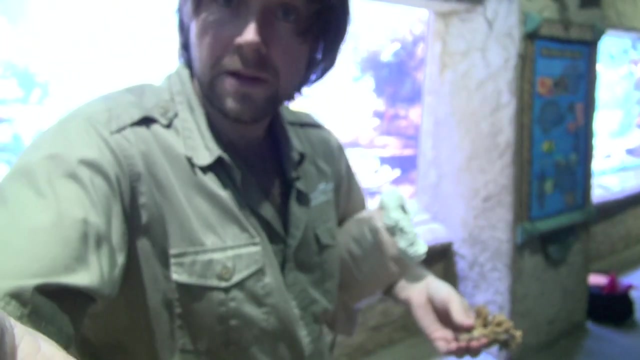 And if you notice all of those little depressions on the surface of the calcium carbonate skeleton there, all of those represent little corallites, which was where polyps once lived, And so I like to think of the corallite literally as the house for the polyp. 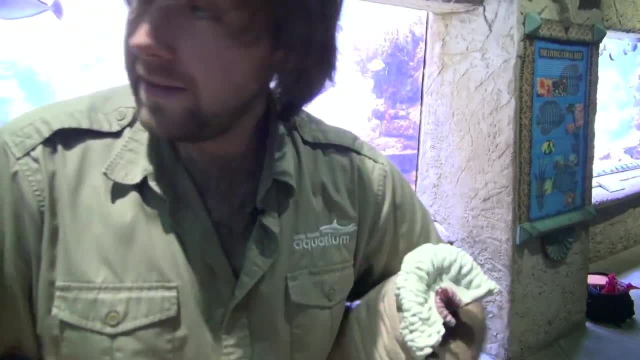 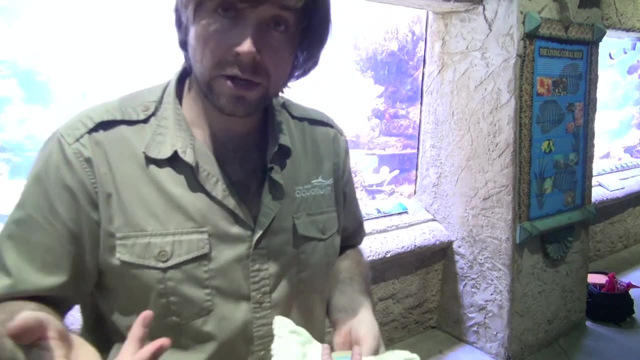 So the polyp will spend all of its time living in that corallite And, like Joe said earlier, they can retract at various different points of the day, whether it's for nutrient, whether it's for energy consumption, for conservation, for avoiding predators. 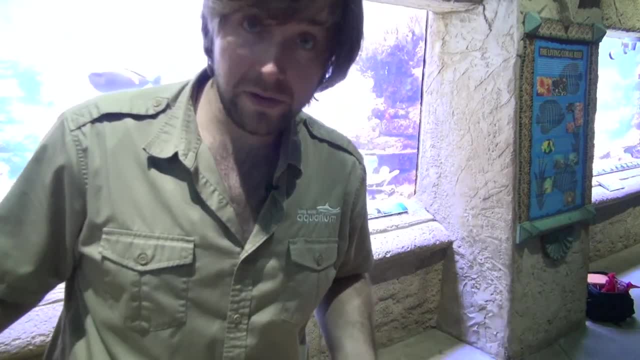 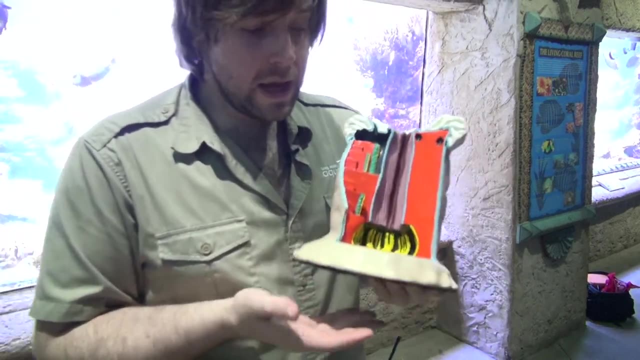 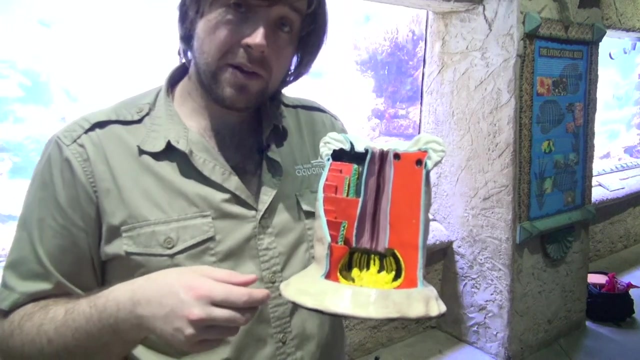 or just because they don't have to be out. There's no food available at that time, And so the coral polyp itself actually secretes calcium carbonate. It builds that calcium carbonate skeleton beneath it, And we're going to talk about that momentarily. 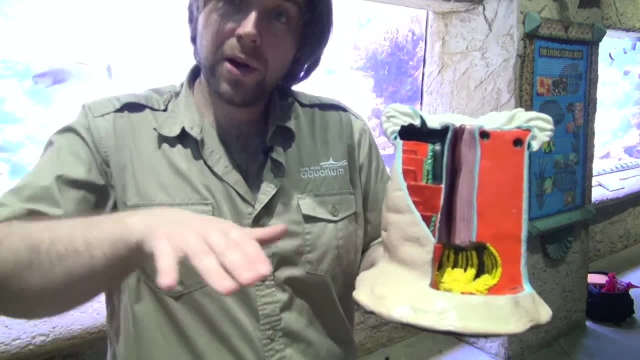 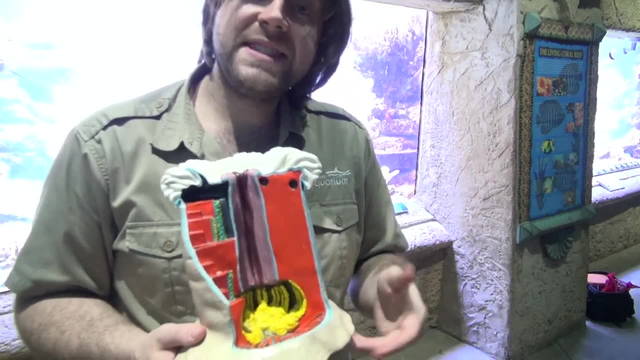 But what I wanted to point out is this little fleshy part. right here This little fleshy part goes out and connects to other polyps in the same calcium carbonate skeleton, in the same colony That's called the cenosarc. 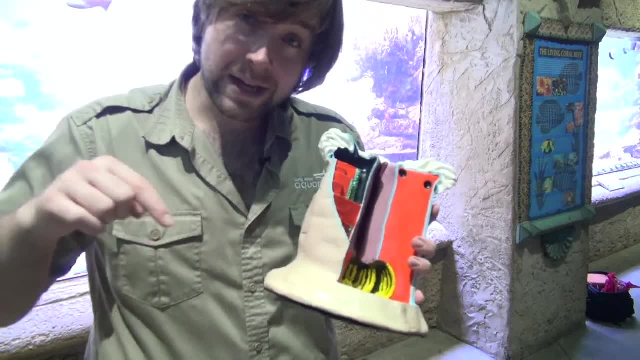 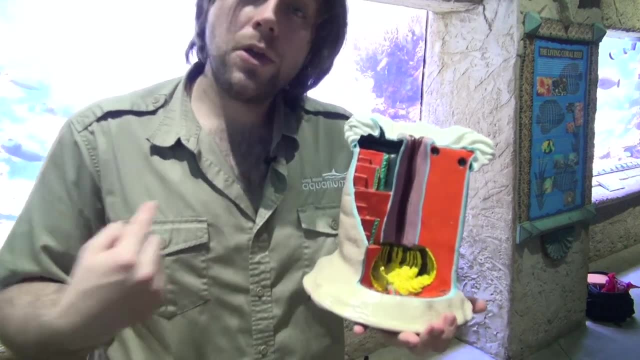 And that's a pretty amazing tissue layer. So this fleshy tissue layer actually connects one polyp to another on a colonial coral And, believe it or not, they can actually share nutrients through that cenosarc between polyps. That's pretty cool. 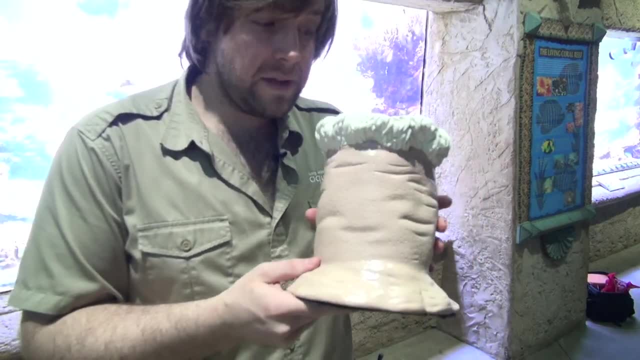 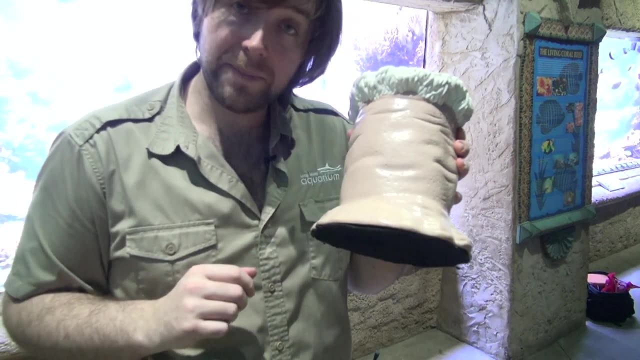 It's a little nifty feature, And the photosynthetic zooxanthellae that Joe mentioned earlier all exist within the polyp itself, within the tissue layer of the polyp itself, And so let's take a look at how the polyp actually builds. 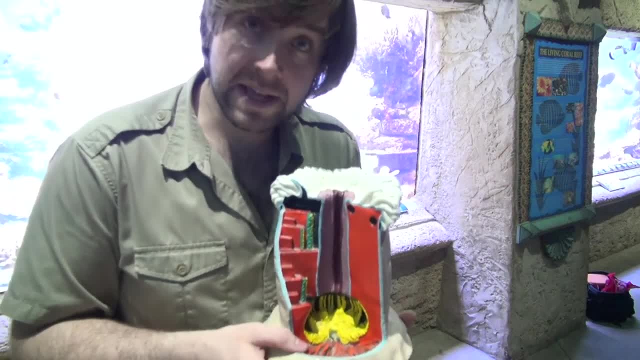 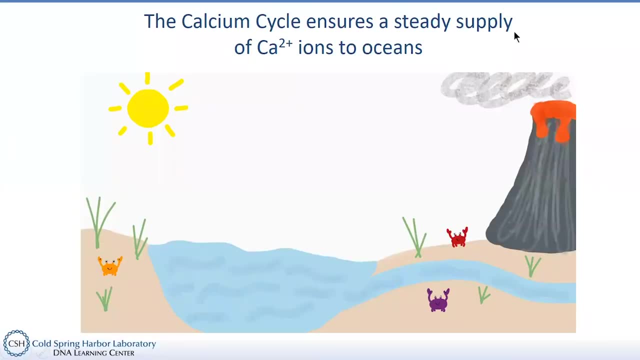 its calcium carbonate skeleton, And it does so by extracting nutrients from the ocean itself. Let's take a look. So, in order to understand how corals produce calcium carbonate for their skeletons, it's important to understand where the constituent ions of calcium carbonate come from. 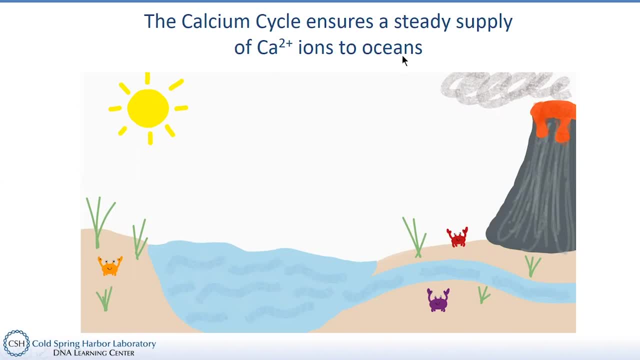 that being, of course, calcium and carbonate ions. Now, calcium is pretty straightforward: That comes from the calcium cycle, And the primary source of that is carbonate minerals from the Earth's surface. So erosion causes those minerals to break down and calcium eventually makes its way to the sea. 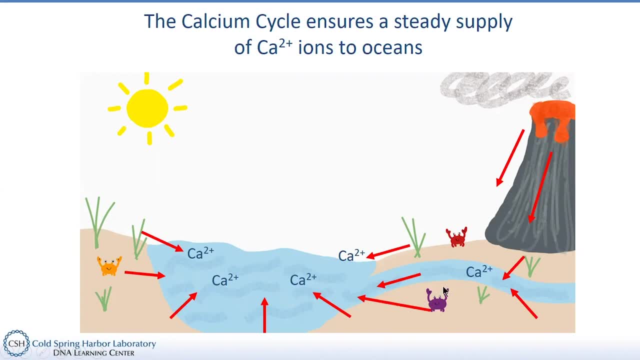 Living things also contribute calcium to the oceans in the form of their bodies. when they die, like these little crabbies here and the grasses, They contain calcium and then, when they pass on, their bodies will eventually decay and calcium will eventually percolate into the soil. 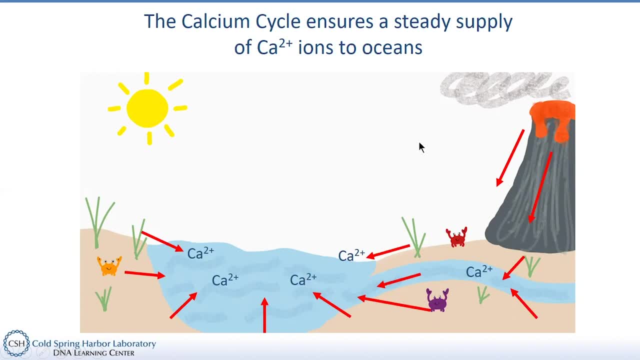 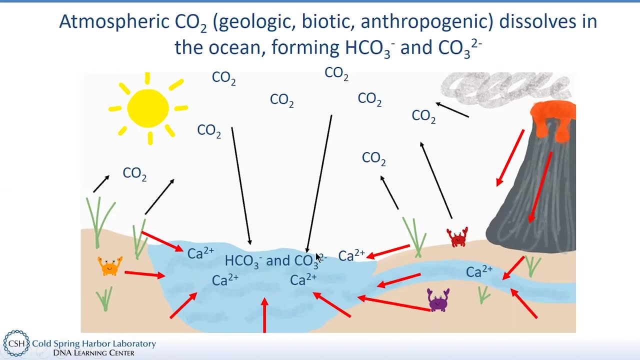 and make its way to the sea. Now, carbonate, on the other hand, comes from atmospheric carbon dioxide. So while the concentration of calcium is relatively consistent throughout the depths of the ocean, carbon dioxide is a little bit different, So it will dissolve into to a certain extent. 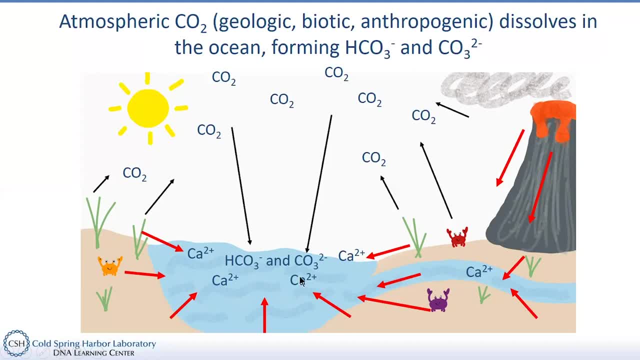 it will dissolve into the surface waters of the oceans And when it does so, it will form several ions, in particular bicarbonate ions and carbonate ions, And this is important, And the amount of carbon dioxide in the atmosphere will directly affect how much will be produced. 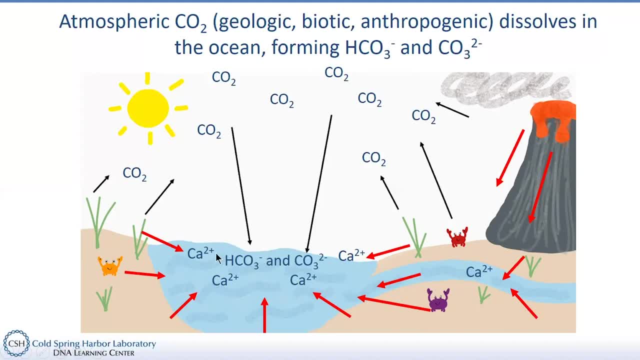 will dissociate into the sea among other factors such as temperature, pressure et cetera, But that is where the carbonate comes from that coral will eventually use, And you know, the sources of atmospheric carbon dioxide come from the Earth itself, from volcanoes and seismic activity. 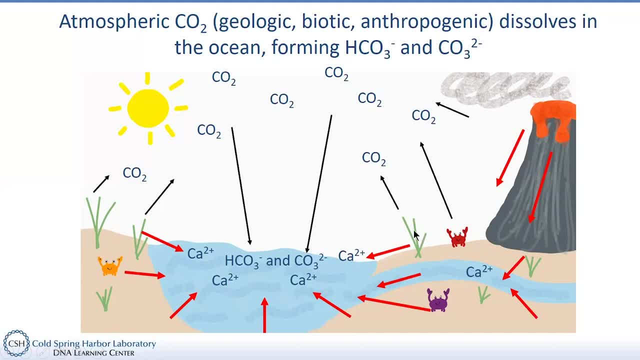 from living creatures like crabby and the grass here that produce carbon dioxide through cellular respiration and also human life. So we can see that in the environment the carbon dioxide is actually a very important factor in the form of the farming industry, et cetera. 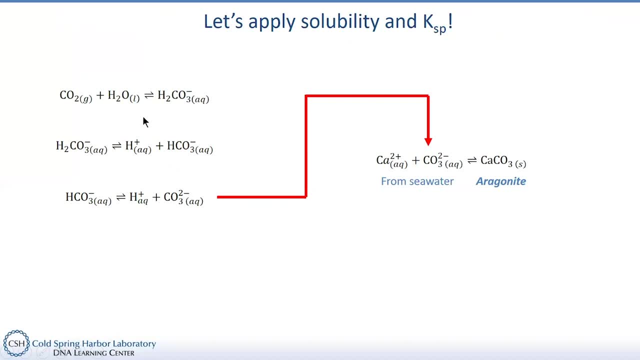 Now to understand how the solubility of carbon dioxide works. let's first understand what solubility is. So we're going to go back to chemistry now. I hope you don't mind. It's not too bad. This looks very intimidating, of course. 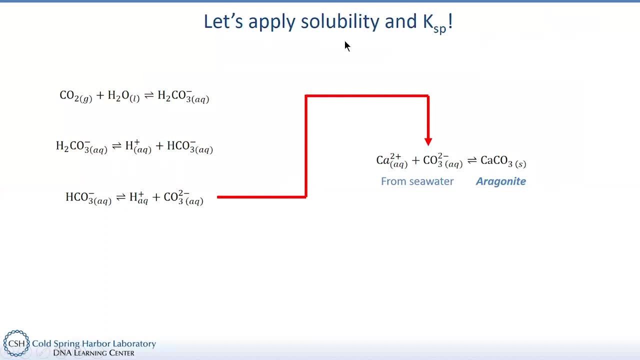 but it's really quite easy. And, first of all, solubility basically means the amount of something that will dissolve in another substance, And we also- I also wanted to bring up this comment- I also wanted to bring up this concept of KSP. 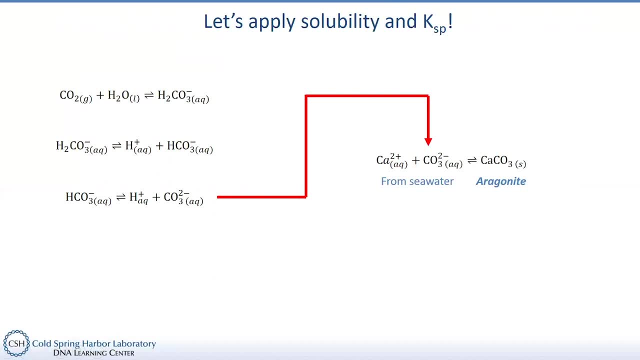 the solubility product constant, And so if you've taken AP Chem or undergraduate chemistry, intro chem, you probably are familiar with this, and it may have seemed very annoying and obnoxious, but it actually does have practical application here when we're talking about ocean chemistry. 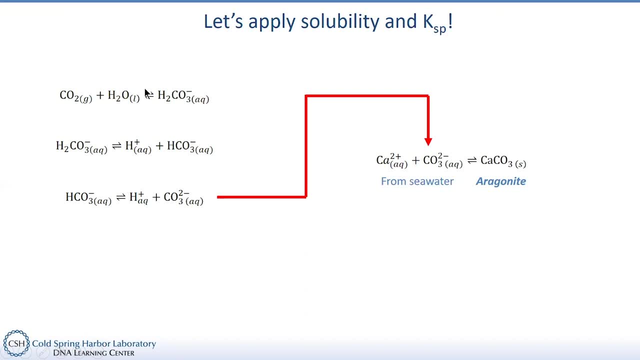 So let's get into it. So basically, carbon dioxide dissolves in seawater to produce carbonic acid. That carbonic acid, because it's an acid, will dissociate And because it's a diprotic acid, it will. 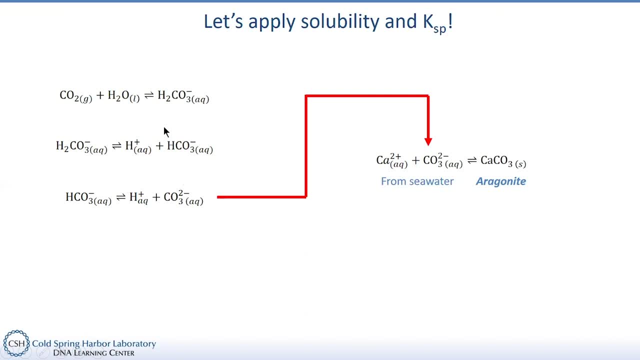 it has two dissociations. The first one will produce bicarbonate ions. Now, this is the primary dissociation that goes on in ocean water, so, but secondarily, however, this bicarbonate will lose a second proton to become carbonate ions. 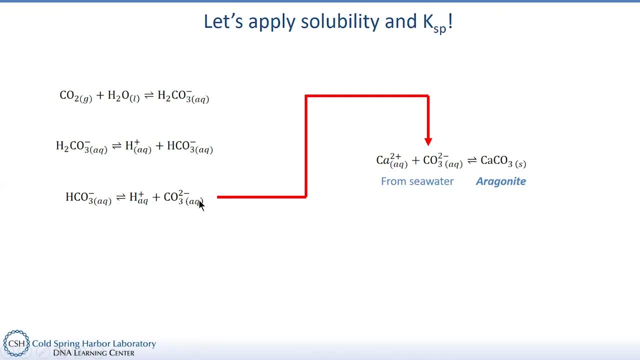 And this carbonate ions. these carbonate ions can be directly used by corals to produce calcium carbonate, And so the it's a very simple process: simply just combining calcium ions and carbonate ions to produce calcium carbonate, Solid calcium carbonate And the particular version of calcium carbonate that I wanted. 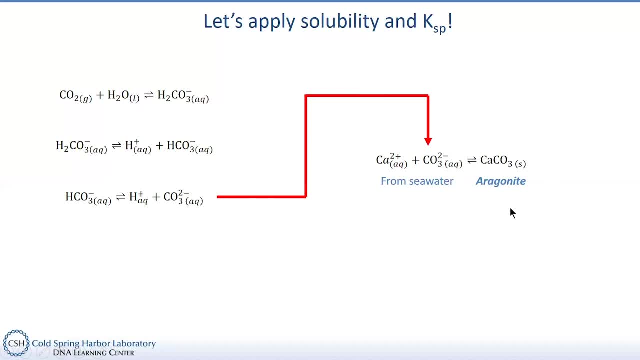 to talk about is the one that stony corals produce, So those are those scleractinian corals, And they produce this mineral known as aragonite. Now, calcium carbonate can occur in many other forms, but aragonite is the one that I'm going to be focusing on now. 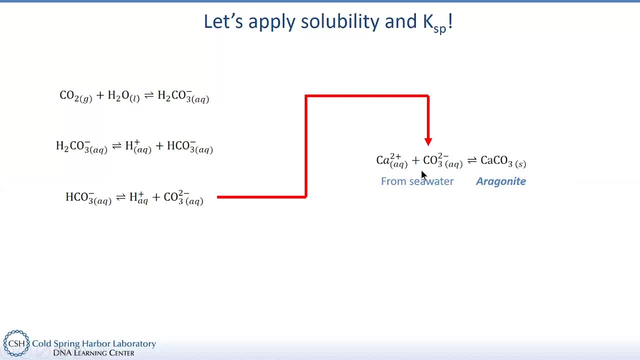 And so they produce that from calcium ions from directly from seawater as well as carbonate ions from directly that have that are just floating around in the seawater as well as pulling a proton off it. And so if we look at the amount of bicarbonate, 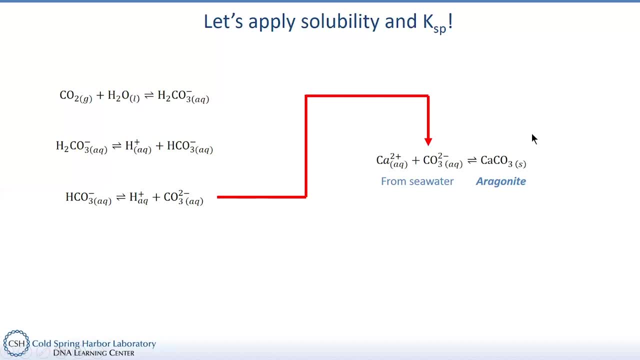 now, when we talk about the amount of aragonite that corals are able to produce and synthesize, it's important to understand the solubility product constant, So the amount of availability of these ions really matters when it's in terms of the ability of corals being able to produce. 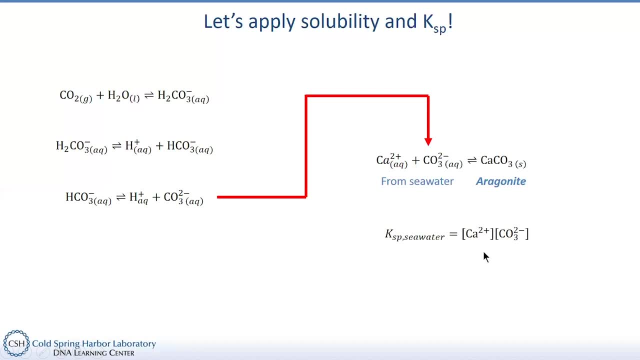 aragonite and build their skeletons. And so, like I said, calcium is pretty much evenly distributed, but carbonate here on the other hand that can fluctuate. It can fluctuate a little bit depending on several conditions, But the solubility product constant describes the dissociation. 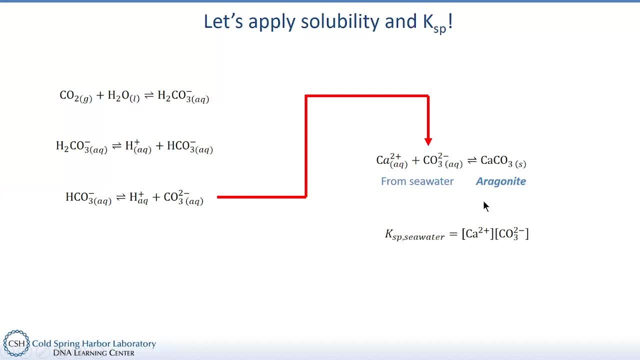 of calcium and carbonate into its constituent ions at equilibrium. So basically, to get that value, we would multiply the equilibrium values of the concentrations of calcium ions and carbonate ions under certain conditions, including temperature, pressure, etc. And that'll give us the Ksp. 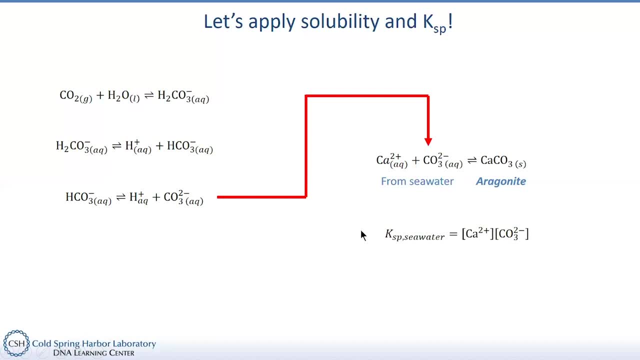 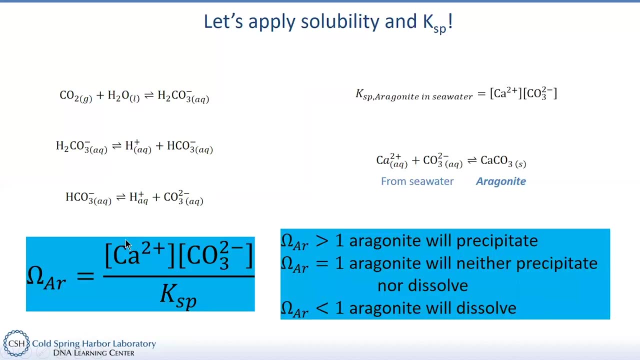 of calcium and carbonate in seawater. Now, when we are talking about the formation of aragonite, we can then expand that definition to this thing. Now this looks very, very scary, but trust me, it's actually pretty easy to understand. 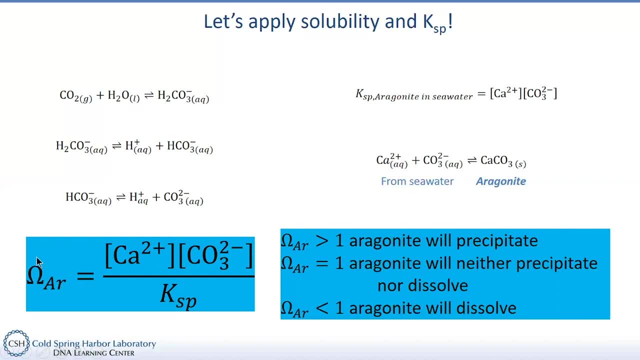 and it's actually pretty important to understand too for ocean chemistry. So this is a Greek letter omega and this is the aragonite saturation constant. So this constant essentially describes the concentrations of calcium and carbonate ions relative to equilibrium. that will predict. 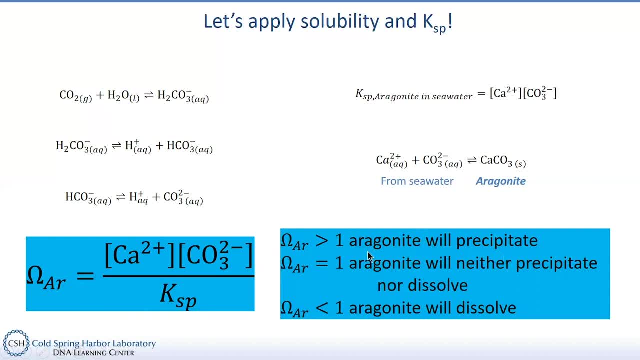 whether or not aragonite will more easily form or will probably not form at all. And so from chemistry back, from Regions chemistry or high school chemistry rather, we can figure out what the meaning of this kind of refers to. So when the saturation constant for aragonite is greater than 1,, 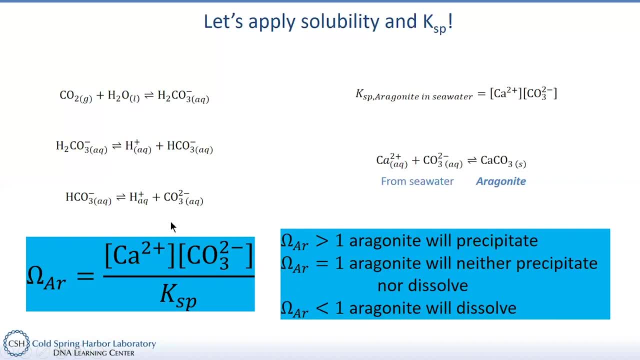 what that means is the current concentration. this is just any given concentration of calcium ions and carbonate ions in a particular solution when the saturation constant is greater than 1, that means that this top value in the numerator is greater than it would be at equilibrium. 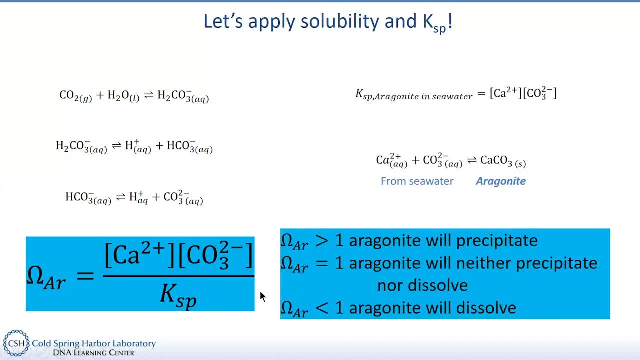 meaning that aragonite will precipitate or form solid in solution, Whereas when it is equal to 1 on the nose, that means that we are at an equilibrium point at which the top values are equal to the bottom values, And that will predict that aragonite. 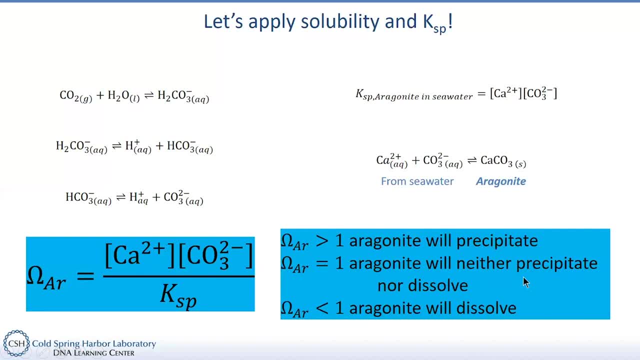 would neither come out of solution or dissolve into solution, Whereas when the saturation constant is lower than 1, that means that aragonite is more likely to dissolve out of solution. And so what this all means is that, depending on where corals might be growing or find themselves, 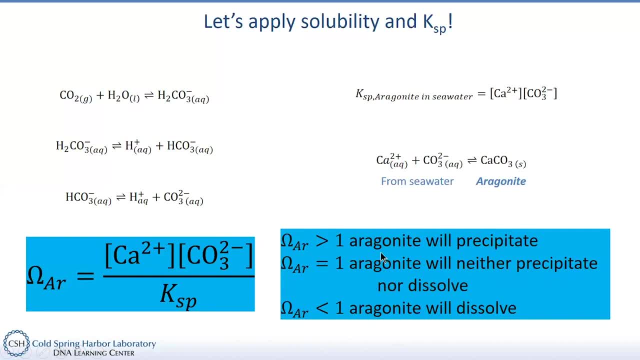 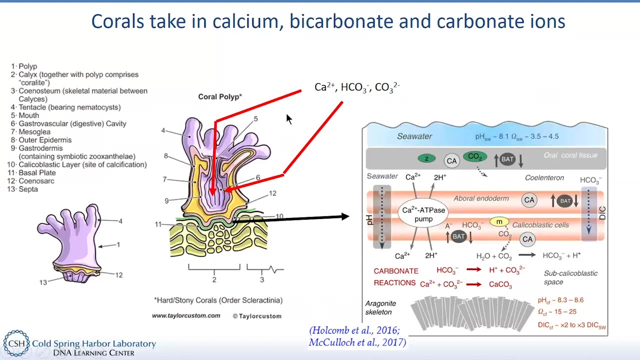 depending on the saturation constant of aragonite, at that point it's going to be a favorable environment or an unfavorable environment to producing calcium carbonate skeleton, And so we'll come back to this later, but for now, just remember that. Keep that in the back of your mind. 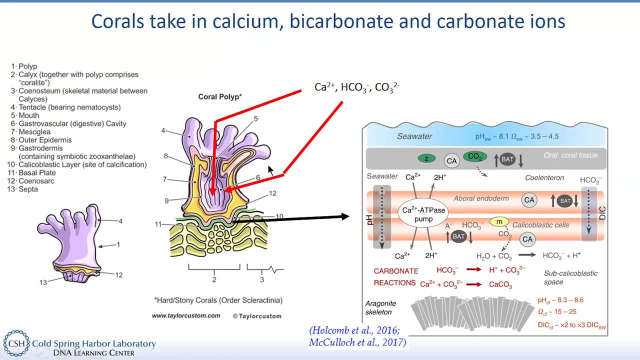 And so the calcium bicarbonate and carbonate ions that are floating around in seawater will eventually make their way to a coral polyp. So here's a polyp here, and just a reminder of the anatomy. We just learned this, so I'm not going to go through that again. 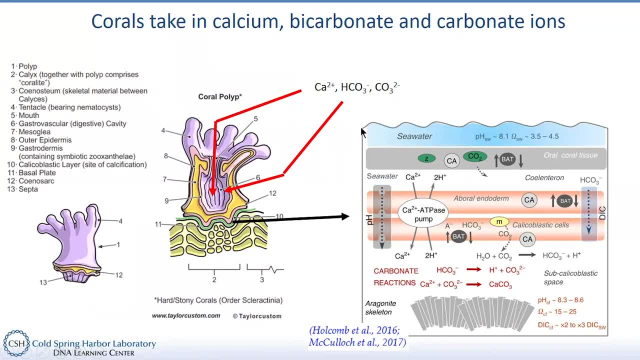 But essentially the ions go through the mouth of the coral or they might even to some extent go through, simply go right through the dermal tissues directly into the cilentron in the middle here, That's that body cavity again. They will then be further moved down here. 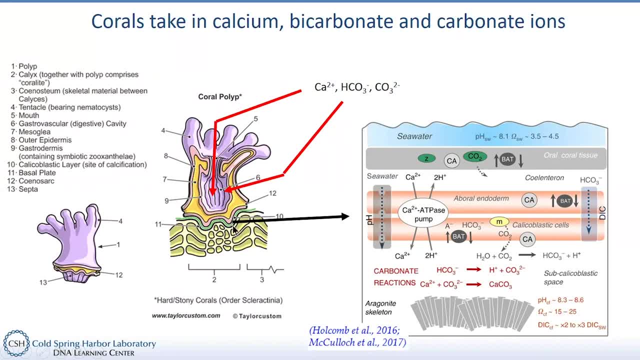 So remember, this is the base plate. So all of these structures, this is the calcium carbonate skeleton down here and this is the base plate underneath here, the basal plate And the green layer. here is what I wanted to focus on. This is a layer of cells known as. 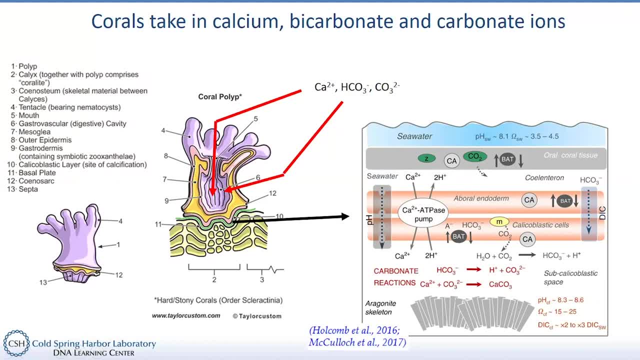 the calicoblast or the calicoblastic layer of cells. These are the cells that are responsible for producing the calcium carbonate skeleton, or at least allowing that calcium carbonate skeleton to form beneath them. So what winds up happening is these ions. 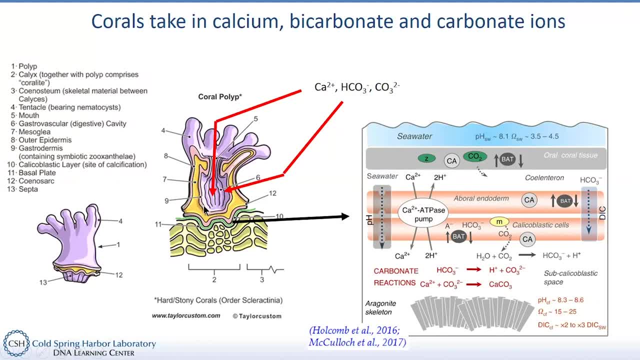 go into the cilentron. here Calcium diffuses via active transport so it takes energy to actually pump that calcium into the layer right beneath the calicoblast here. So if we take a blown-up image of that, we can see that right over here. 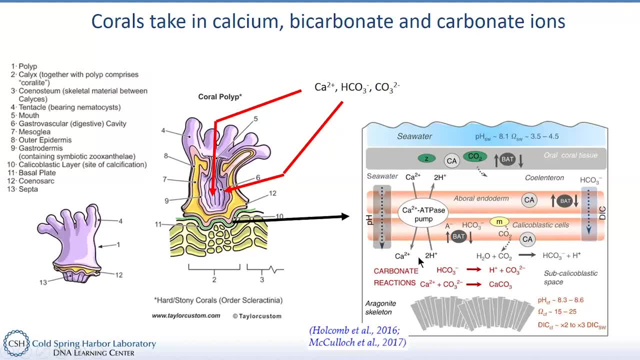 So here are the calicoblastic cells here, and we can see that energy is expended trying to pull those calcium ions right beneath that layer of calicoblast And they will then combine with carbonate that has been deprotonated down here in the subcalico. 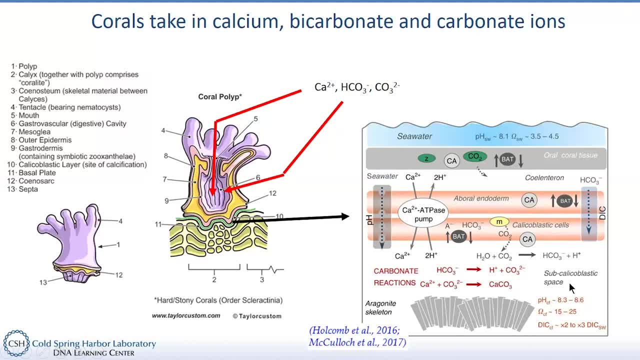 I'm sorry. they will combine with bicarbonate that's been deprotonated down here in the layer below the calicoblast. Now, remember, seawater's flowing all through here, and this arrow here is meant to indicate that seawater's flowing directly. 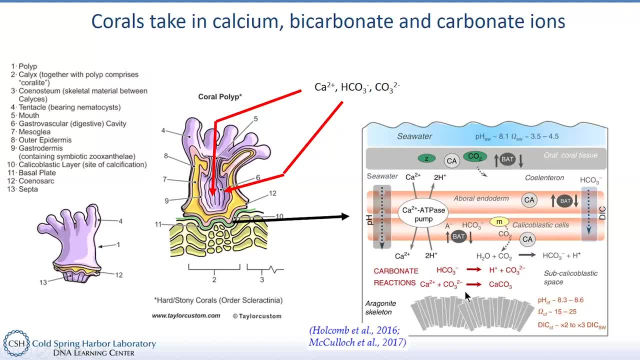 into that layer as well freely, And so, if there are carbonate ions available, obviously they are going to be combined with calcium ions much more easily than by having to remove a proton from the bicarbonate here, And so, either way, what winds up happening is: 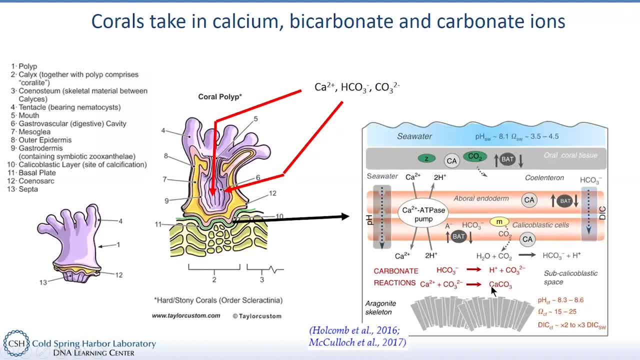 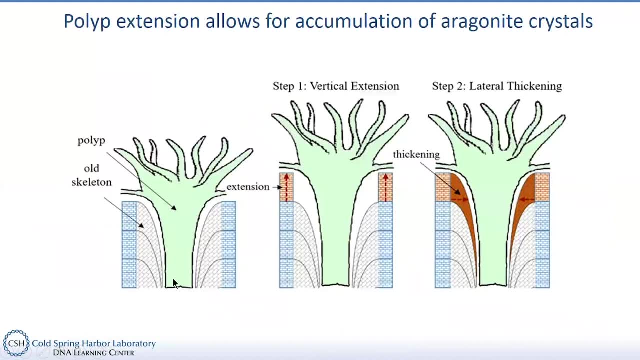 once they combine together, they will form a crystal of aragonite, or they'll begin to form a crystal of aragonite, And these crystals will layer themselves down here, And what winds up happening is the polyp will extend up out of its little corallite. 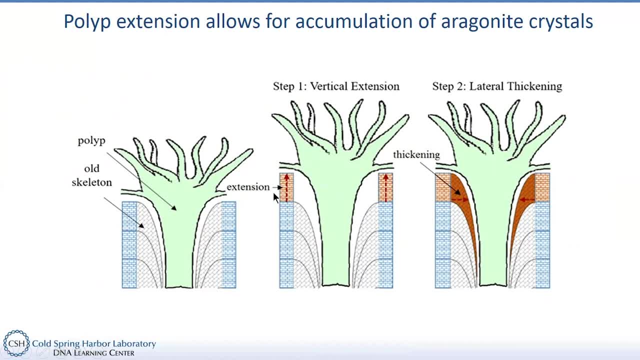 in the endoskeleton here, or the coral skeleton here, rather, and it will allow for that calicoblastic layer of cells to start depositing aragonite crystals both vertically and horizontally. So this will essentially allow for the coral branch itself to extend. 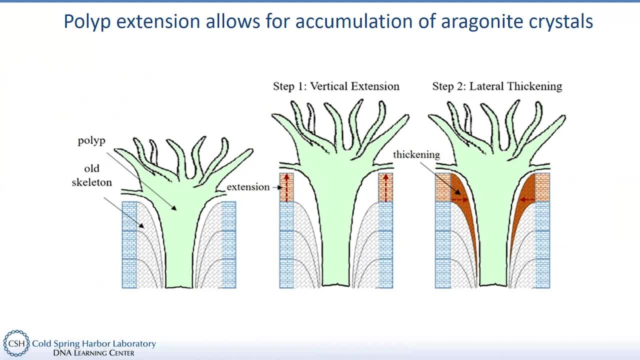 both axially and radially, meaning it'll grow in girth and length. And so, remember though, this is not reproduction, This is simply just growing that coral skeleton, It's fortifying that skeleton, And notice that this extension happens, So even the calicoblast here. 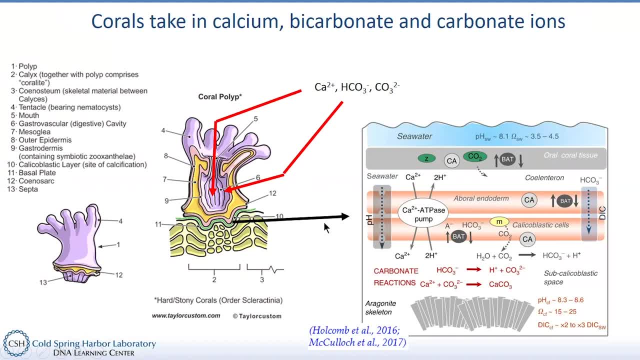 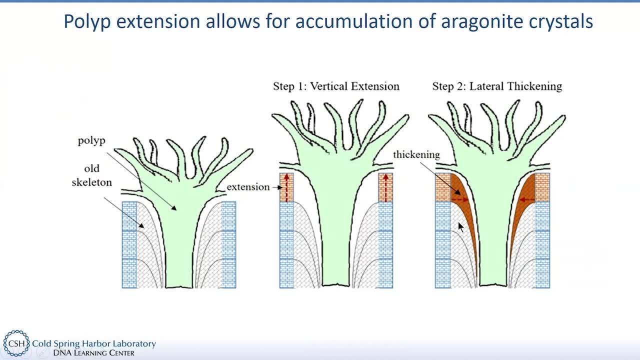 notice that it is below the coelosarca as well, So this is happening all over the surface of the coral colony, And so that's how we get to these big, gigantic branching corals. Now reproduction is a little bit different, however. 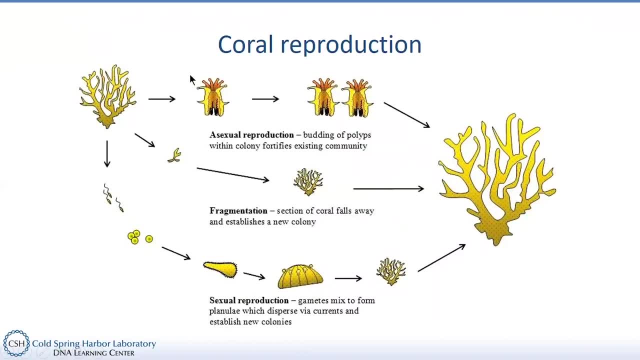 The individual polyps on those colonies will be reproducing through something like asexual budding or asexual reproduction and producing more clones of themselves to grow that colony and produce more polyps all over the branching structure of that colony. This gigantic colony can also break. 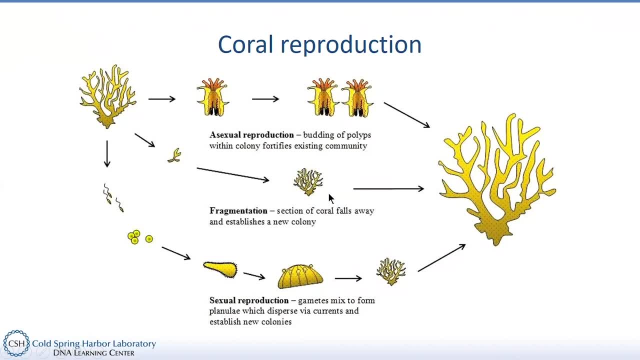 and little pieces of it can float away and be carried elsewhere and situate themselves somewhere else on the seafloor or on another part of the reef, and then they will establish a new colony there And that same process of skeleton building and asexual reproduction. 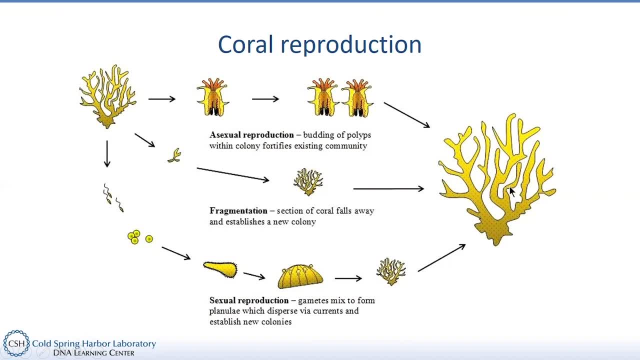 will continuously build that new branching structure to form a gigantic colony. But, believe it or not, corals can even undergo sexual reproduction, And they do so by releasing sperm and egg at various different points over the course of a year, And the sperm and egg will combine. 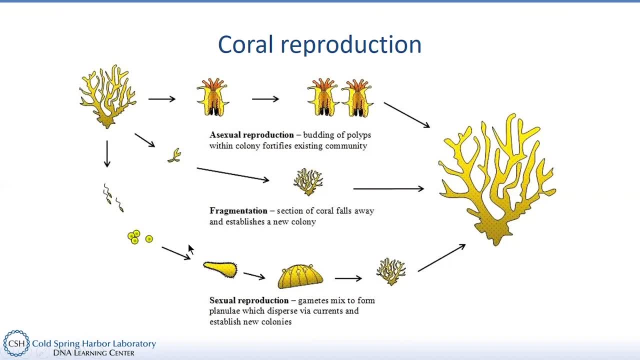 to eventually form a planular stage that will disperse through the oceanic, through oceanic currents. It's free swimming, I believe, to a certain extent, And it will eventually situate itself on a new location that have favorable nutrients and conditions for that particular species of coral to grow. 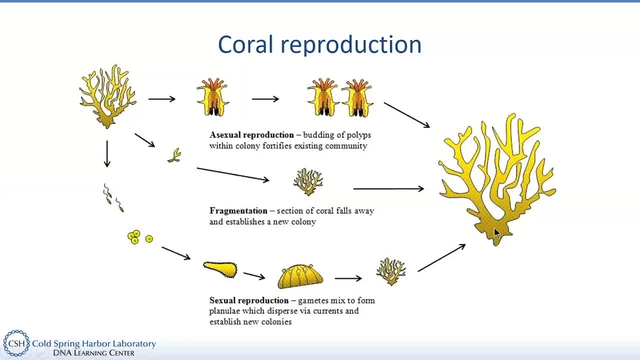 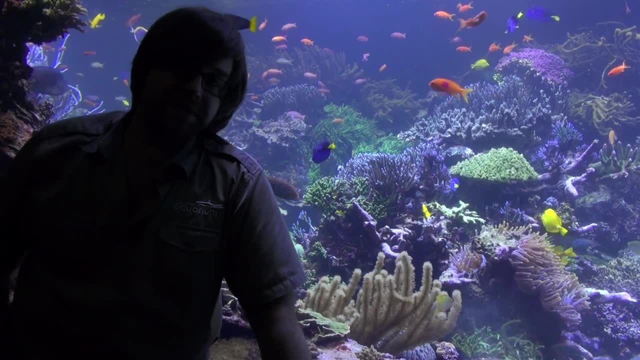 And that's how coral reefs extend themselves. Now let's take a look at some of the feeding mechanisms of coral a little bit more closely. So, as Joe was saying, both hard and soft corals have the ability to retract their polyps into their skeletons at various points. 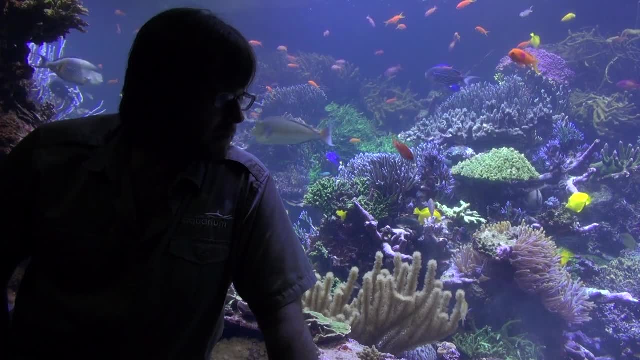 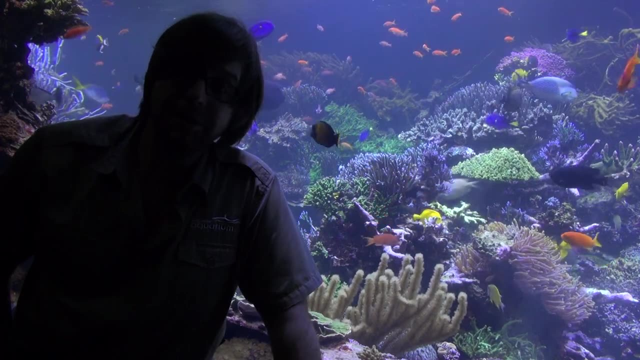 throughout the day, depending on you know, for one reason or another. So basically, they might go in, they might retract just because of energy conservation. They might retract because of a storm, They might have predators that are messing with them. 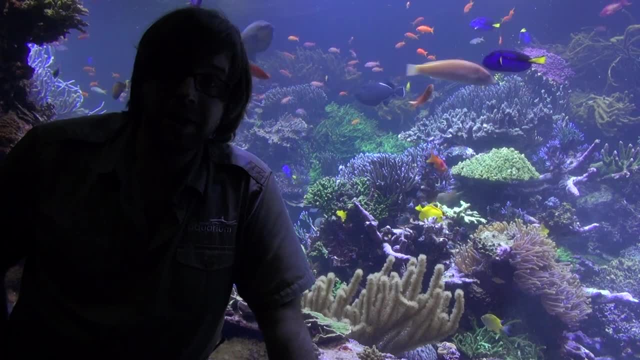 And, as you can see, the little yellow tangfish in here are going around picking at all of the different corals in here. They're eating, trying to go for polyps and things. So the fish actually present a pretty great risk to corals. 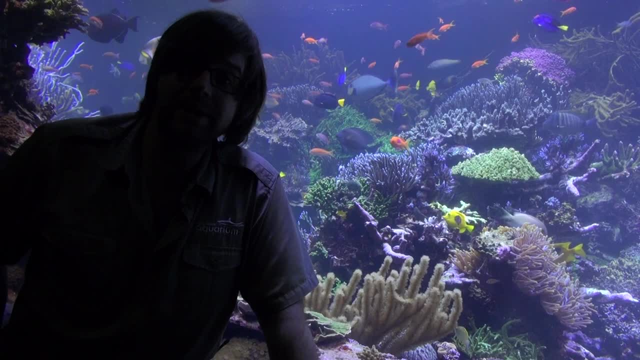 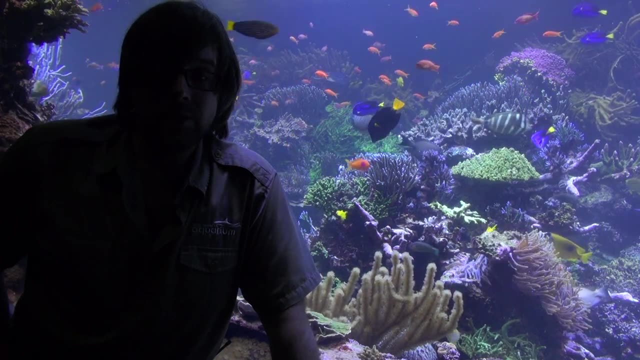 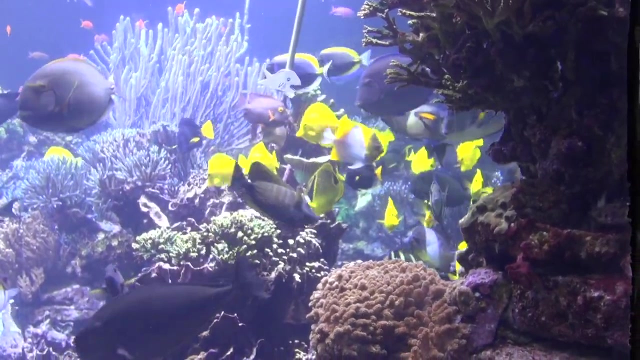 And so, in order to deal with that, retracting is a good way to avoid getting eaten by predators. So let's take a look at a soft coral: how it responds to a potential predator. So a lot of corals are a food source for fish. 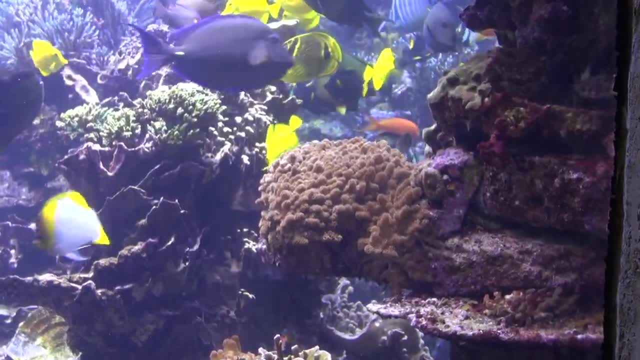 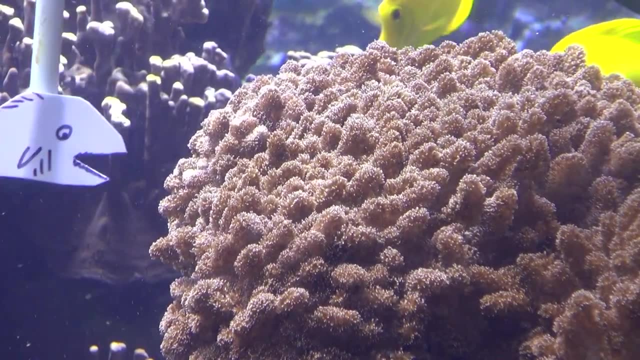 and they have a means of protecting themselves from predation. And we're going to pretend. here comes our little fish who likes to nibble on some of these soft corals, And you can see the polyps are out and how fuzzy the coral is. 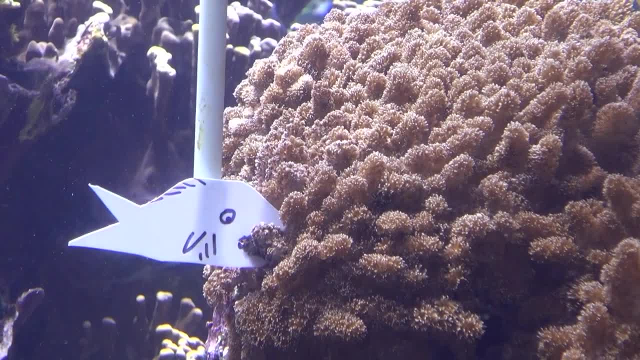 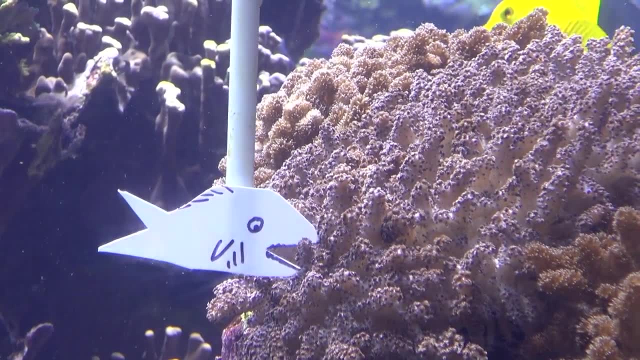 But if I was a little predatory fish here and I start chewing on this branch, you can see how fast the polyps do retract And that's a way of them protecting themselves. They'll pull their polyps in and completely retract And you can see the rest of the colony. 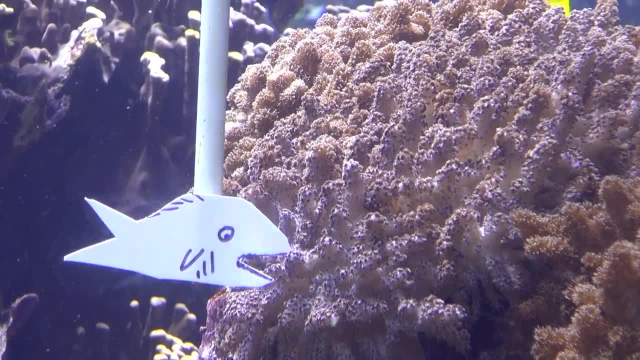 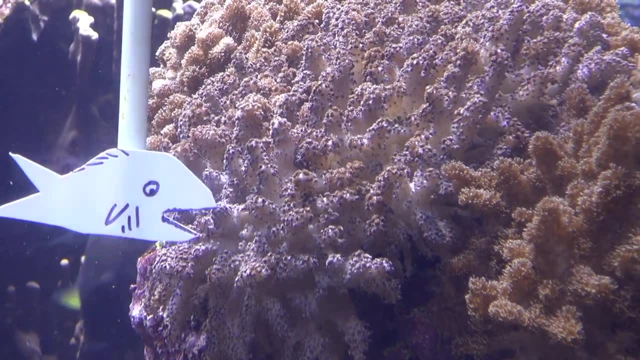 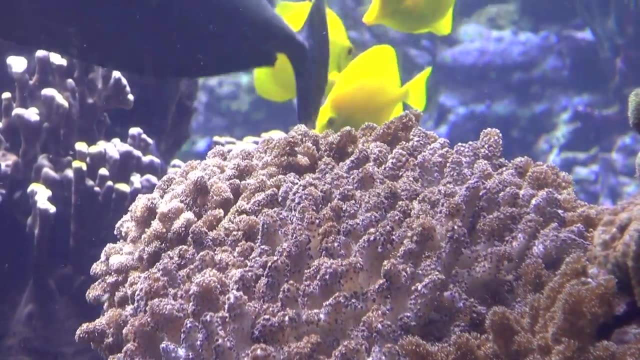 also reacting to what might be a predatory fish nibbling on some of the corals, And this way the polyps are protecting themselves. And then, when the danger passes and the fish swims away, there he goes. the corals will open back up again. 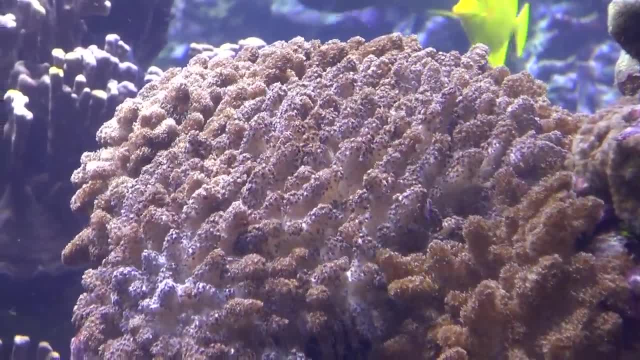 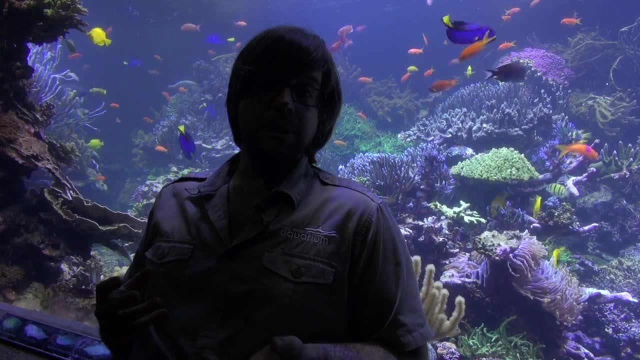 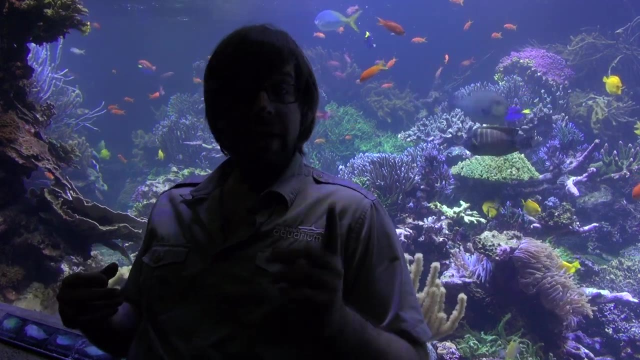 once they feel the danger is gone. So, as Joe said, it's never a good idea to deal in absolutes when we talk about science, especially when it comes to coral, just because there are so many different types out there with so many different behaviors. 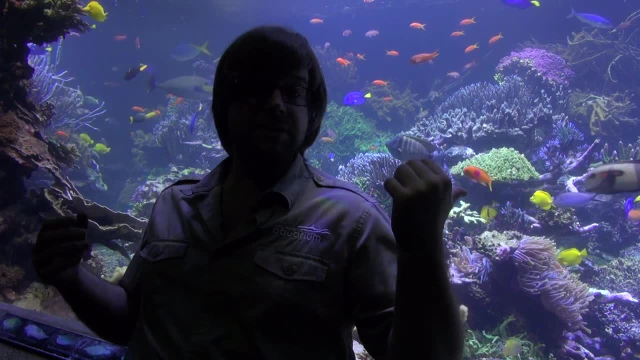 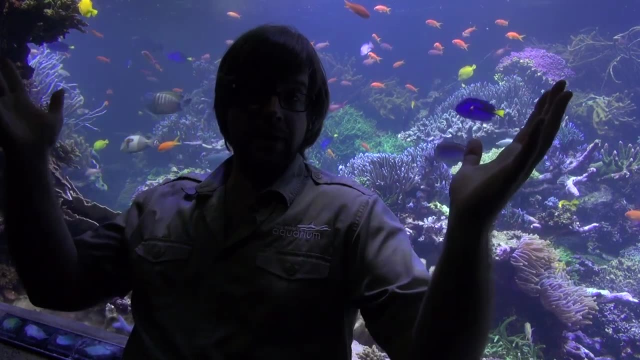 However, when we were filming today, you may have noticed that a lot of the stony corals were retracted, Their polyps were retracted, Whereas the soft corals, like the gargonia, were out and about, Their polyps were extended. 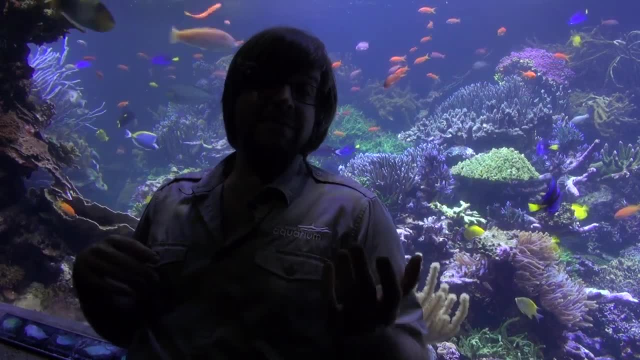 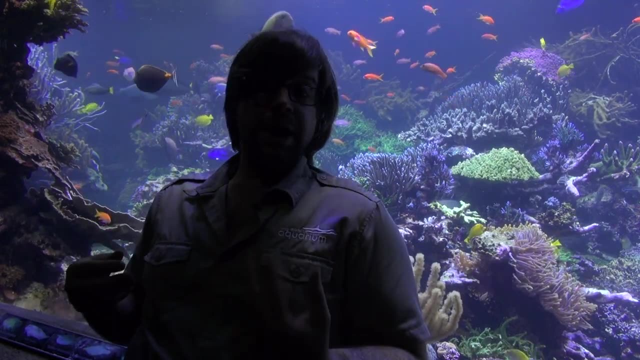 their tentacles were flailing, etc. And a lot of that behavioral difference comes from the types of food that both of these corals like to feed on. So, generally speaking, a lot of those stony hard corals really enjoy taking advantage of zooplankton. 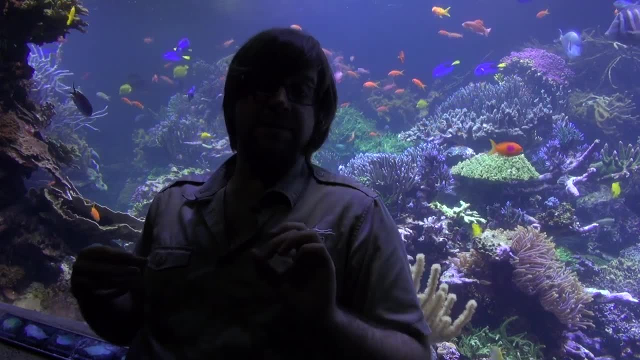 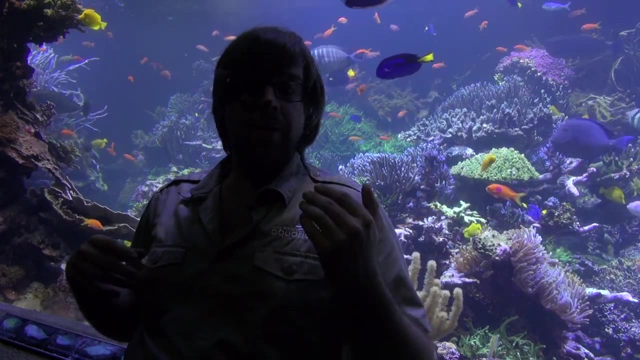 They like to feed on little microscopic planktonic organisms- animals, that is, that are floating around in the water column, And unfortunately a lot of those zooplankton are not really at the surface during the day, So a lot of them like to hide in the depths. 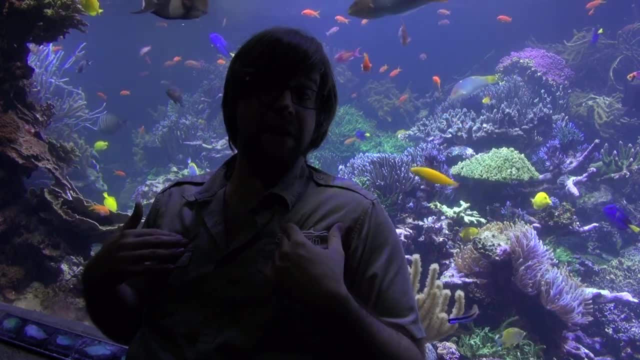 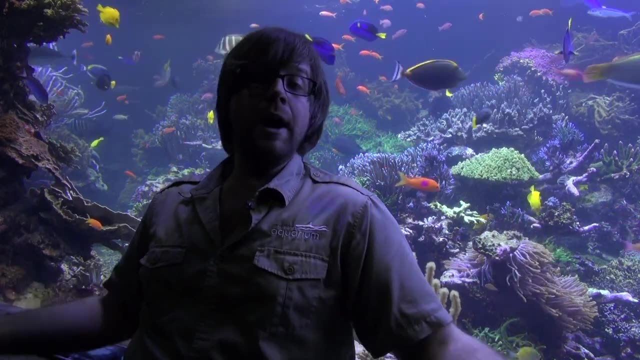 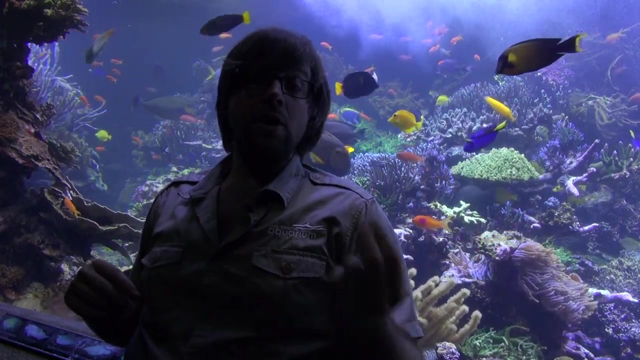 away from predators, So they themselves don't get fed upon, And so, every night, these little planktonic organisms will rise from the depths up to the surface in a major migration known as the marine dial, And this is one of the largest animal migrations on Earth. 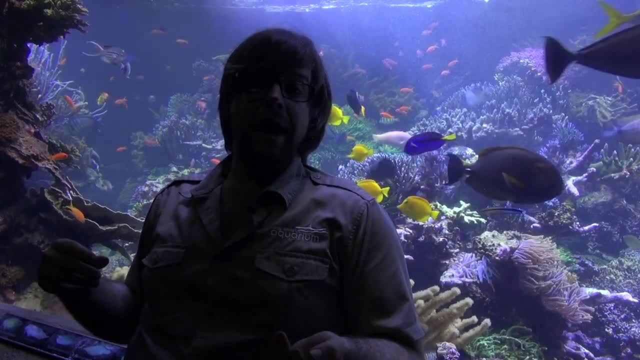 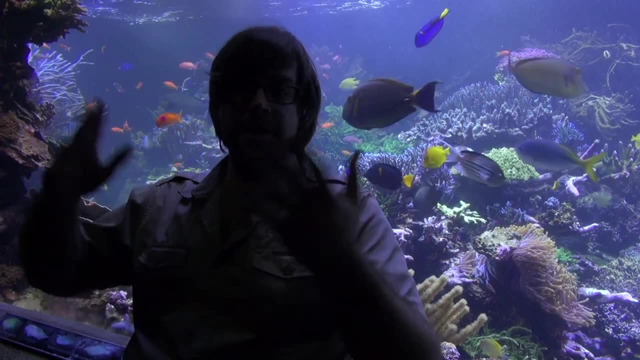 Actually, it is the largest animal migration on Earth in terms of the number of animals involved And basically you have fish, larvae, crustacean larvae, cnidarians, all kinds of things essentially coming up from the depths and they go to the surface to do whatever they got to do. 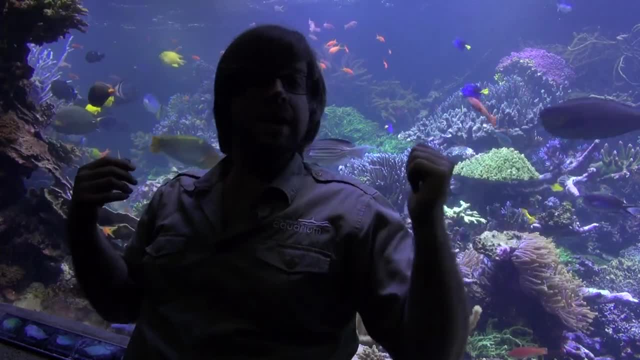 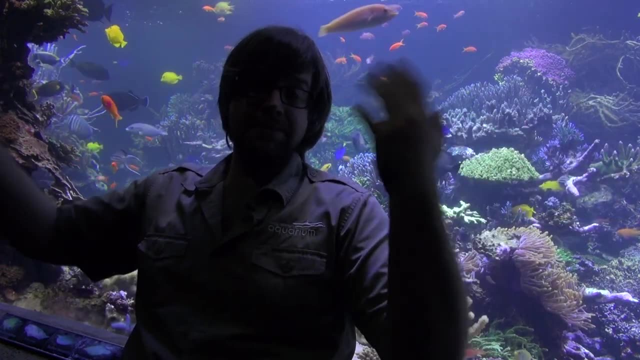 and free from, hopefully, predation. And so these hard corals, these stony corals, will then send out their polyps at night and they'll be able to take in some of those organisms. Right now, the reef tank is essentially daylight. 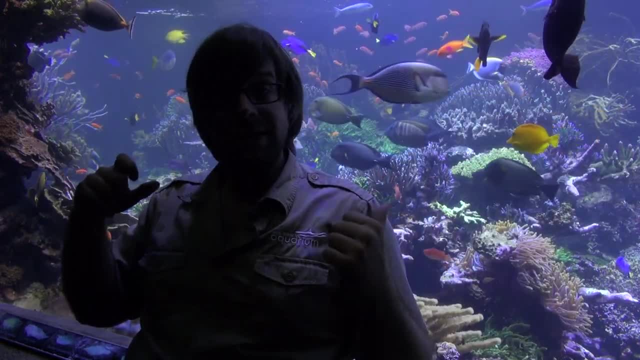 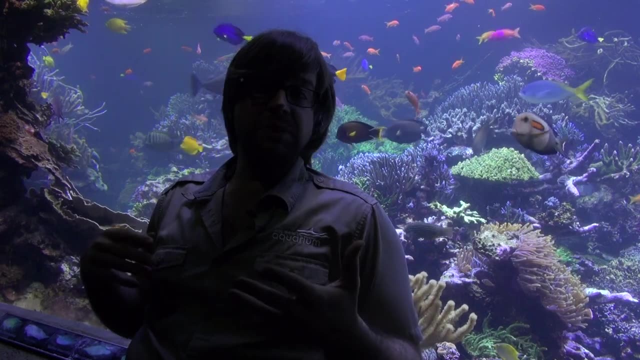 You can see the daylight bulbs are on right now, So all the corals in here think that it's day, Whereas the soft corals, on the other hand, they're not necessarily feeding as much on zooplankton, generally speaking. 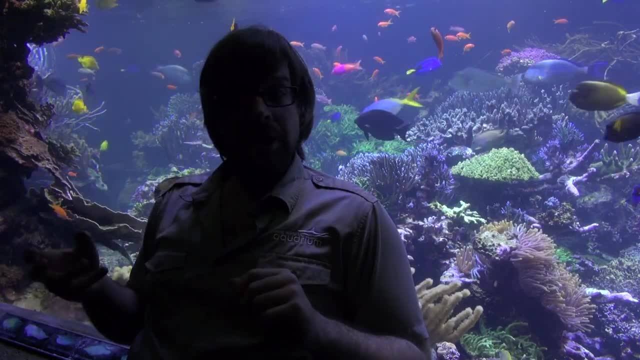 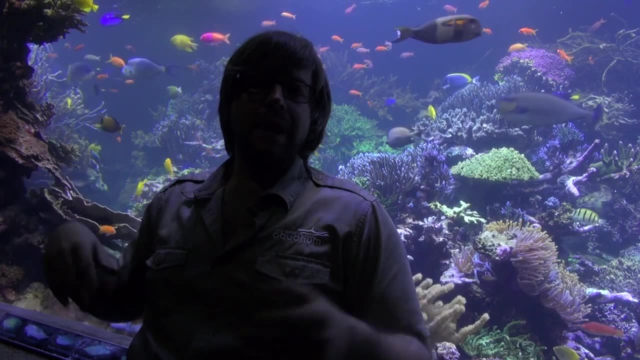 They like to take advantage of what are called phytoplankton. Phytoplankton are planktonic plant forms, And so basically single-celled algae and things like that that are floating around in the water column And they carry out photosynthesis. 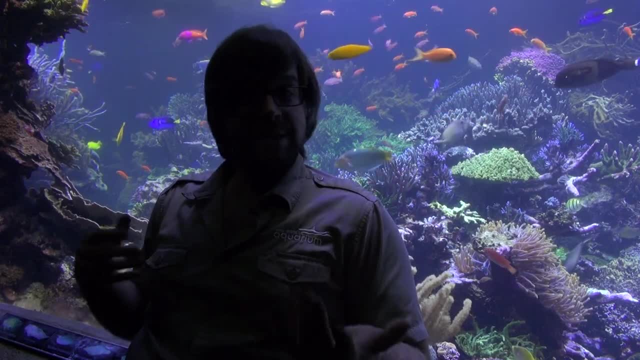 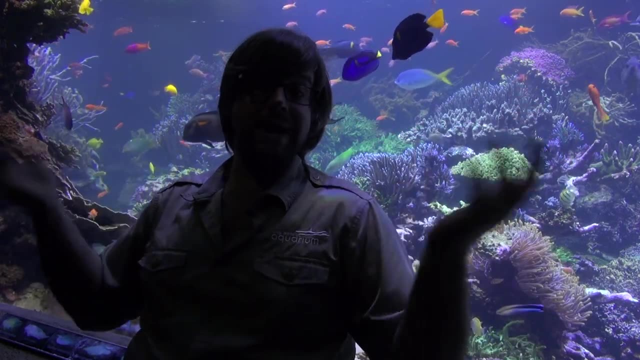 meaning that they need light in order to produce their own food, So they tend to be a little bit more active during the day at the surface. So these soft corals can take advantage of them as a food source And they'll be able to become active during the day. 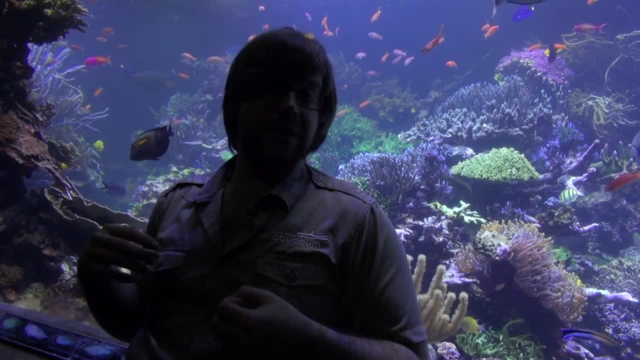 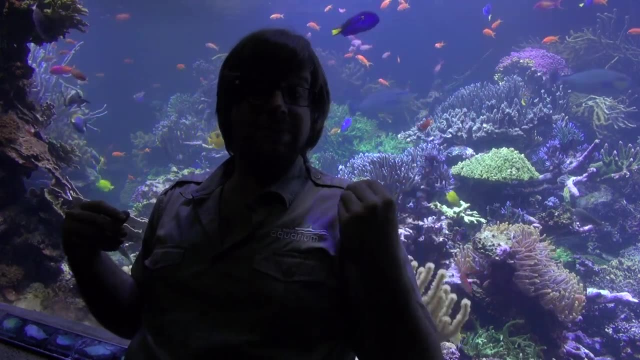 and they'll be able to take in those phytoplankton. Now, as Joe mentioned, and as we saw actually earlier, the soft corals are able to defend themselves from predators such as fish by retracting almost immediately, which is pretty cool right. 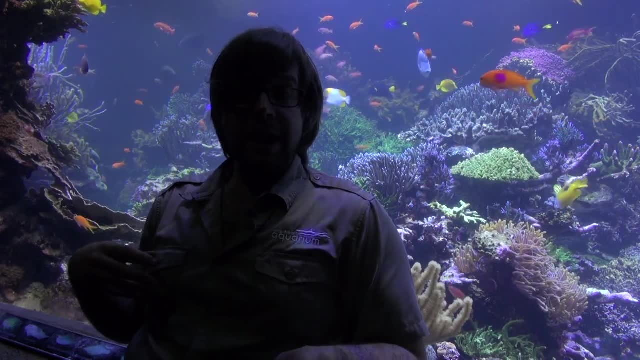 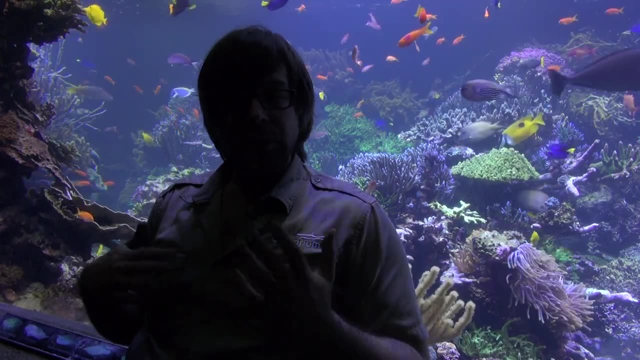 They also tend to have less of those zooxanthellae that Joe mentioned And when it comes to zooxanthellae, they tend to be very highly concentrated in those hard corals And zooxanthellae when we're talking about them. 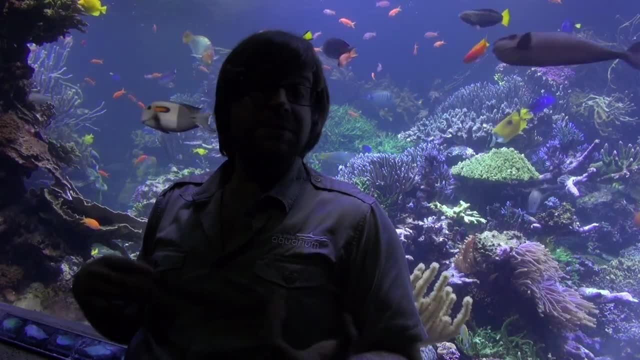 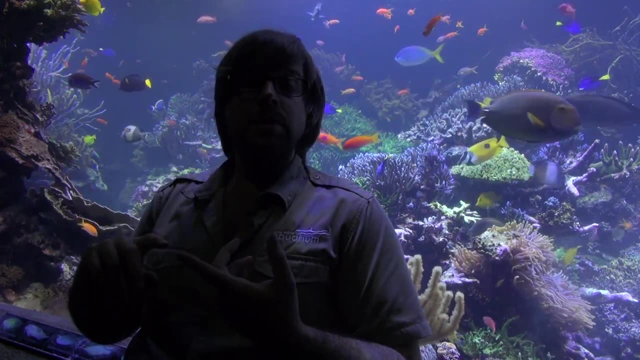 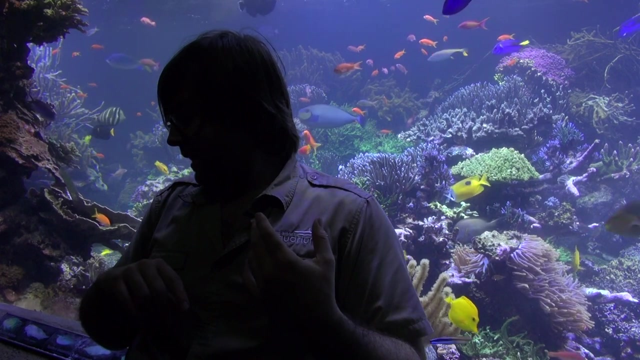 they're actually dinoflagellates, so single-celled protozoans, And they also are photosynthetic, So they have pigment molecules inside of them, known as including things like chlorophyll A, chlorophyll C, pyridinin and diodiaxanthin. 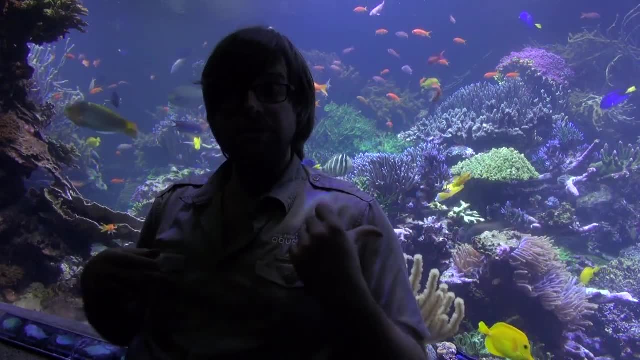 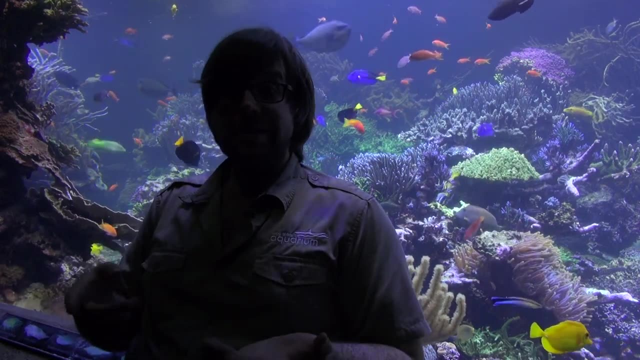 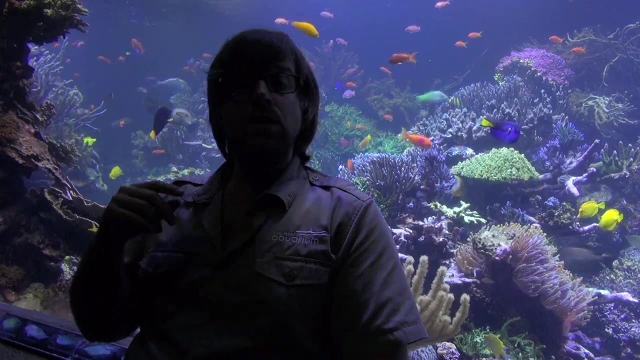 And so these pigments allow those dinoflagellates to produce food and other nutrients through photosynthesis, And so they're going to be giving things like oxygen and amino acids and glucose and glycerol to coral, whereas the coral will be giving them shelter and protection. 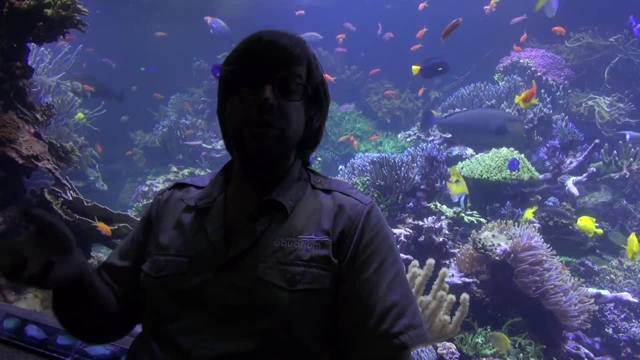 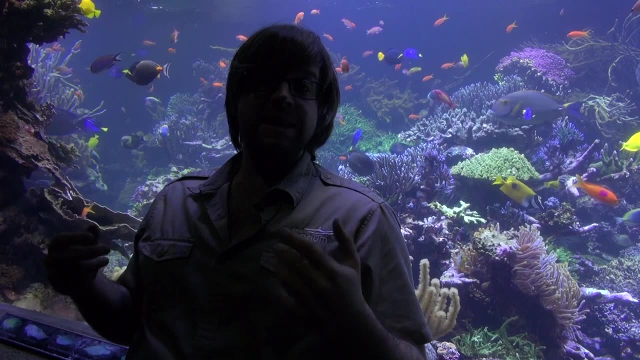 from herbivores and other things that may want to try to eat those dinoflagellates. And, by the way, the dinoflagellate that you find in most corals is known as symbiodinium, And you know we saw earlier as well. 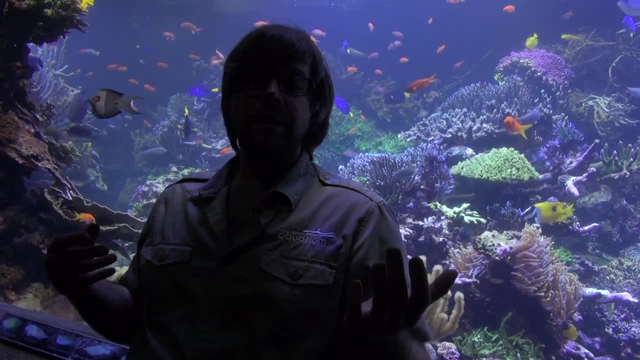 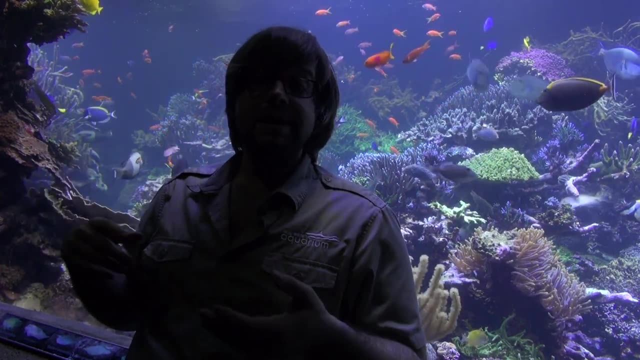 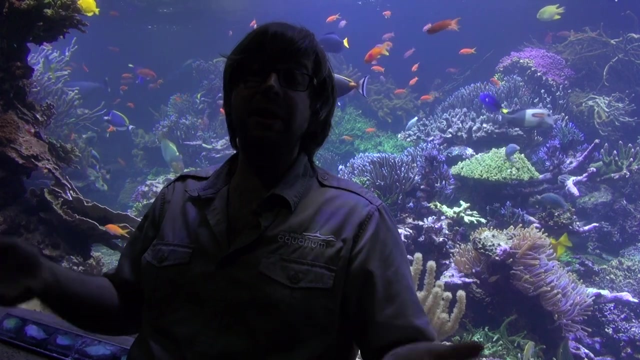 how calcium carbonate is essential, and the availability of carbonate, as well as calcium ions in oceanic water and seawater are necessary for corals, especially stony corals, to synthesize more skeleton and build upon themselves and essentially give structure to a reef. 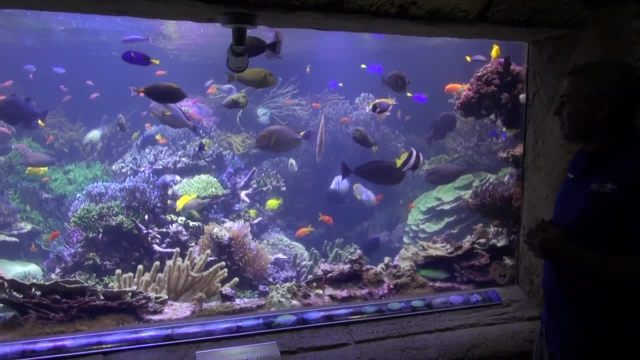 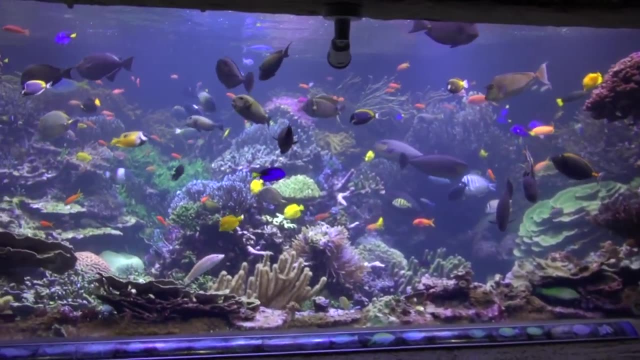 Corals are animals and they are laying down this calcium carbonate skeleton. This skeleton and the corals themselves provide structure. They provide the buildings, the buildings of the city, these reef cities. They provide shelter for the fish to sleep at night. 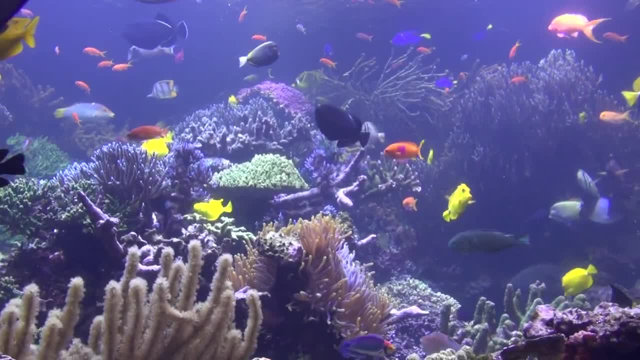 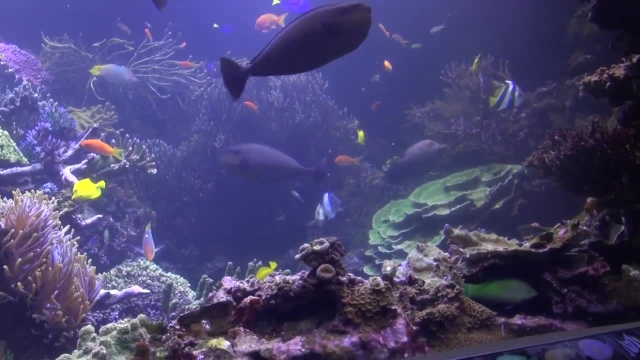 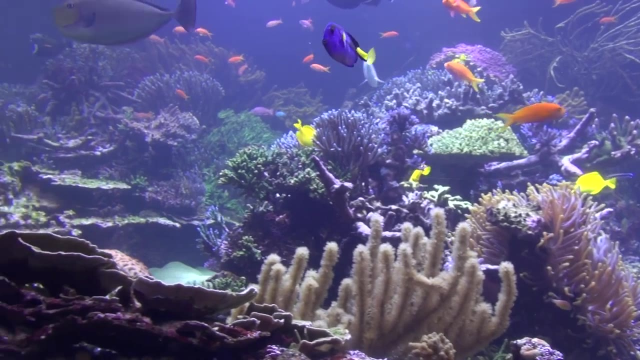 Some fish do eat the corals, But they provide the homes for this whole food chain because reefs grow in very nutrient-poor water where there really wouldn't be a lot of other animal activity if it wasn't for the reefs providing the base of the foundation of an entire food chain. 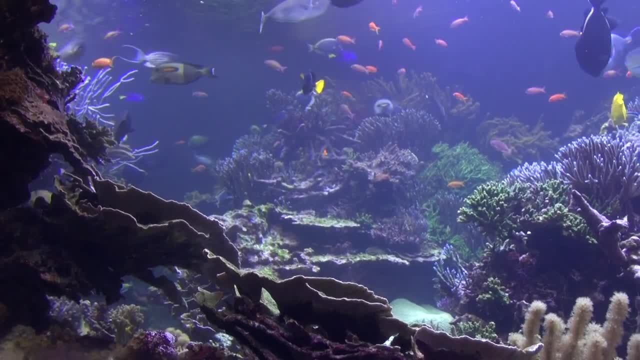 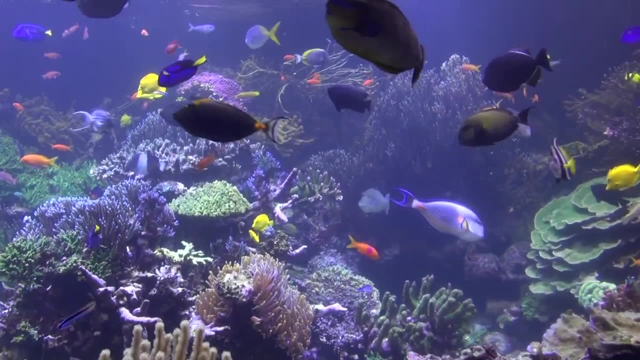 as compared to, say, like our local waters around Long Island, where we have a lot of nutrients and a lot of terrestrial runoff and a lot of algae growth and that's sustaining Reefs are growing basically in a desert of nutrients and they're generating that city. 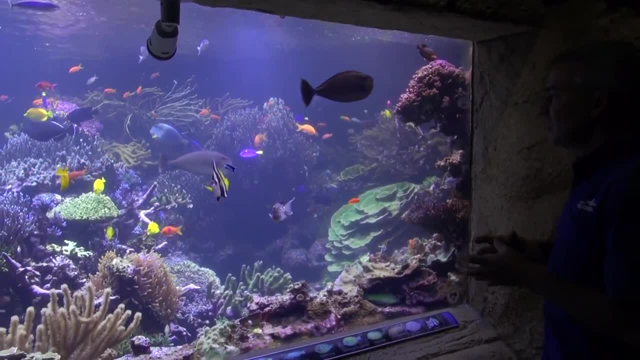 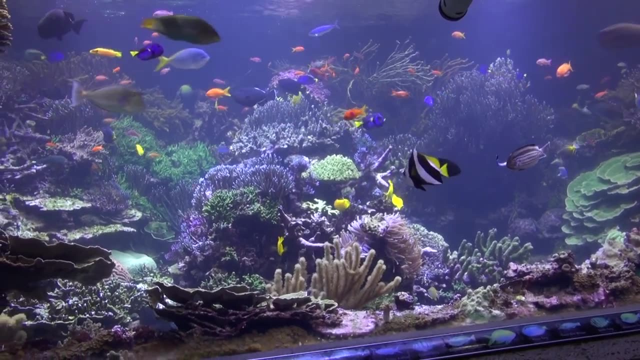 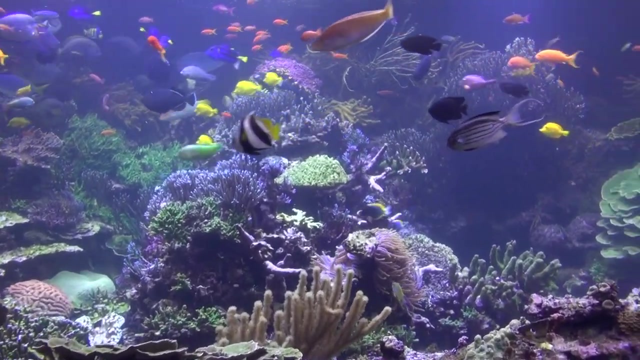 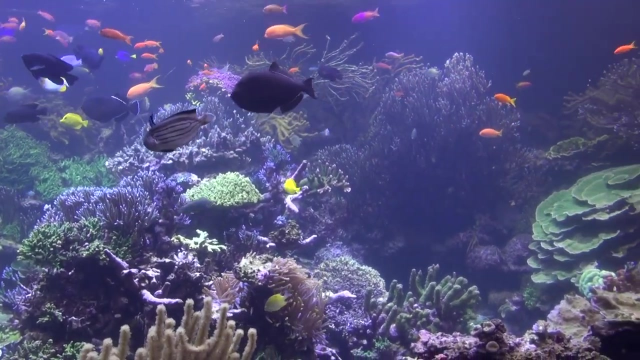 So, as they're laying down that calcium carbonate skeleton, they're providing the homes and structures for the entire food chain. They're providing a break from the wave action. So reef health is very important for the sustainability of the shoreline and the corals are going to be growing. 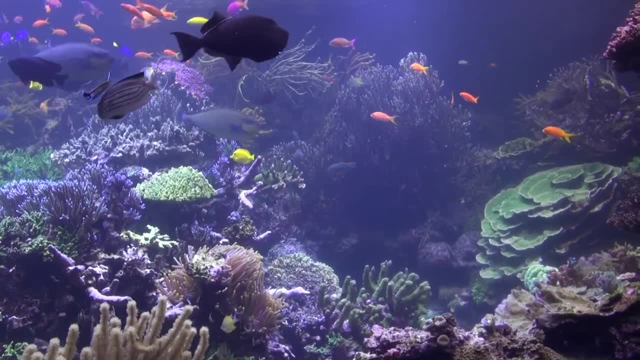 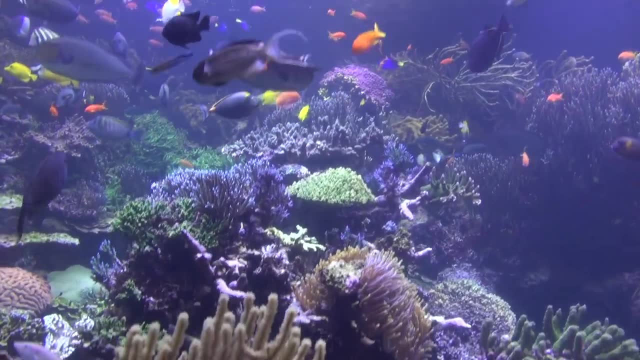 They want to get to the light. They want as much light as possible. So there's a lot of competition. So when you look at some of the corals in here, a lot of these have to be pruned on a regular basis. 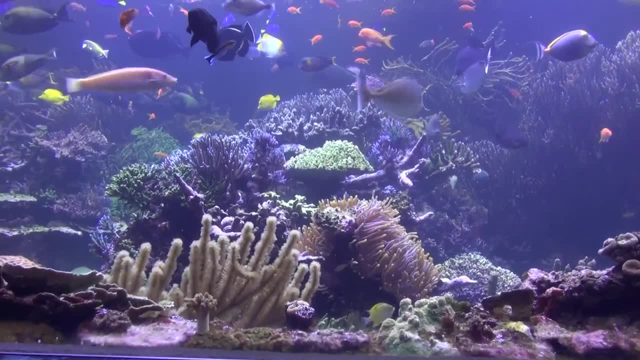 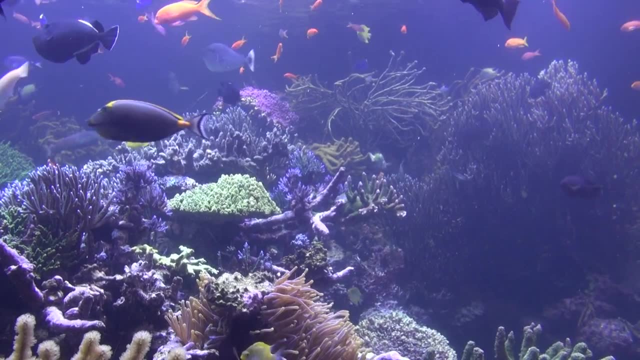 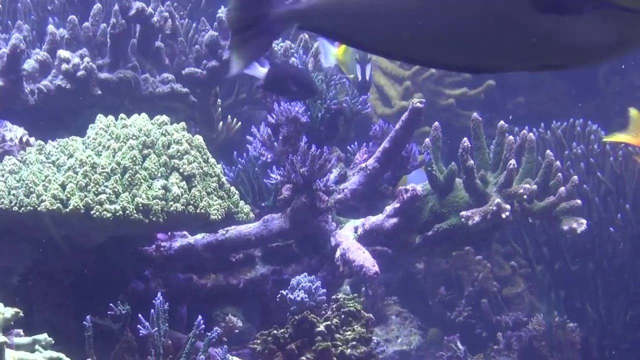 Certain corals are stronger. They have a stronger nematocyst, They have a stronger stinging cell and they will sting and kill their neighbors and then they have a nice clean dead calcium carbonate skeleton to then grow onto. So the competition for space on a reef is really intense. 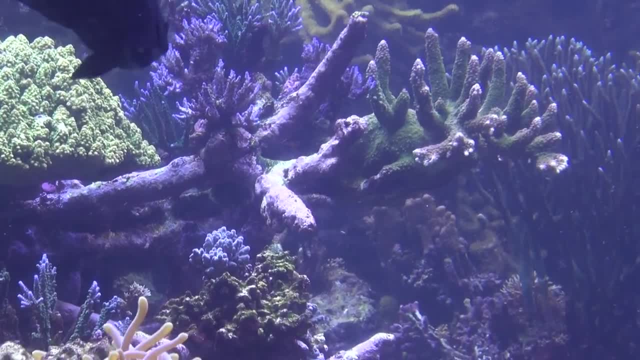 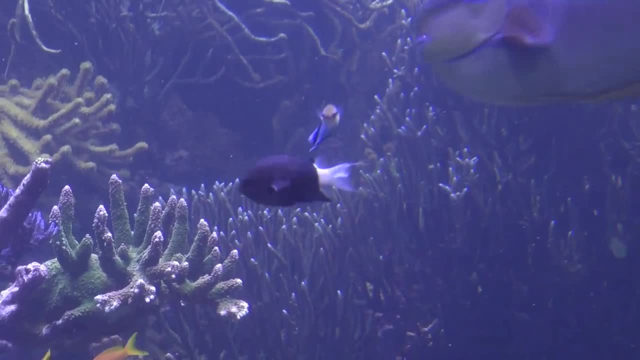 So this tank is pruned on a regular basis, because otherwise the dominant corals would then take over and you'd only end up with a couple of species of corals. So it's kind of like an old-growth forest- different things- where the dominant trees 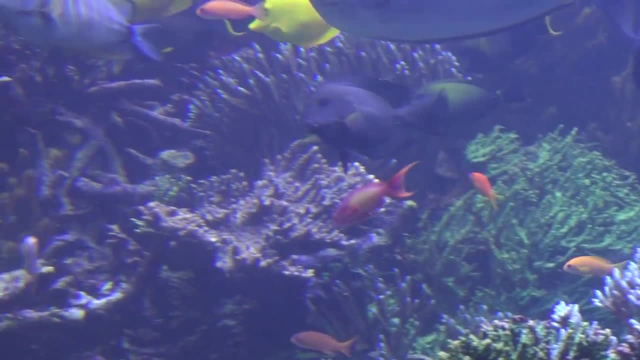 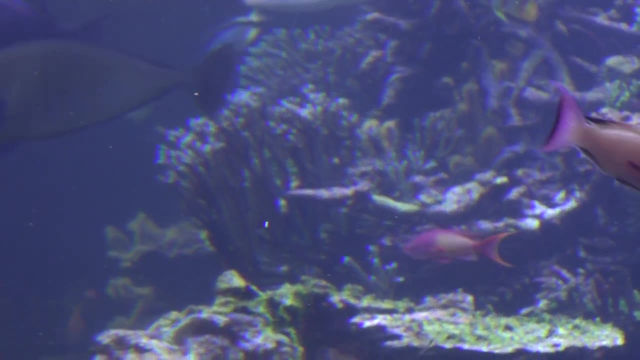 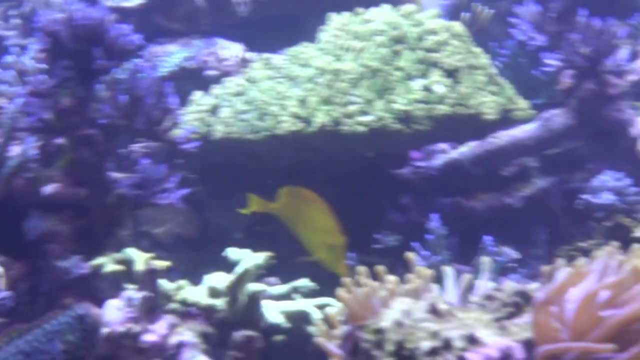 take over an entire section. A reef is very, very competitive and it's forever changing. They're secreting all kinds of toxic chemicals to kill their neighbors. They're sending out long, sweeper tentacles to kill their neighbors. Certain species of little palethoas here. 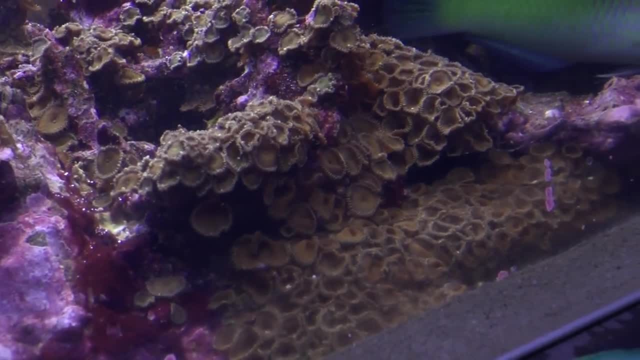 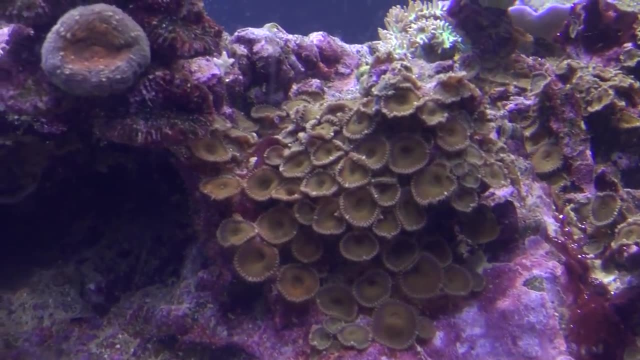 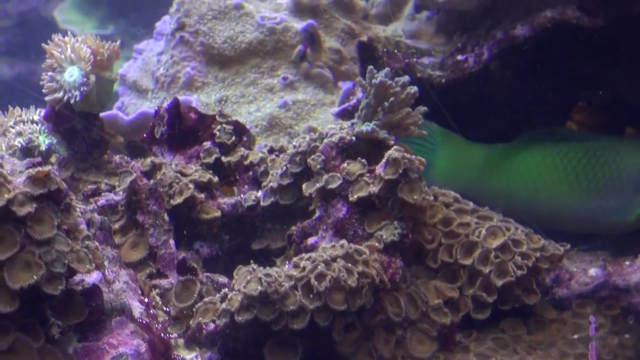 pretty much generate the most toxic substance of any animal on the planet. So one has to be very careful in handling any of the palethoas because they can easily affect a human, And so reefs look static to us, but they're constantly growing, constantly changing. 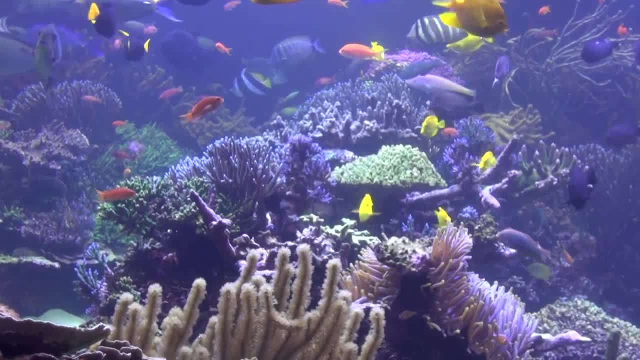 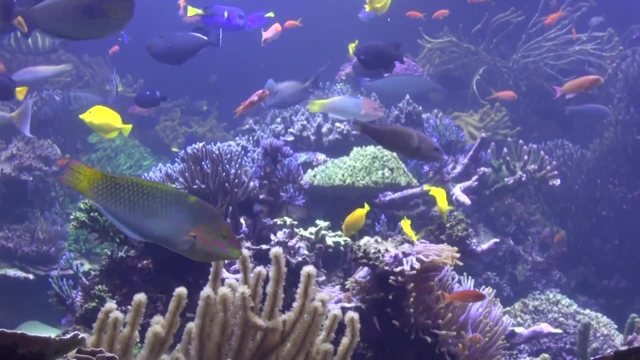 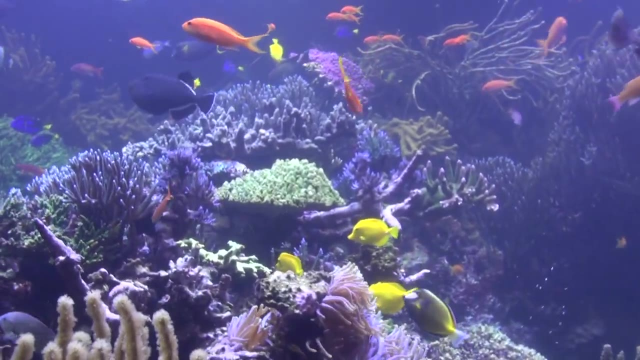 and it's a very dynamic environment. But basically a coral's goal in life is to- to put it bluntly, is to kill its neighbor, eat its neighbor and then grow on its denuded skeleton to then continue the growth of the reef structure. 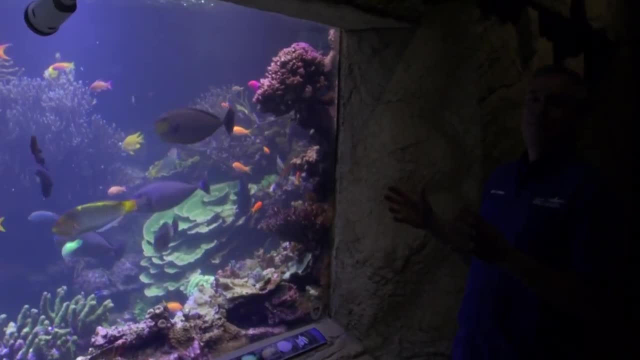 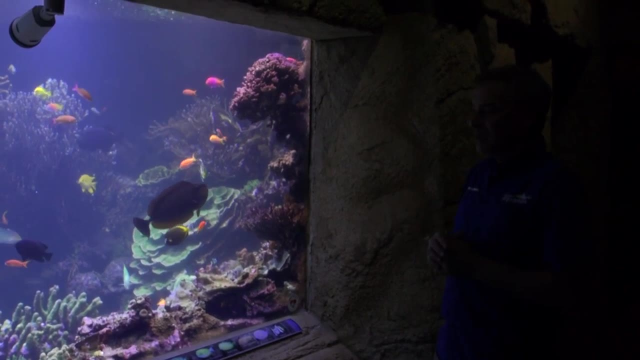 I know that sounds kind of harsh, a little bit cruel, but that's what's happening on a reef. There's just constant competition and a coral doesn't have to outright kill its neighbor. It can just overgrow its neighbor, It can overshadow its neighbor. 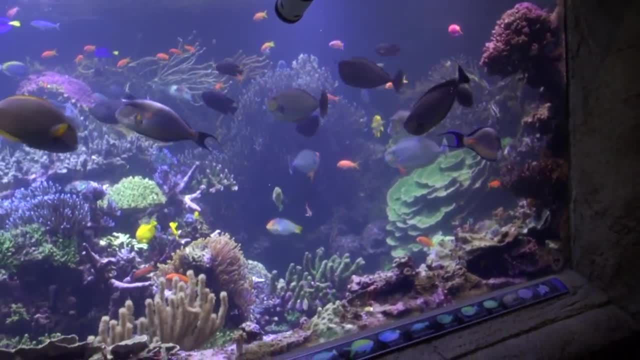 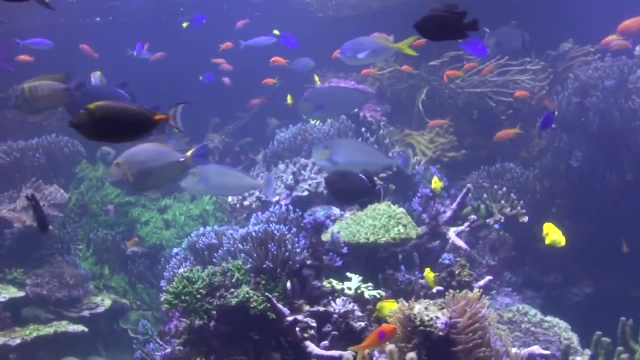 So again, they want corals want that sunlight to fuel their algae. So a coral doesn't have to physically sting and kill its neighbor, but plating corals, especially like the montepores and things that there's some competition in there. 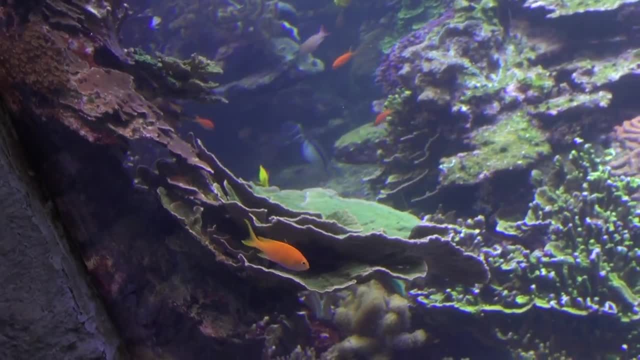 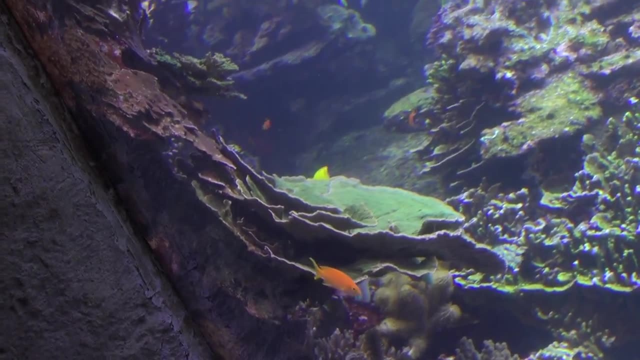 between a couple of species, but those plating corals there are just going to. if they just continue to grow out, they're going to overshadow anybody below them and then if you remove the light, that coral is going to die and then that secures the place. 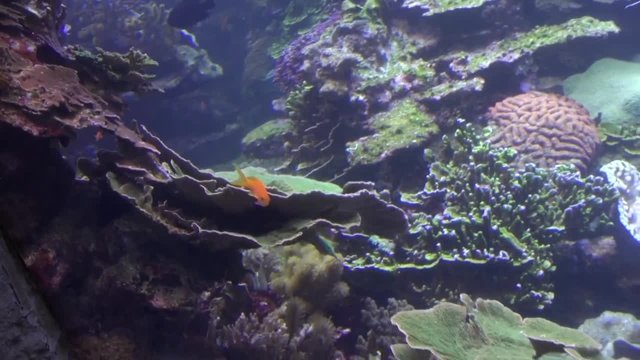 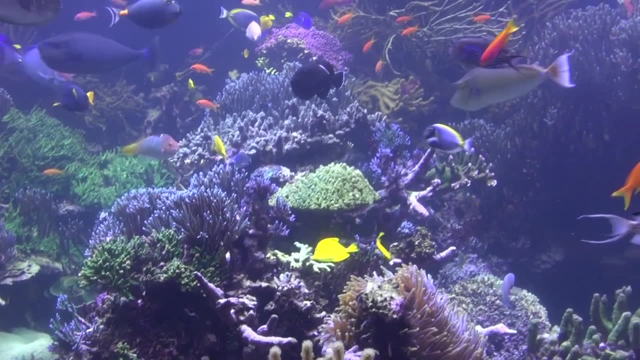 of that montepore, on that colony. So a lot of in this tank especially, a lot of pruning takes place to make sure corals aren't overshadowing and killing their neighbors as well, And in certain sections then we'll just give them the space. 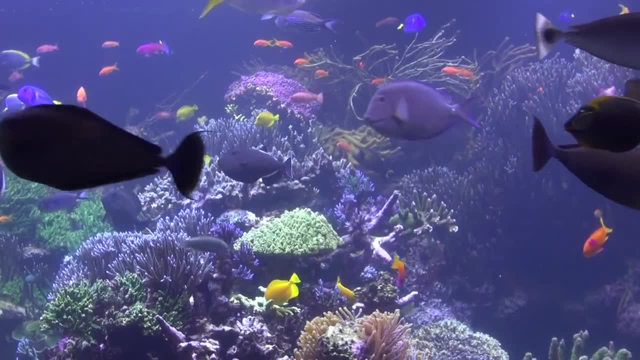 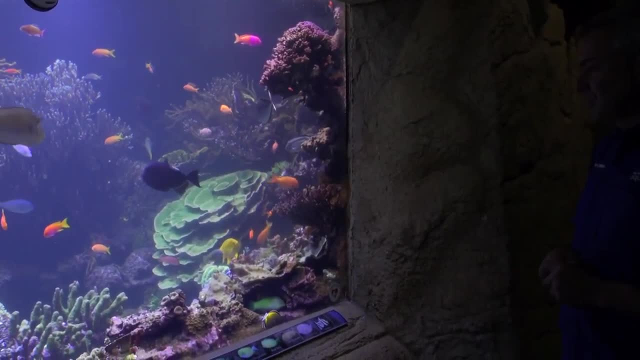 to grow to a very large size, so, depending on the spot, So it's just like a garden, but it's a garden of animals that needs to be pruned on a regular basis, just like a garden at your house. Reefs are so important to our oceans. They manage to touch so many different corners of oceanic ecosystems that without them, many creatures would find survival much more difficult. So take, for example, this giant Japanese spider crab which, to be honest, probably doesn't spend much time in coral reefs itself. 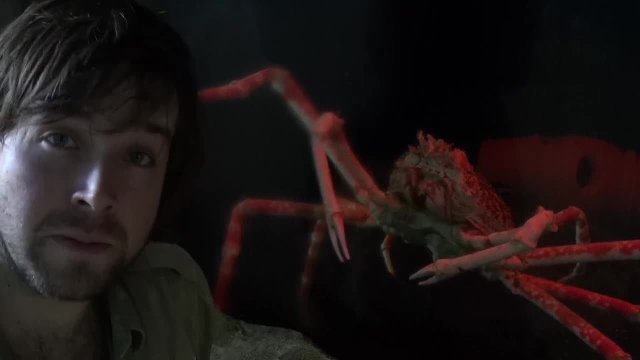 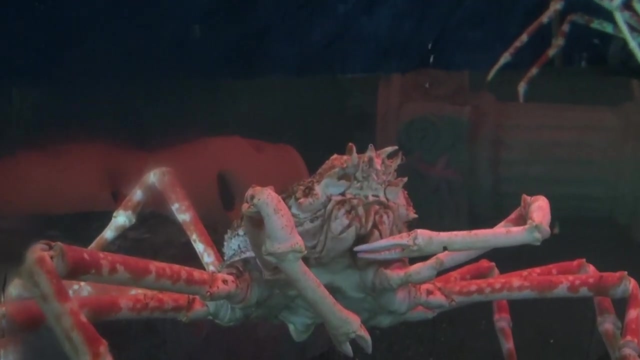 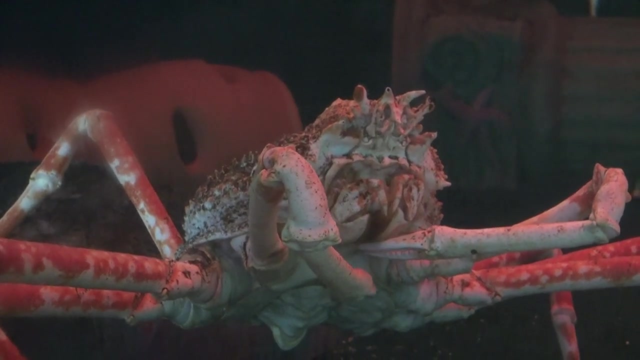 However, indirectly, reefs contribute to its survival. The giant Japanese spider crab is a huge crustacean. These guys can grow as big as 12 feet across in leg span, sometimes even larger than that. These guys come from the colder depths off the coast of Japan. and Southeast Asia And you know they'll spend their time like 1,000 feet down or so. So they're not really going to be a sight that you would see on the reef. They might not even be even kind of co-occur. where reefs exist. However, even these guys are indirectly affected by coral reefs. Giant Japanese spider crabs spend their days as omnivores. They're scavengers on the ocean depths- in the ocean depths rather- And they feed on little fish. or crabs or algae, things like that, But they'll also scavenge organic material that drifts to the bottom from the ocean surface, from the shallower depths. Coral reefs are so rich in life that they produce an abundant amount of organic material. that will inevitably wind up on the bottom of the ocean, allowing these crustaceans to exploit a valuable resource when prey might be scarce, Further their prey worms and other crabs and things will also rely on this organic material, this detritus. for survival. Without reefs, these guys might find it more difficult to find food. Well, let's take a look at some other crustaceans that rely a little bit more directly on reefs. These guys are known as sexy shrimp, which is a pretty funny name. 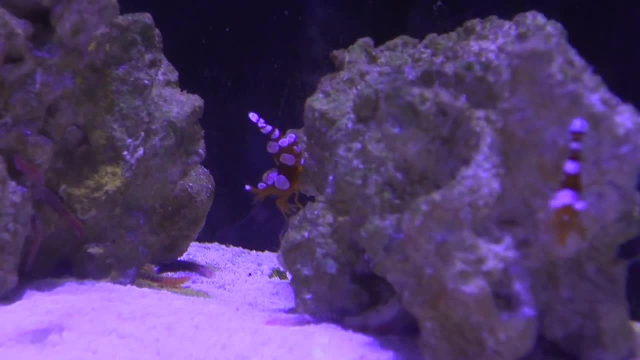 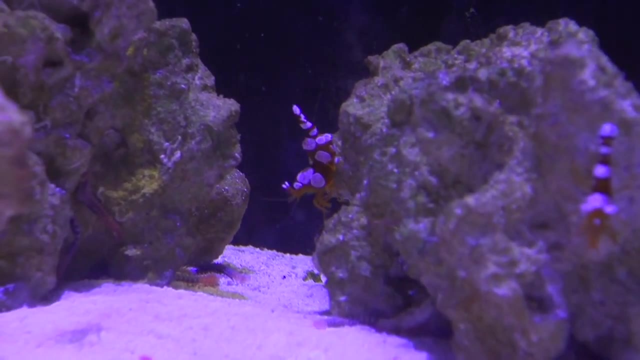 And this actually comes from the way that these guys wave their abdomens around rather provocatively, like this one's doing right now. But they come from Southeast Asia and they're a common site on reefs. They're actually a symbiotic organism with things like sea anemones. 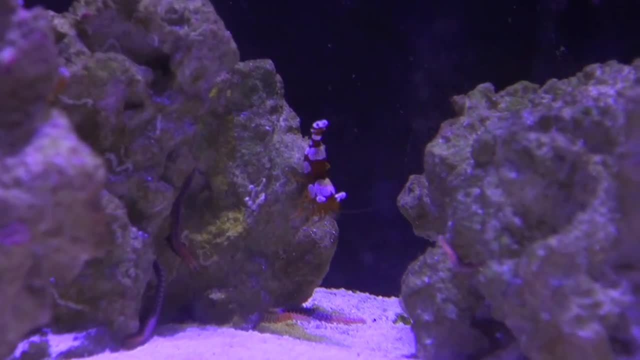 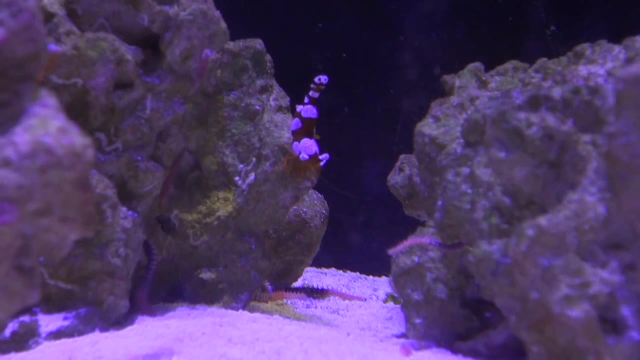 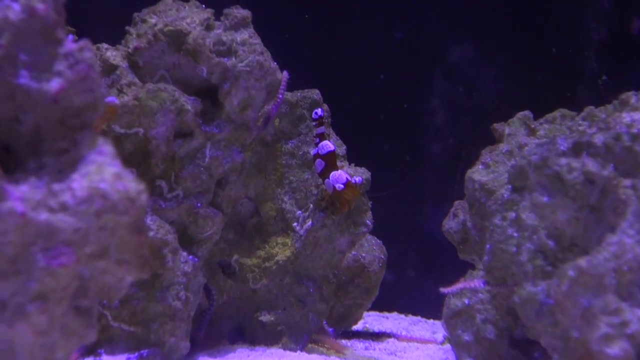 in which they'll live on the sea anemones within their tentacles and they feed on the mucus produced by the anemone, which apparently builds up, and this can help prevent the anemones from getting disease or other parasites. 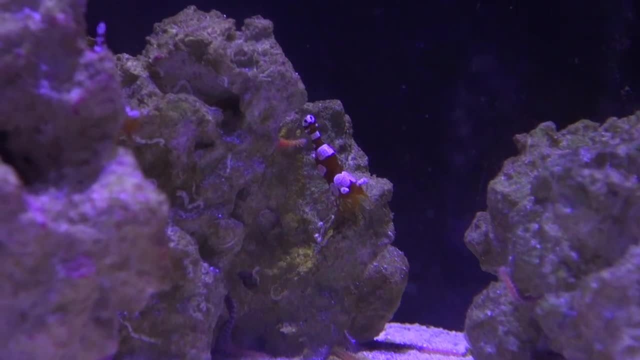 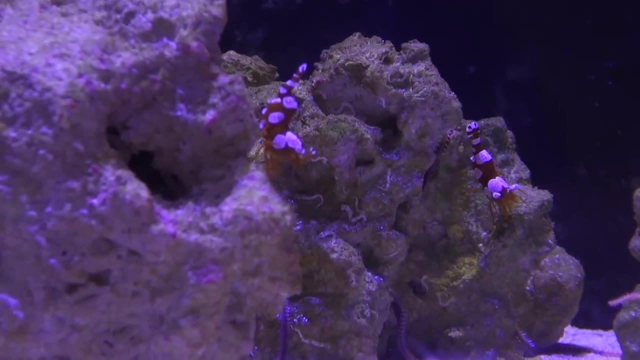 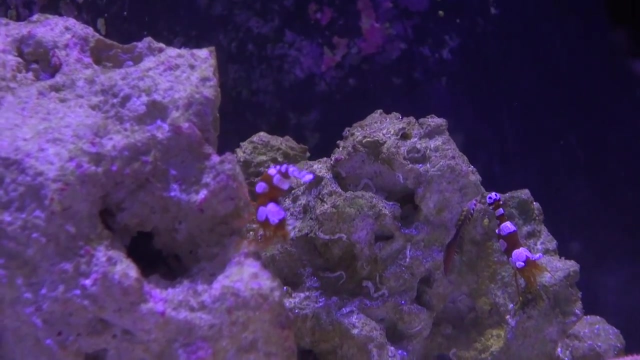 And the anemone serves to protect the sexy shrimp. This symbiotic relationship is fairly common among reef organisms, And crustaceans are very often going to be cleaners, since these guys like to pick off a lot of the things that will attach themselves. 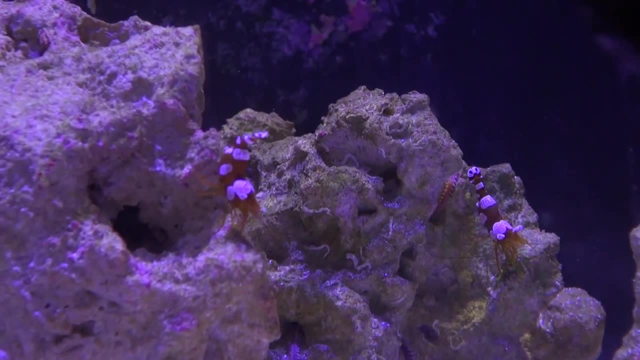 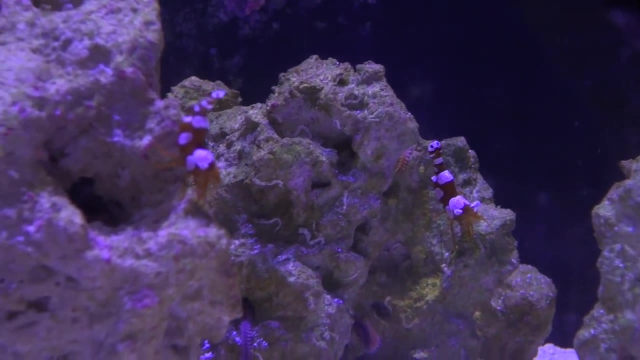 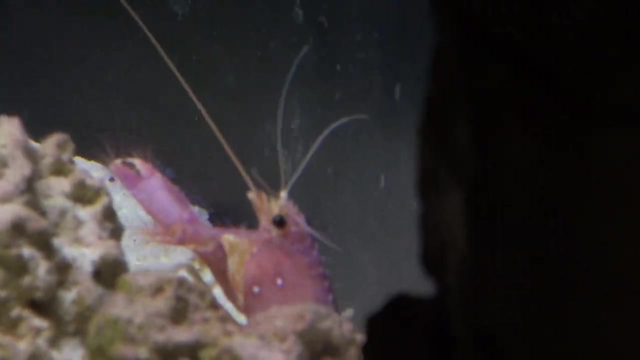 to fish and other marine organisms. You can even see there's a bunch of worms crawling around in the background there. Let's take a look at another crustacean. This guy is known as a reef lobster. Reef lobsters find their home on coral reefs. They come from Southeast Asia, as well as some parts of the Caribbean and the Atlantic, And reef lobsters form burrows within crevices within reefs, and they're basically detritivores and scavengers, essentially looking for grabbing food. that falls near their burrows and they just sort of go out and grab it and they bring it in and eat it. Without reefs, obligate organisms like the reef lobster here, who rely on reefs for habitat, would not be able to survive. 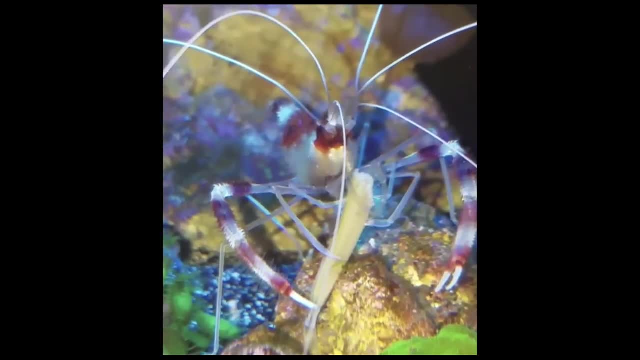 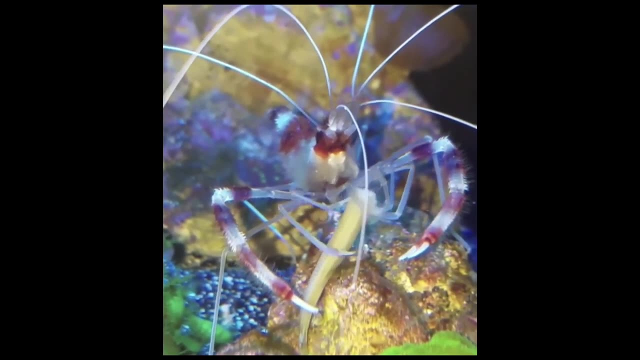 So here we have another crustacean that can be found on the reefs of the Indo-Pacific as well as Caribbean. This is known as the banded coral shrimp, and you can see them here enjoying a little sand eel highlighting one of their roles. 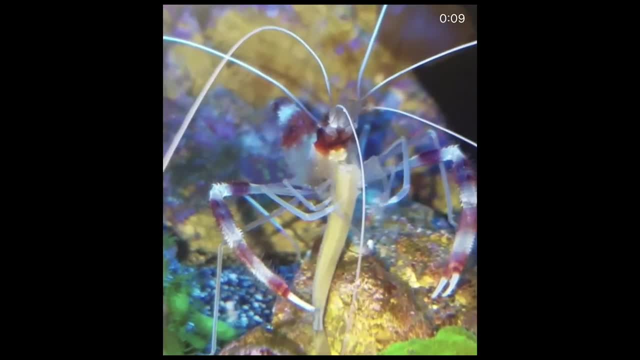 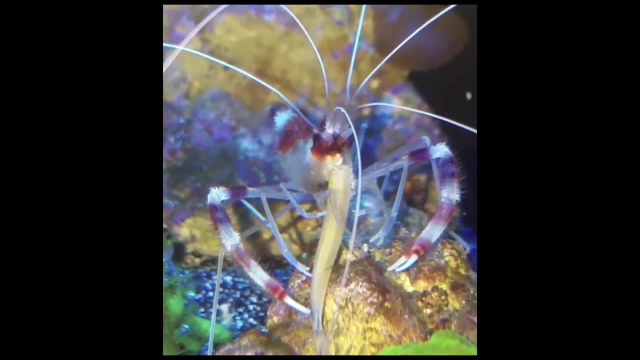 on the reef as a scavenger. However, they're not just scavengers. They'll also feed on little marine invertebrates and, in particular, they'll feed on the parasites of other marine animals, And so these guys will live in the cracks and crevices. 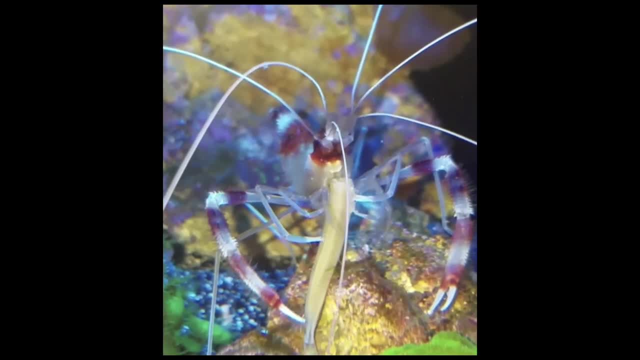 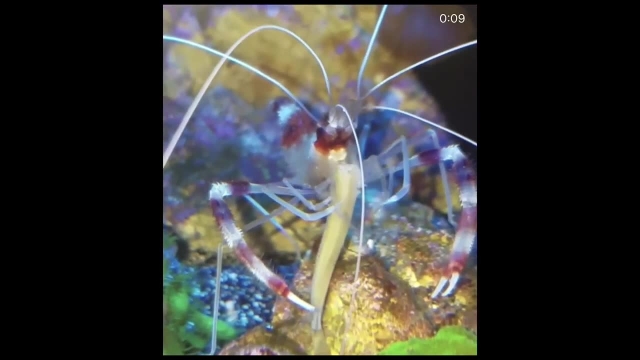 of the reef, kind of like the reef lobster, and they will come to the opening of their little burrow and they'll wave their antenna around and fish and other passersby will take note of this and go over to the shrimp so that their mouths and gills 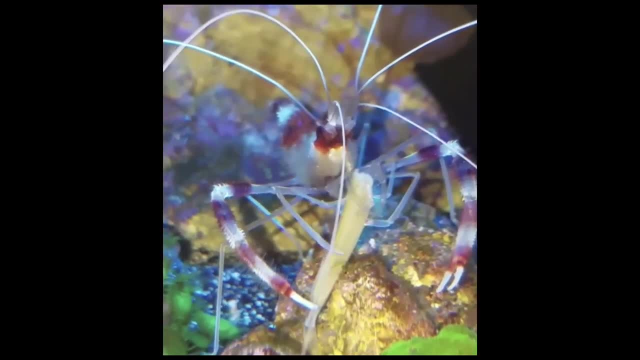 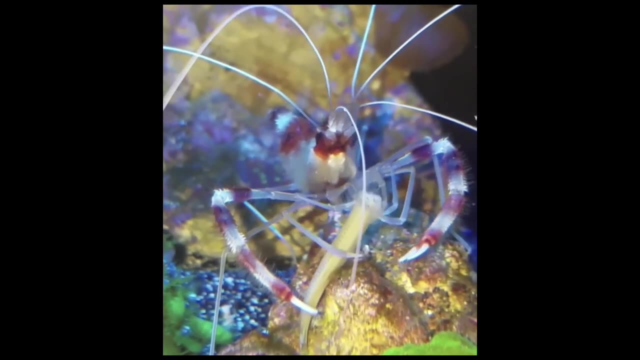 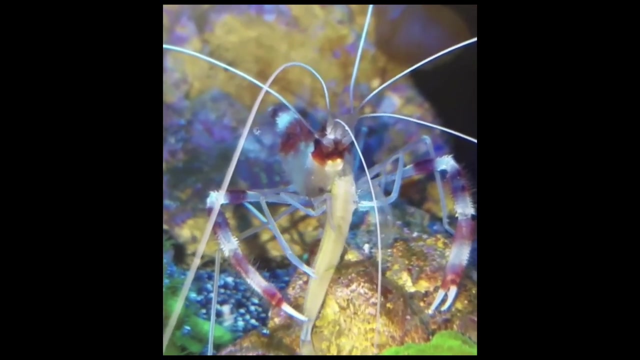 can be picked clean of parasites, And in so doing, this symbiotic crustacean helps to play a cleaner role in the reef ecosystem. Now let's go over to Joe for some other invertebrates that we might find on the reef. 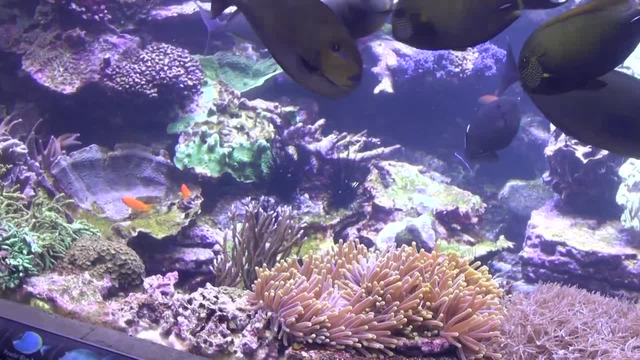 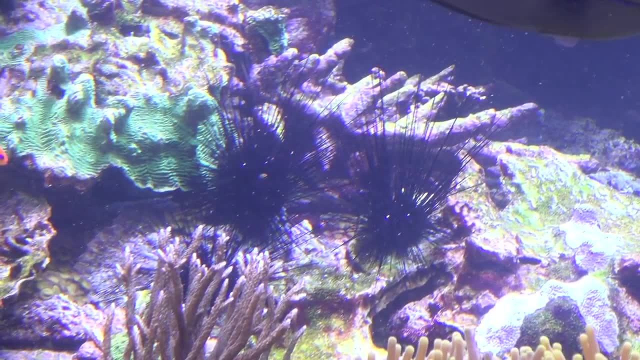 The reef. while it provides homes for a huge amount of crustaceans, it also provides a home for countless, countless other animals. So reefs are really the underwater rainforests where they're. just the biodiversity is mind-boggling and looking right now. 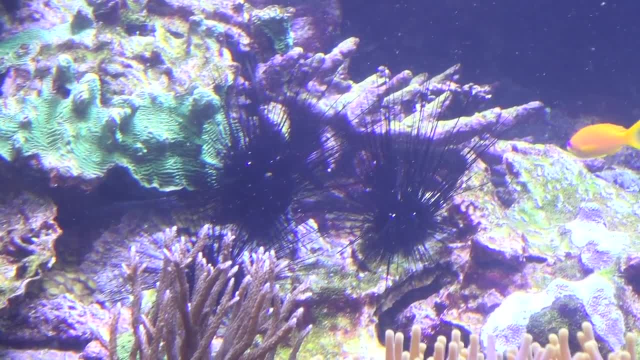 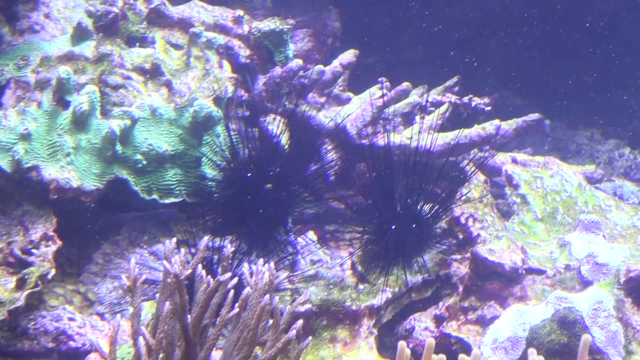 at some long-spine sea urchins here. These guys are invaluable to the reefs. They are algae grazers. Of course, the reefs are located where there's a lot of light, A lot of macroalgaes can grow, and if the system is thrown out of balance, 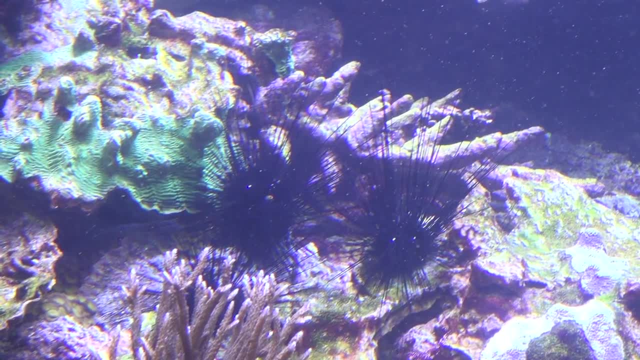 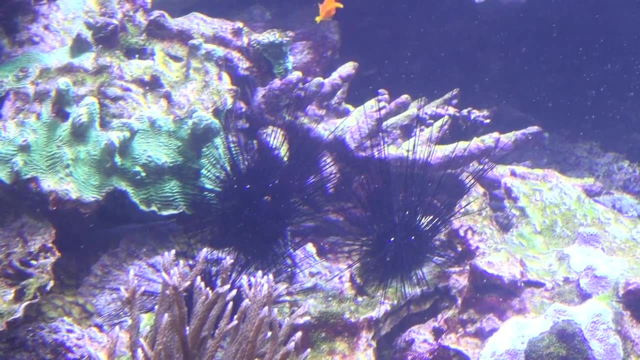 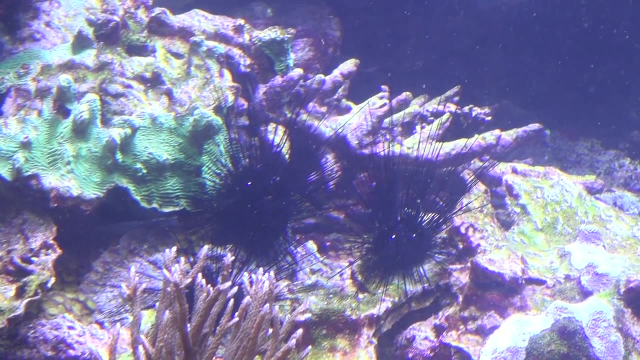 these macroalgaes can actually overwhelm and take over a reef, So these herbivores are crucial in maintaining the macroalgae, keeping it short and cropped. It's one of the main reasons a lot of the Caribbean reefs and Florida reefs have been seeing so much trouble. 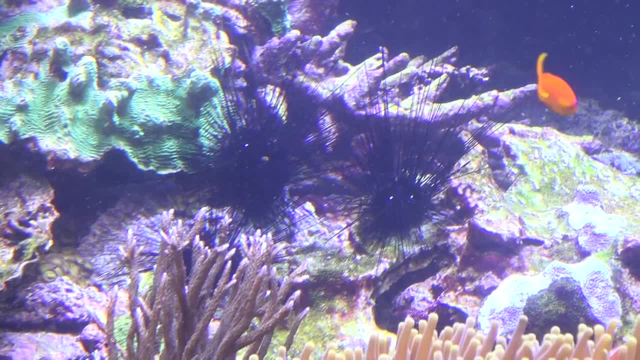 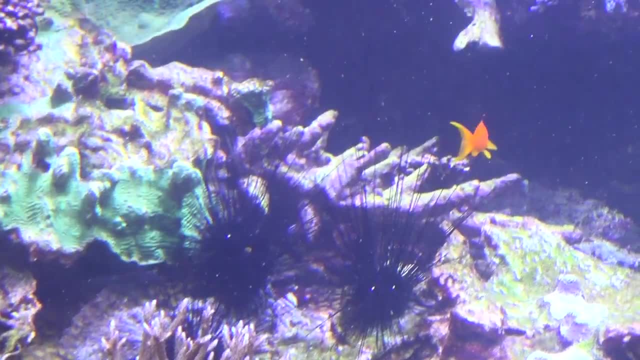 One of the main reasons is they had a huge die-off of the sea urchins and then that allowed a lot of macroalgaes to grow, So you have all kinds of different types of sea urchins. These are some long-spine sea urchins. 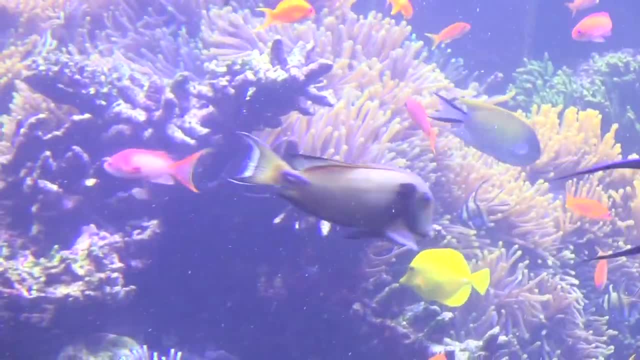 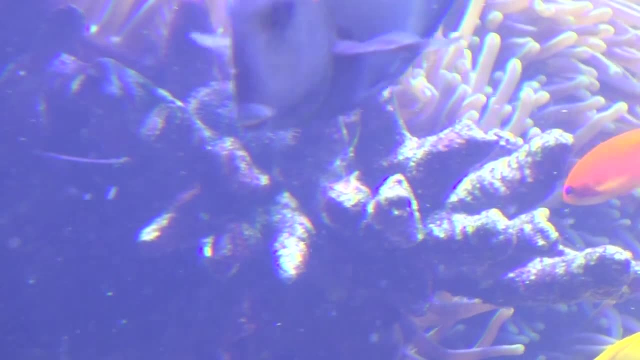 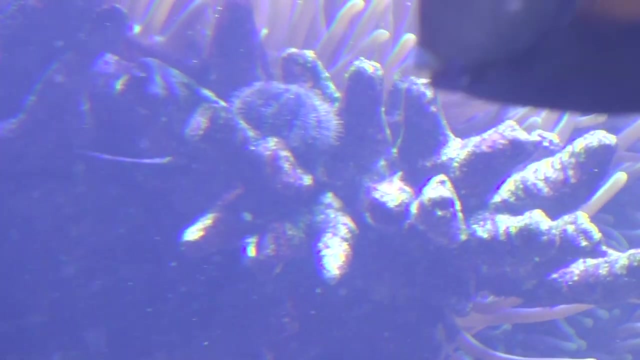 Up higher. we have this little short-spined urchin kind of hanging in the reef structure there. So our urchins are relatives to sea stars, So they've got this grazing mouth that they're just going around and constantly just grazing the reef structure. 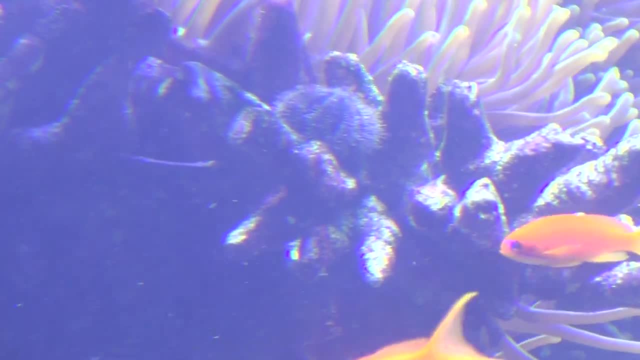 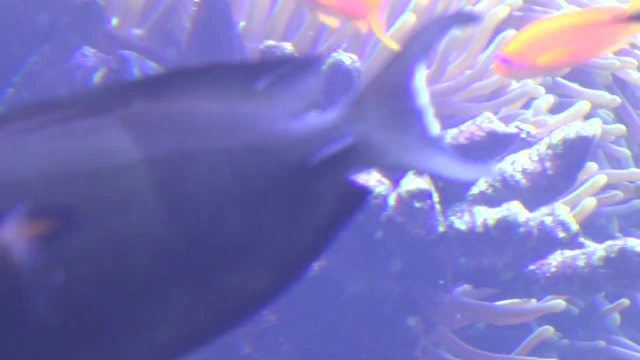 And again, keeping that structure really crisp and clean allows for new recruits and for new corals to settle out as well. But again, the diversity of life on a reef is mind-boggling. There's all kinds of mollusks. We have some giant clams here. 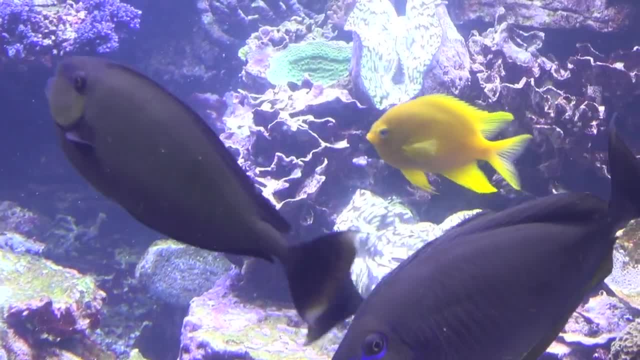 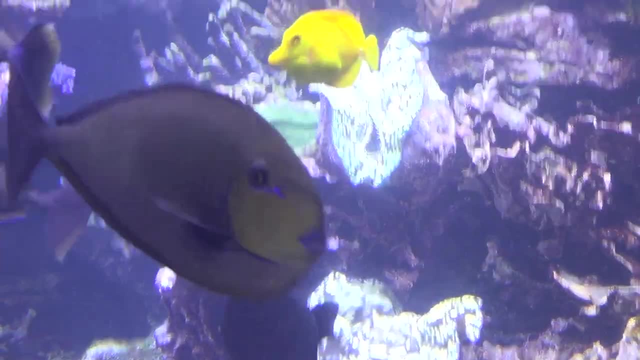 in the reef tank here. These are tridacna clams. Fish can be a bit pesky sometimes. They're looking at me for some food right now too, so we can maybe do a feed after this is said and done. 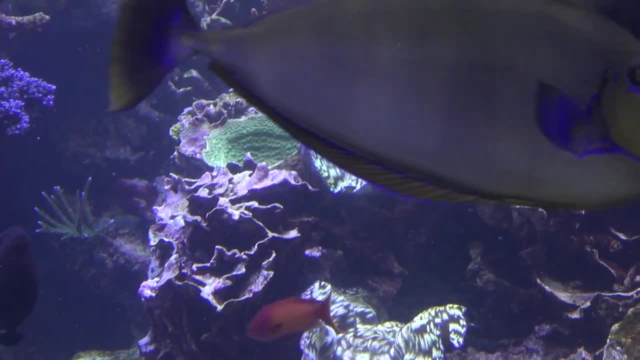 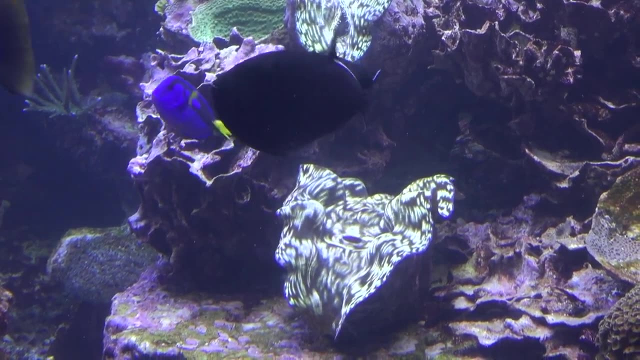 But you've got a number of different species of giant clams. These are tridacna duracea, The one up top- you can see the incurrent where they're pumping the water into their body. That's slit there- And actually the one on the bottom. 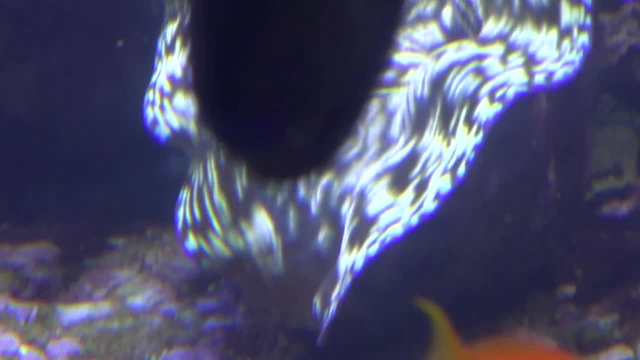 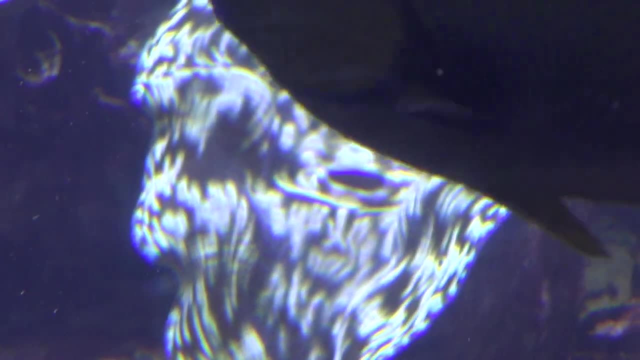 I have it reversed so you see that circular part and that's where the water is being pumped out. So these guys are constantly filtering a huge amount of water, But they also have- surprise, surprise, these guys also have zooxanthellae. 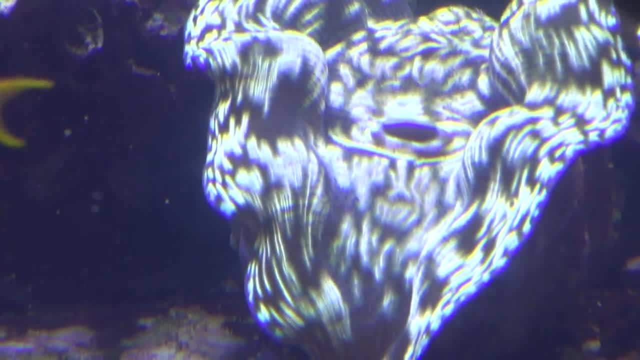 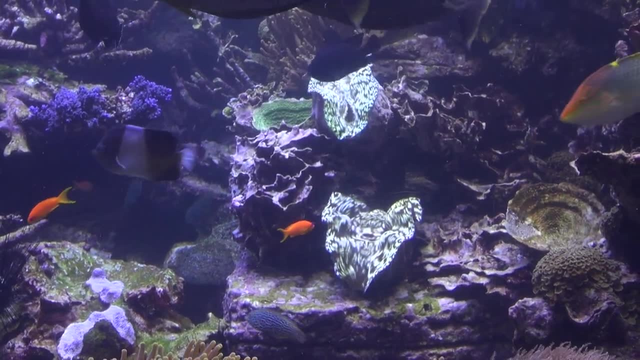 that algae in their tissue. So that's why these clams are opening up so much. They want to open that mantle up. get as much zooxanthellae exposed to the sunlight and they're gaining a lot of nutrition, lots of good energy and food. 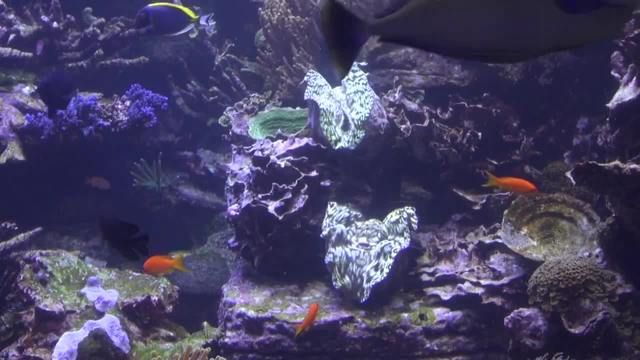 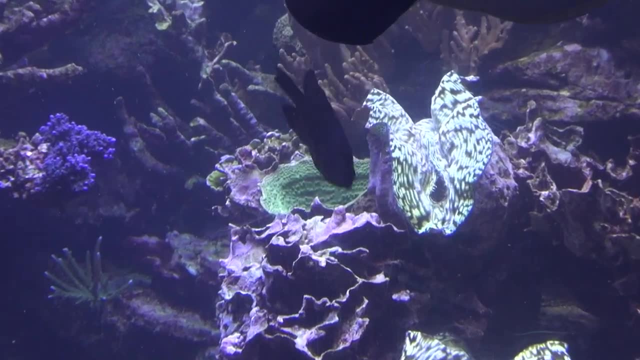 from the zooxanthellae in their tissue. These guys also have eye spots along the perimeter of their mantle. They don't see an image, but they can see shadow and light and sometimes you'll see these guys And they can retract. 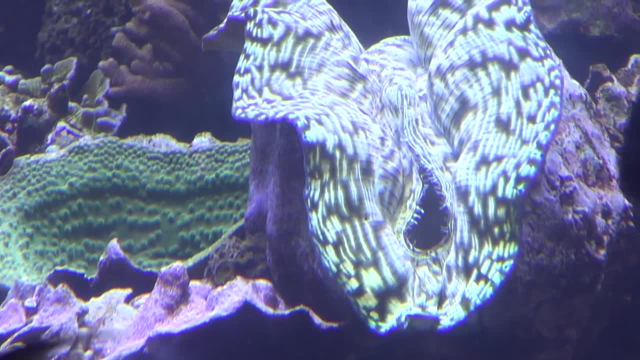 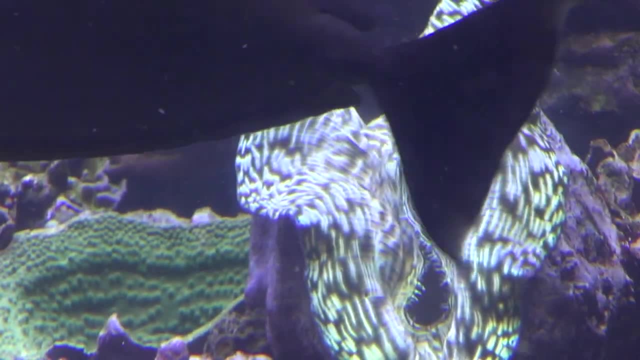 completely, completely within their shells and look more like a local clam. Right now, though, they're going to be opened up. They don't feel threatened, So that mantle is out to again get as much nutrients as possible. So, these clams- 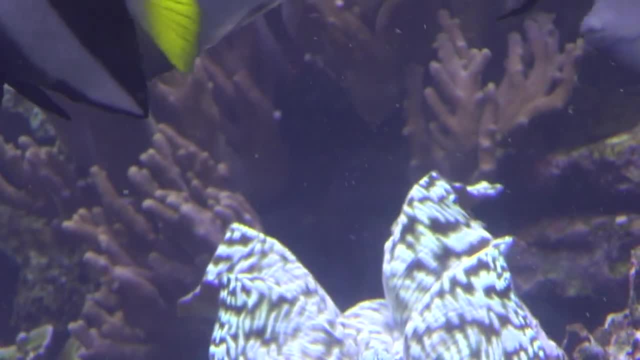 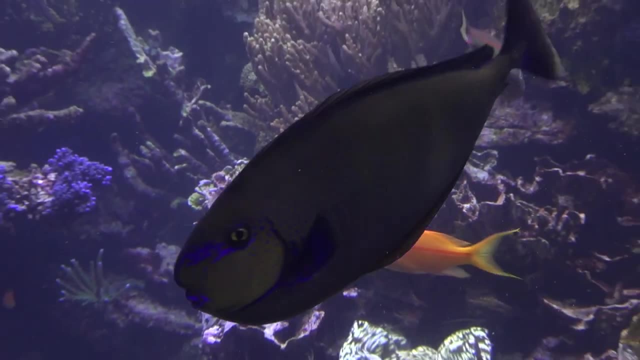 can get quite large and there's another species called Tridaconic Gygus that gets to, you know, over five feet across, and the old diet of these guys is that they're going to have these giant clams eating divers. 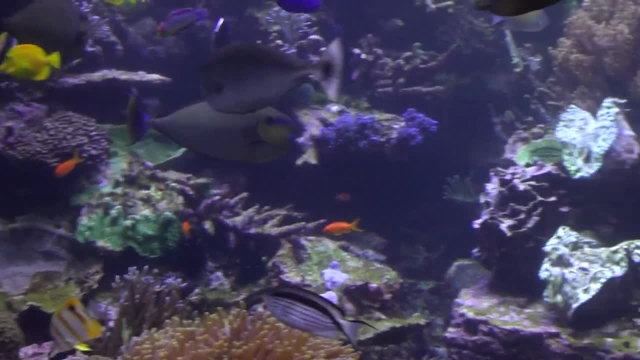 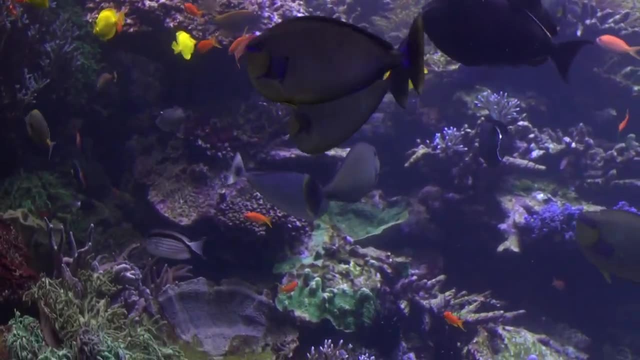 and they will not eat a diver. but if they, if you do happen to have your leg or an appendage in the region and they close up on it it's, they will hold on to you and you could drown. They're not eating you. 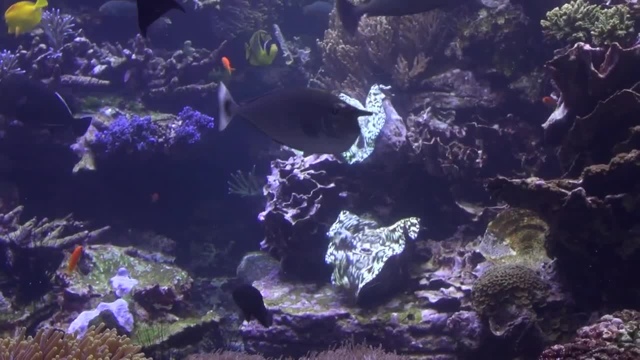 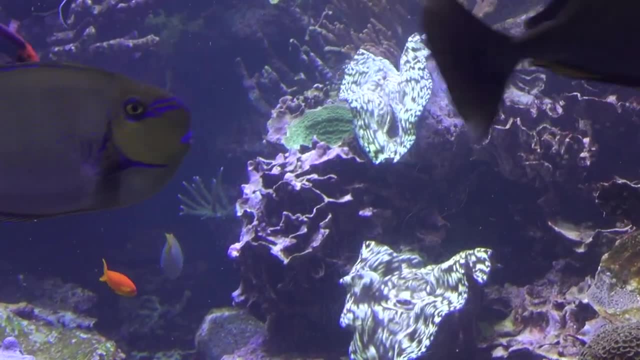 They're just trying to close. and if you get your arm or leg stuck in there and if it's a big enough, clam you, you are not getting out. So you know, it's, it's, it's, it's. 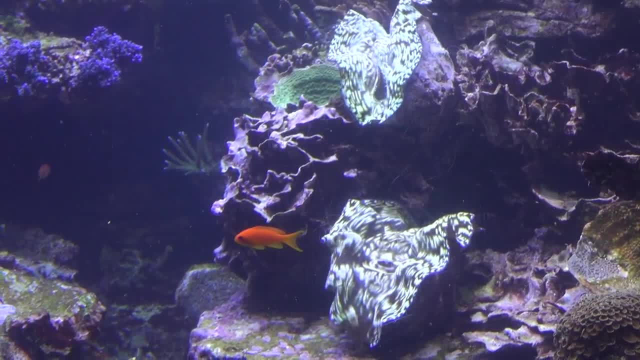 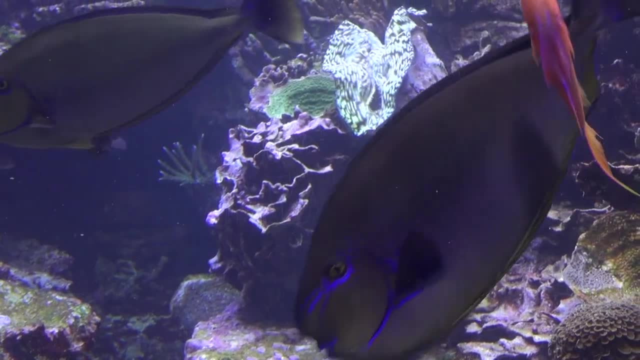 it's hard to find out. So, as with anything on a reef when you're diving, you just don't want to touch anything. That's that's the basic rule for your own well-being and and the reef's well-being as well. 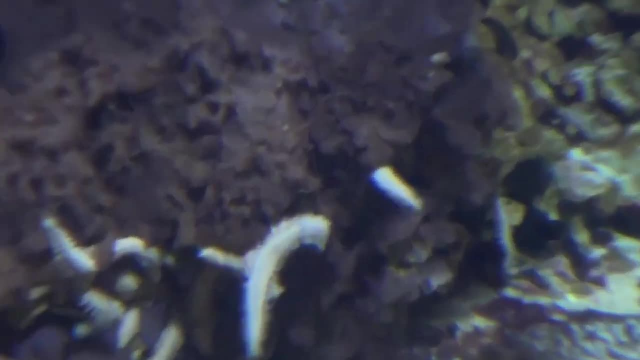 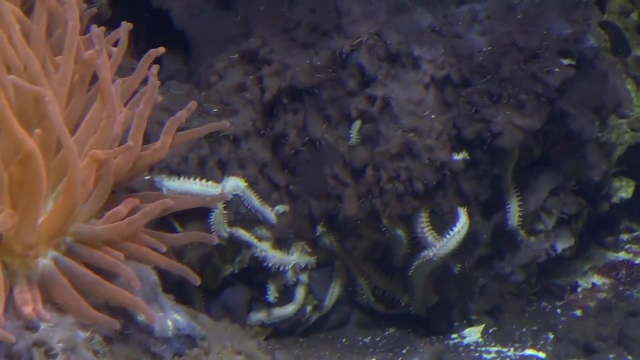 So not all of the creatures on a reef are flashy like the giant clam or the crustaceans that we saw earlier. Some of them are a little, I guess, a little more reserved in their coloration, like these bristle worms here. 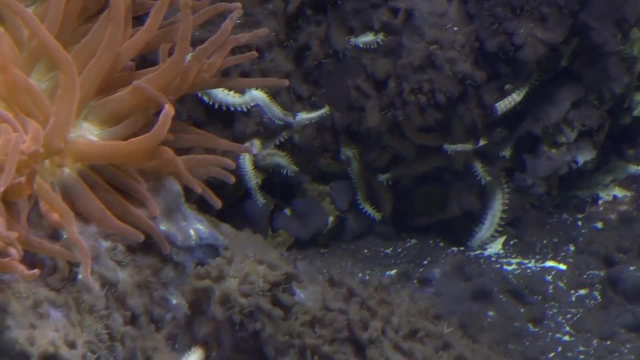 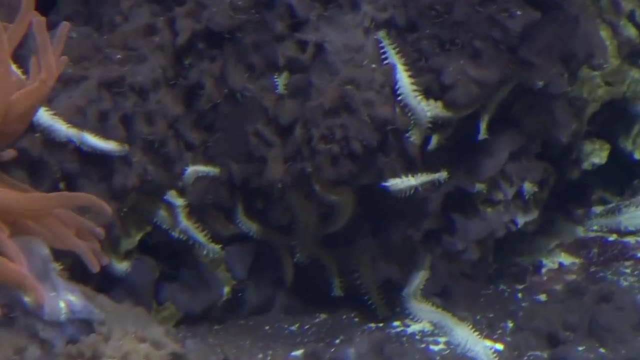 Now Joe has just fed some some frozen fish to this habitat and almost instantaneously, hundreds of these little bristle worms started to emerge from the rocks. and these guys are cleanup crew on a reef. So basically, they'll come out and they'll pick up. 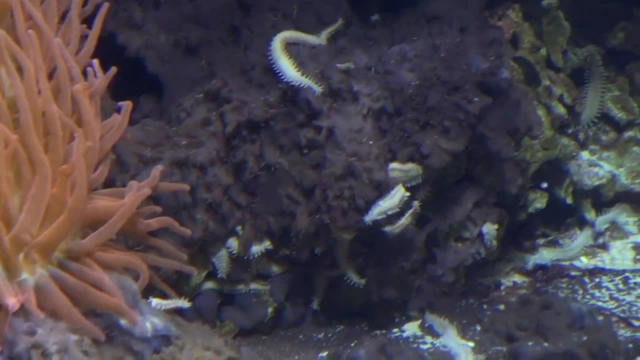 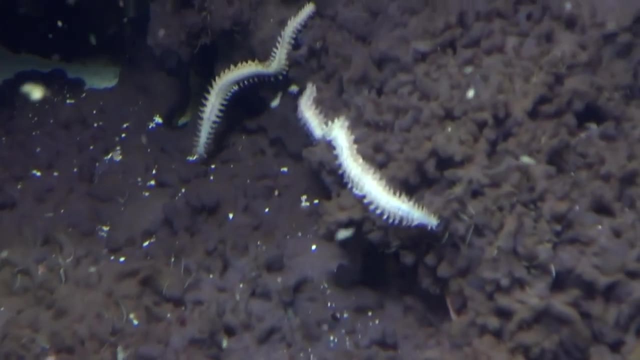 a lot of the decomposing organic material that floats to the bottom. These particular bristle worms don't have bright colors, but there are thousands of different species of bristle worms, or the so-called polychaete worms, that have all kinds of different lifestyles. 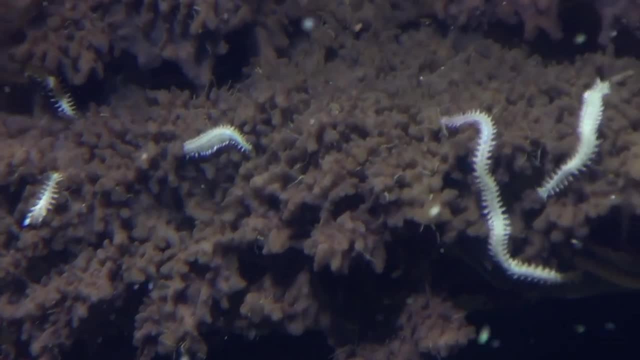 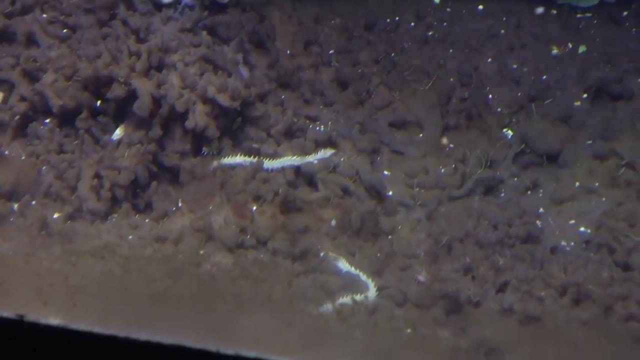 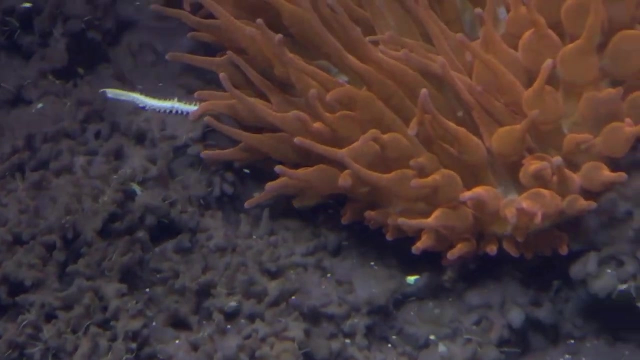 including predation herbivory, flashy colors, and there are also some gigantic ones out there as well, But these guys are pretty neat to see because you don't often see them in our aquarium habitats, unless feeding has taken place And you can see. 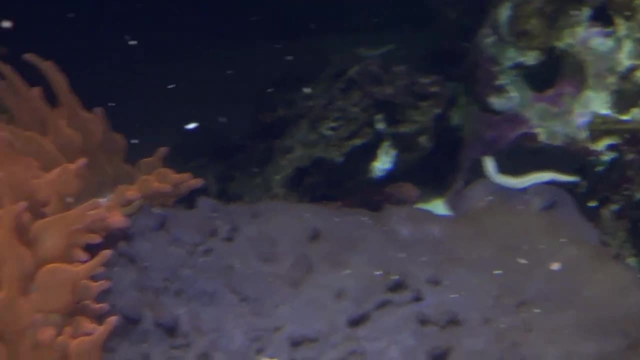 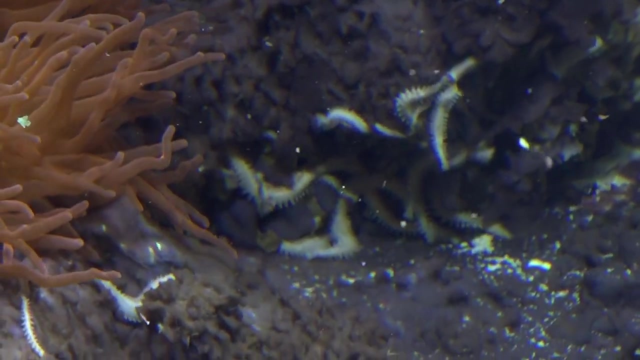 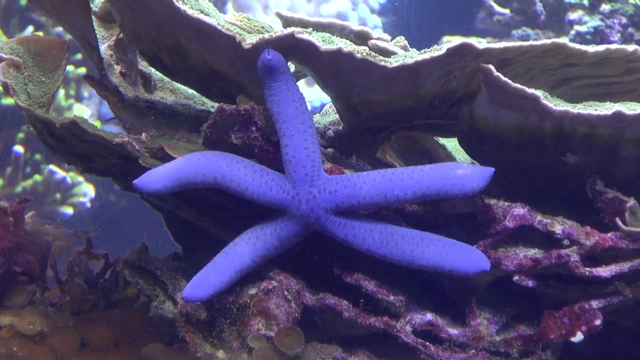 them retracting into the rocks. So they obviously play the same role on an actual reef ecosystem. But let's check out some of the other bottom dwellers that we might find on a reef Sea. stars, or echinoderms, are one of the. 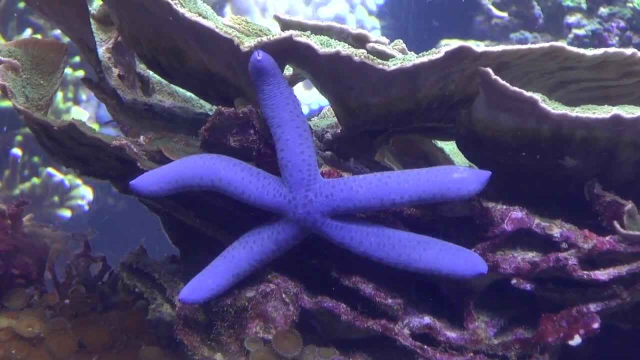 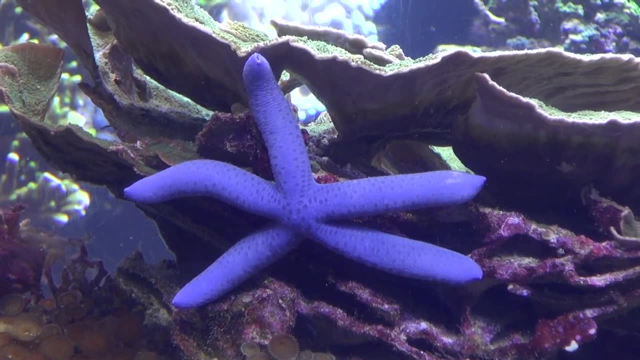 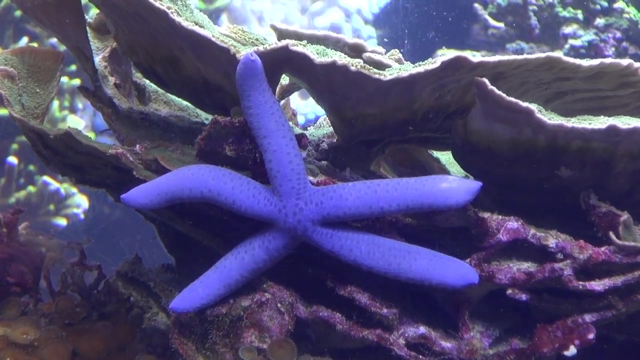 other major groups of invertebrates that you might find on a reef. So these guys are called echinoderms due to their skin. So echino refers to spiny and derm means skin, So these are little spiny. 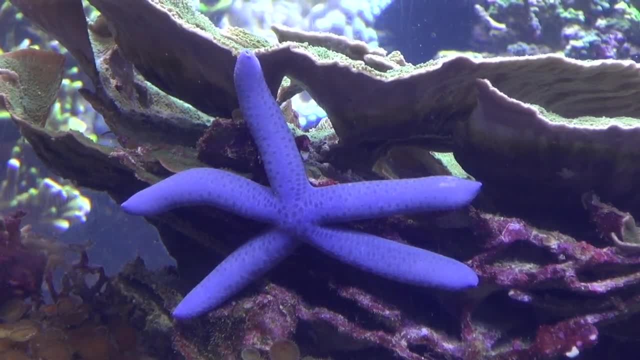 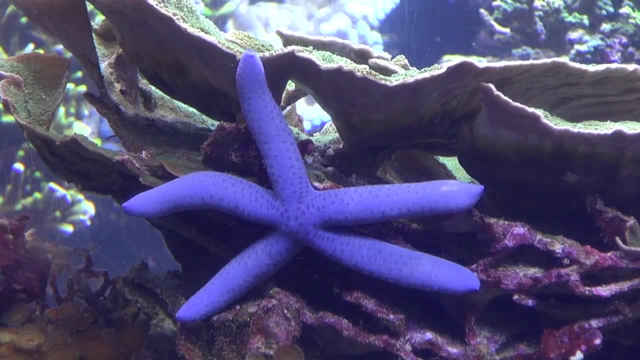 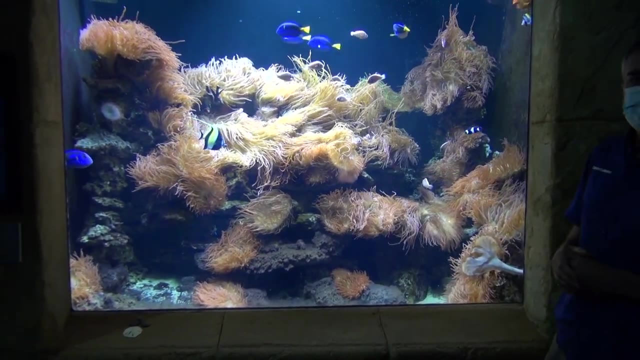 skin animals that you might find on other sea stars. And then many are also going to be feeding on scavenging whatever might fall to the bottom. But just another common creature that's reliant upon reefs for survival. All righty So. 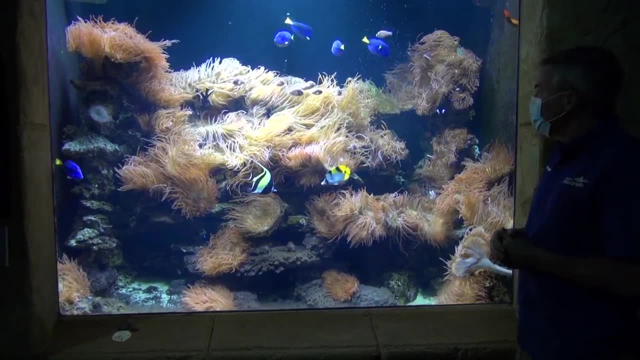 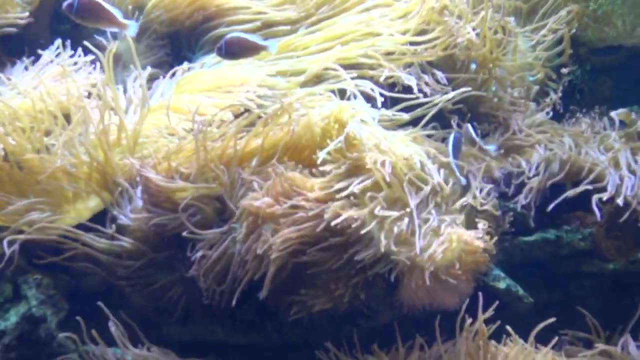 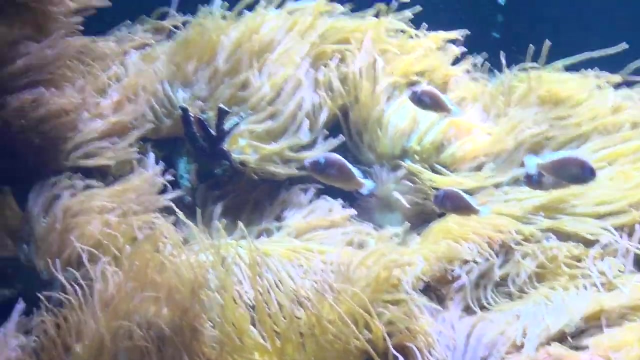 we're standing in front of our clownfish anatomy tank, our best buddy's habitat here. It's about 2,400 gallons. There's rose and the split-apart section can then move around, kind of crawl around almost like a kind of like a snail. 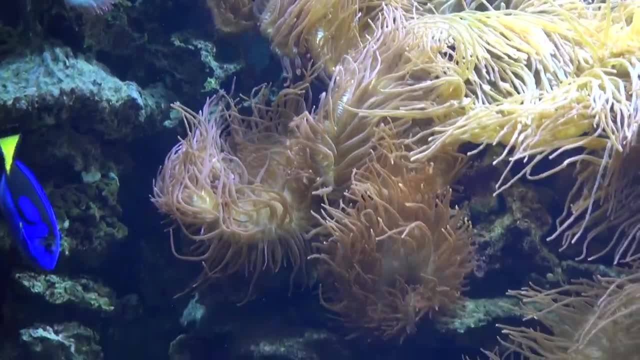 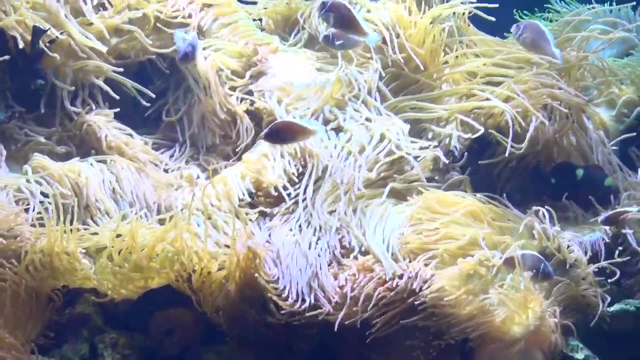 They can just kind of slink along very slowly. They don't have a shell, They don't have a skeleton. Basically, just try and picture like a jellyfish that's attached or a sea jelly that's attached to a rock. They are. 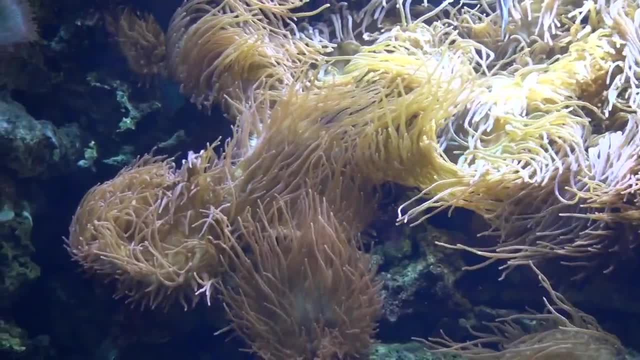 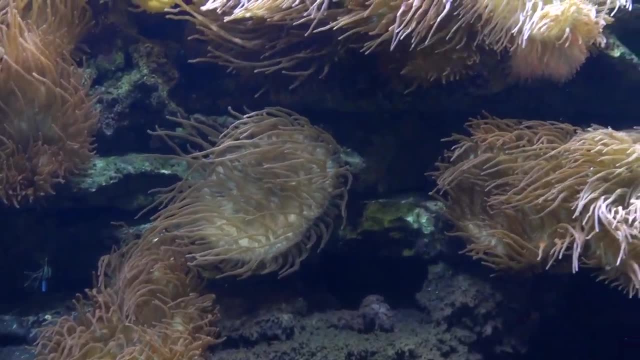 cnidarian, so they are related to the corals and the sea. Those tentacles are loaded with stinging cells and nematocysts. They can sting and capture quite large prey and ingest them. The clownfish has a nice relationship with them. 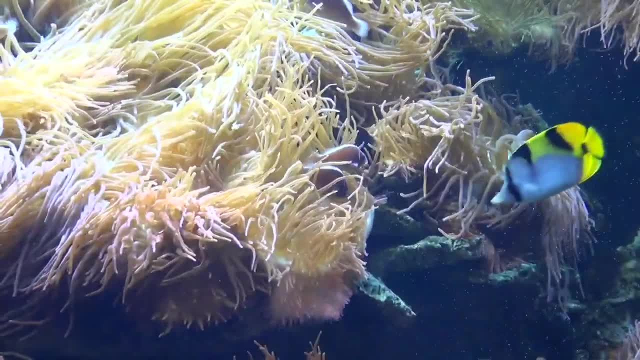 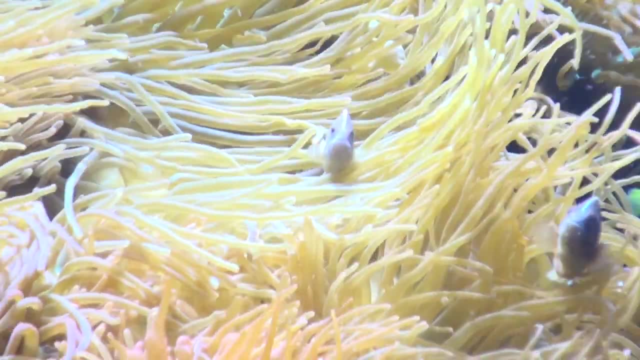 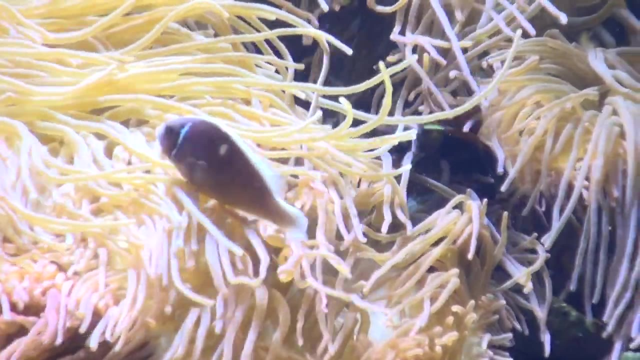 The clownfish are immune to the sting. Clownfish will protect the anemone from predation And, in return, clownfish get protection by living within the anemone, And they'll also lay their eggs underneath the anemone and these 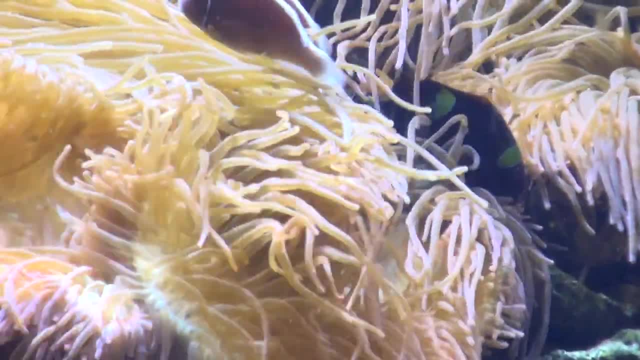 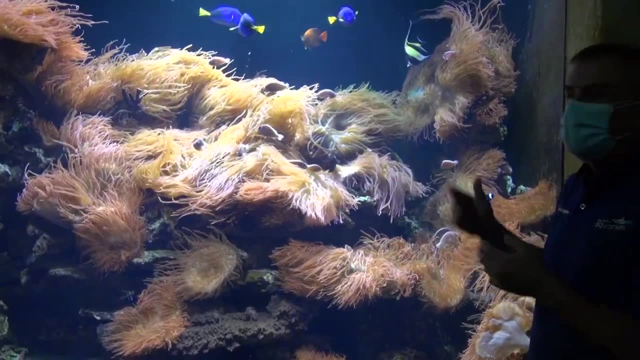 are protected by the anemone as well, So these guys will open up, kind of like a flower opens up when the sun comes up. These guys have, surprise, surprise zooxanthellae in their tissue, So they're going to open up. 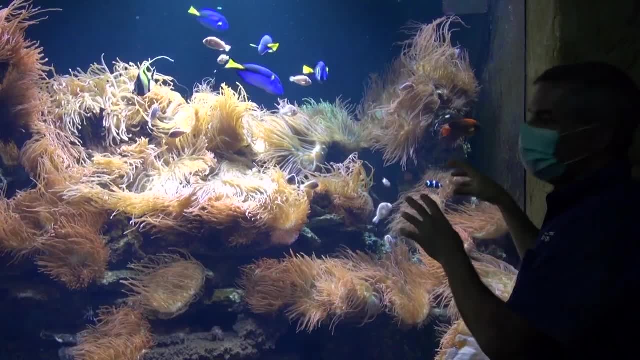 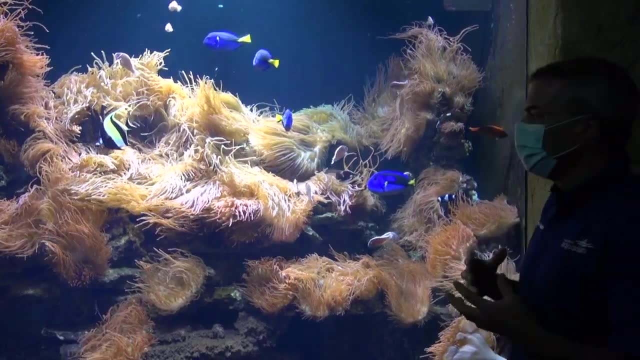 They want to expose as much surface area to the sunlight. So if you come here in the morning, these guys are a lot of. these are even bigger than the regular balloon And get larger. expose themselves to the sunlight as much as possible. 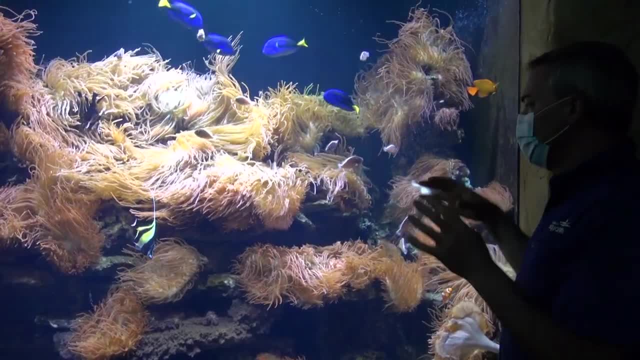 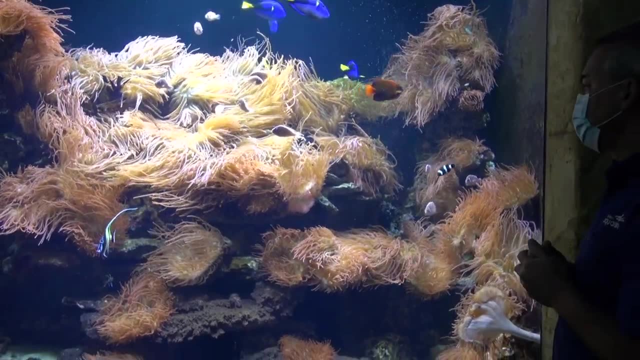 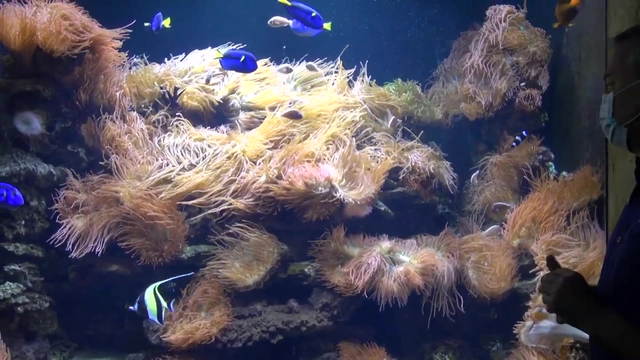 And then at night again they'll expel that water, shrink back down and find safety among the rocks, And they can also retract quickly also from predation as well. So again they have those tentacles are loaded with stinging cells. 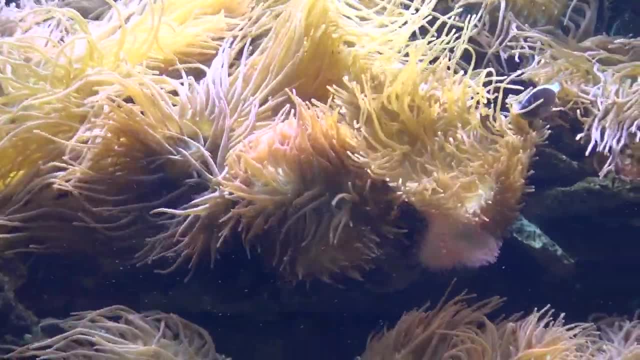 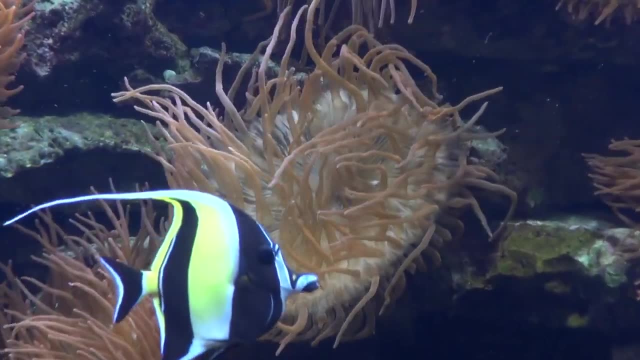 or loaded with nematocysts just like a jelly, So you don't want to be touching them. You want to get some pretty, pretty nasty stings from these guys And I could actually grab see if there's any food in the back. 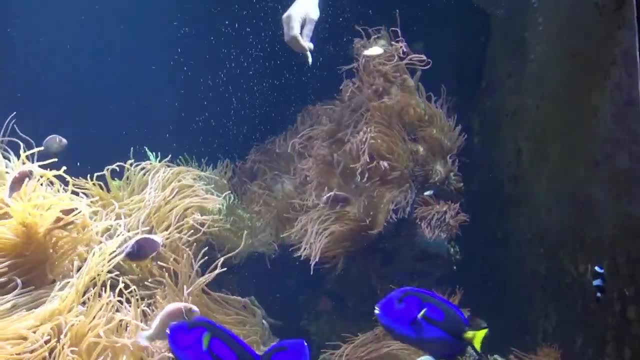 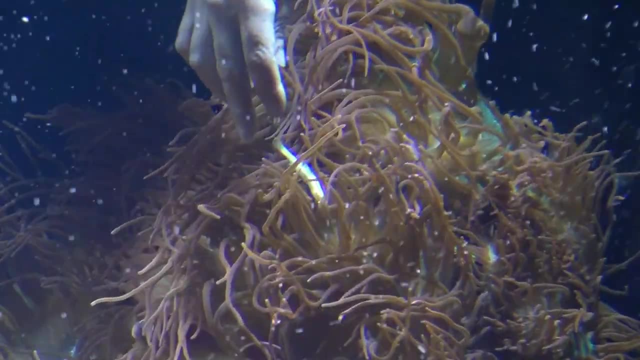 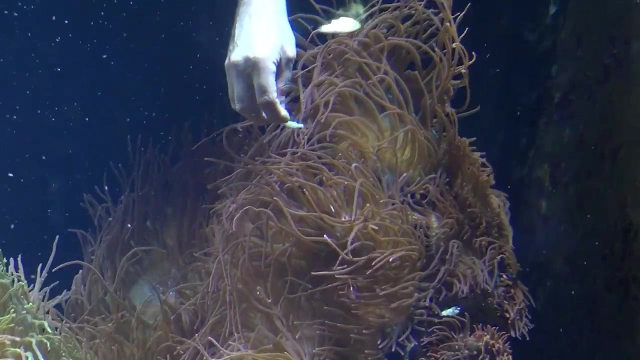 Okay. so let's watch as Joe feeds the anemones some silver sides, some little frozen silver sides, So you can see his hand going in descending towards the tentacles. Look at those tentacles, reaching out to try to grab that silver side. 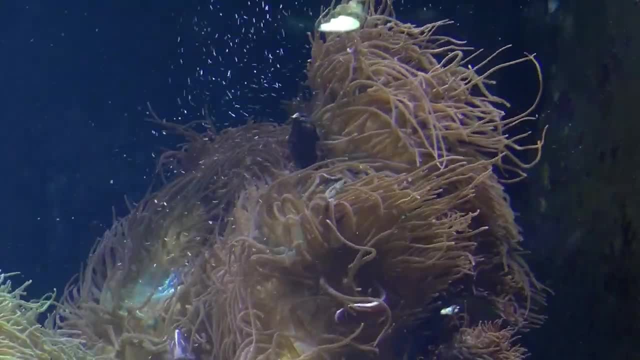 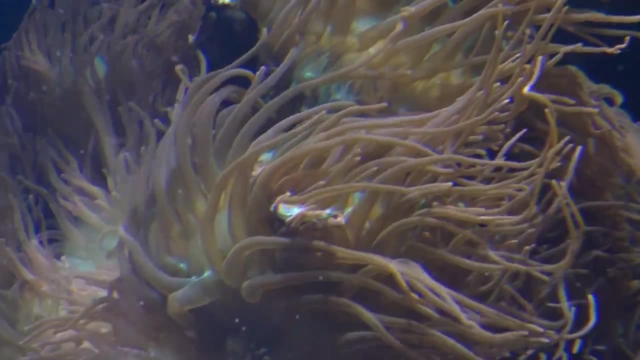 Look at that. There you go. Look at them. They're grabbing that silver side with their tentacles, So that one polyp has grabbed this silver side and it's going to be basically moving the silver side towards its mouth. You can see. 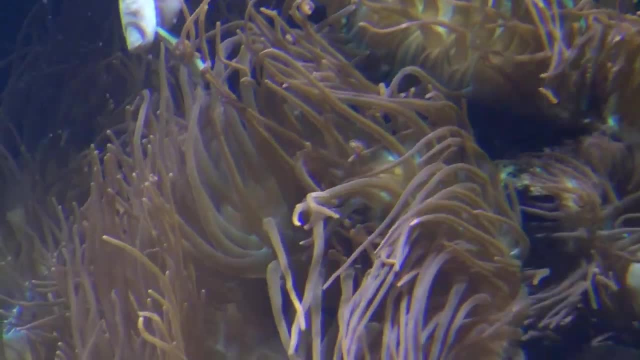 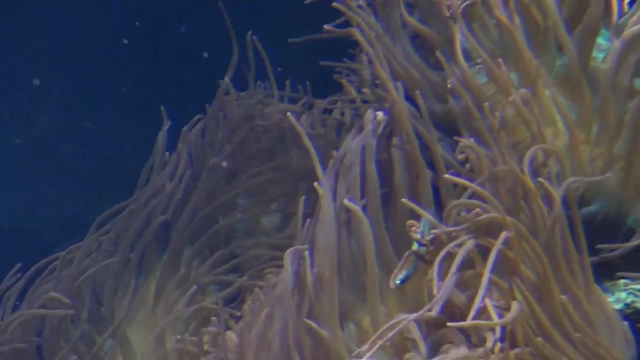 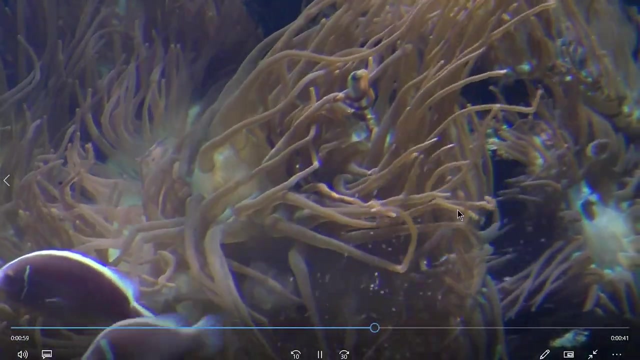 that behavior again. Watch as the tentacles wrap around the silver side. That's amazing. Look at that. And so they're slowly going to move this. this You'll see in a moment. the mouth, Actually you can see it. 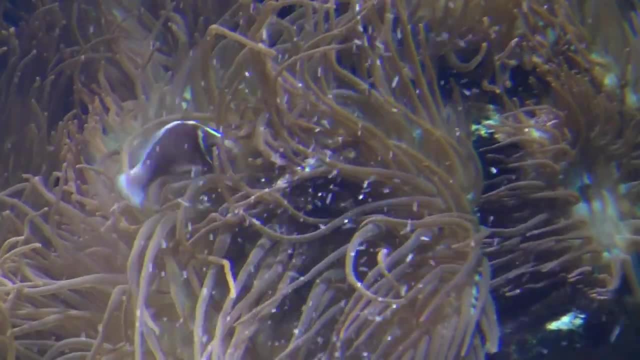 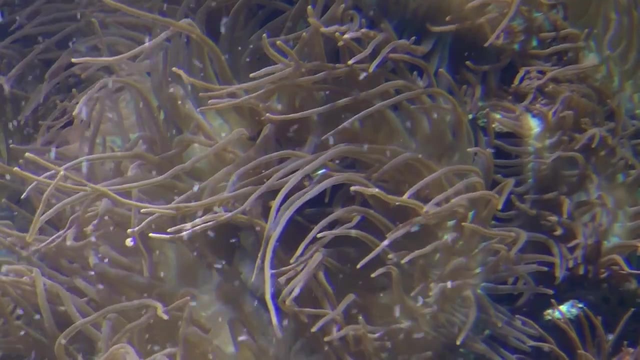 right now, The mouth is actually becoming engorged. You can see it right down here, right over there, And so, as Joe mentioned earlier, these guys are Cnidarians and they're related to corals, but they're not quite corals. 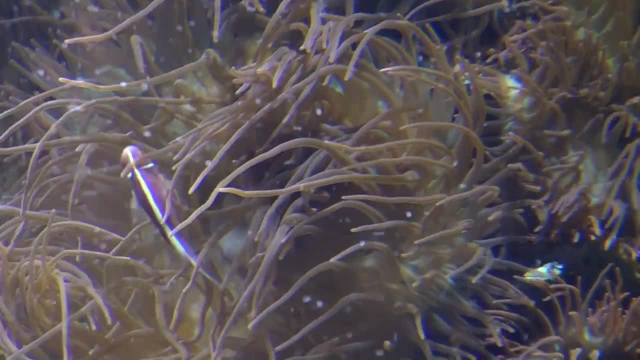 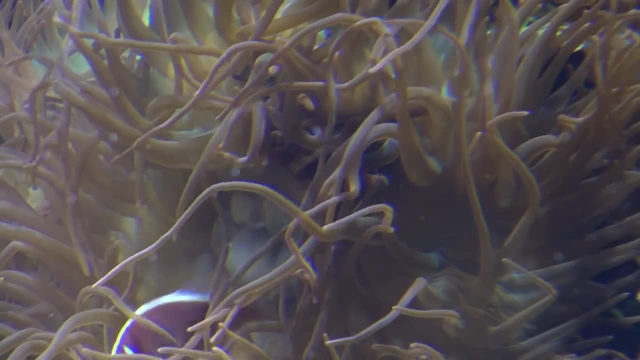 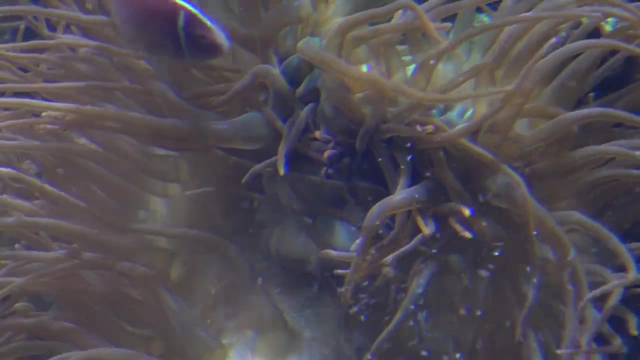 They're in their own little order within the hexachoralia. That's that subclass. we talked the stony corals, but you can see how behaviorally and even morphologically they look very similar. check that out, look at that mouth. so there you can. yeah, you can. you can see the mouth has uh. 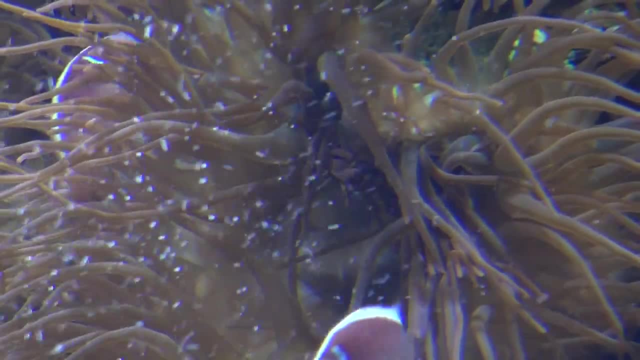 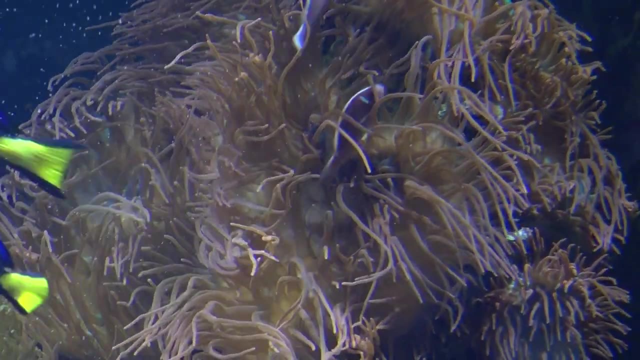 opened up a lot more to ingest- ingest the food. getting ready to ingest the food: some of the silver sides are still wrapped in the tentacles. you saw how the uh tentacles were able to grab the food. they're the way. the way they're able to grab that is, they have those nematocysts. 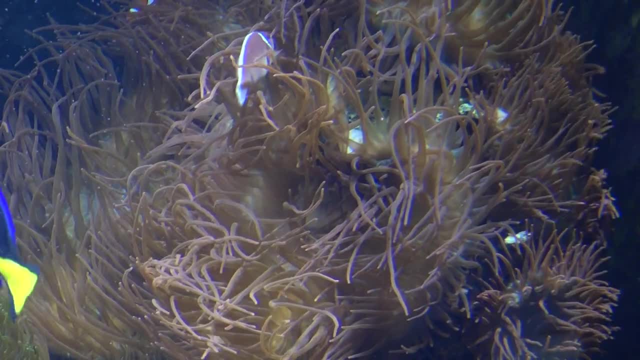 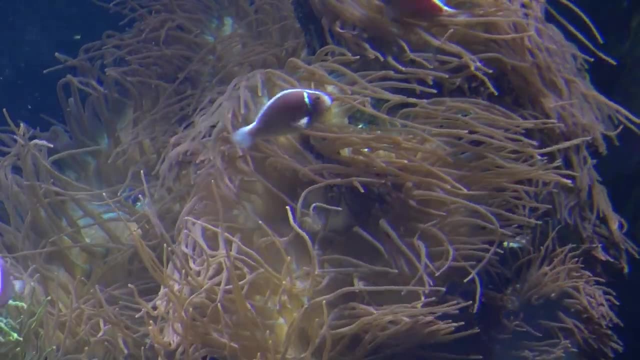 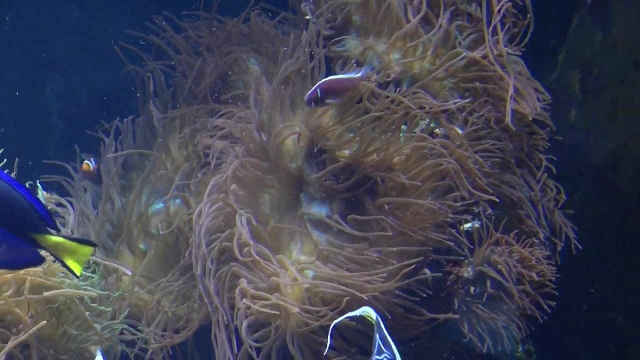 those stinging cells and those are basically little uh poison tipped harpoons with a tether and they're shooting into the food item and harpooning it and then grabbing it and then they're going to just slowly work their tentacles down. so there's still some. there's some silver. 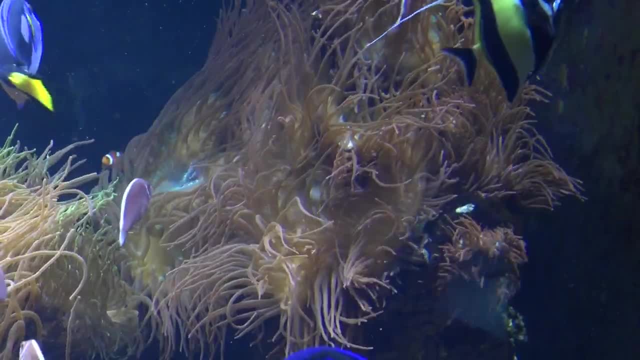 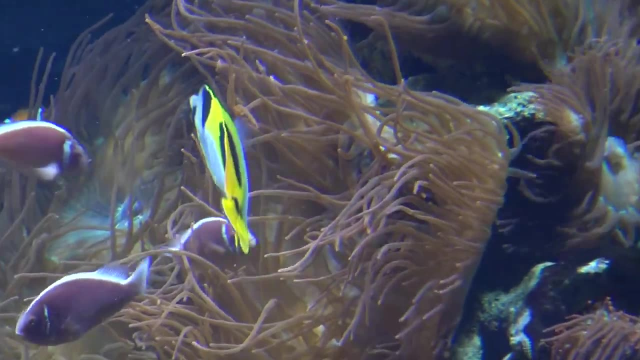 side still wrapped in those tighter tentacles there, and he's going to tuck that into his mouth. so this is uh you're kind of looking at. let's pretend this is a huge, a huge coral polyp or a blown up vision of a coral polyp eating the corals will do the same. 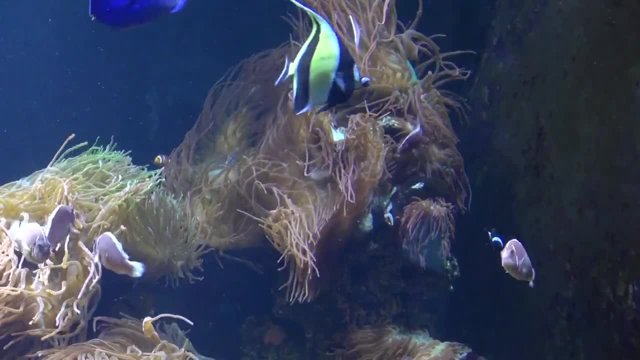 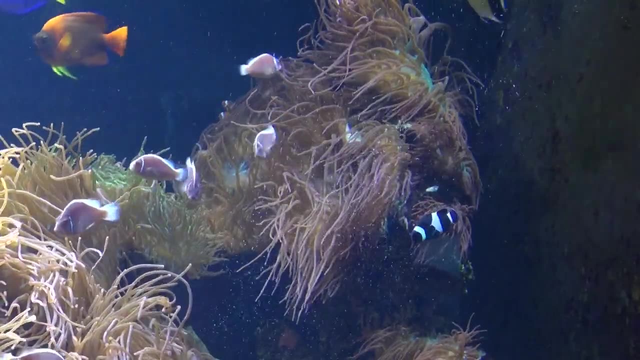 thing. they've got those tentacles around their mouths and they're going to grab a food item- not not a silver side per se, but some corals certainly can eat something that large- and then they're just going to slowly work it into their mouth. so, just like forests on land, 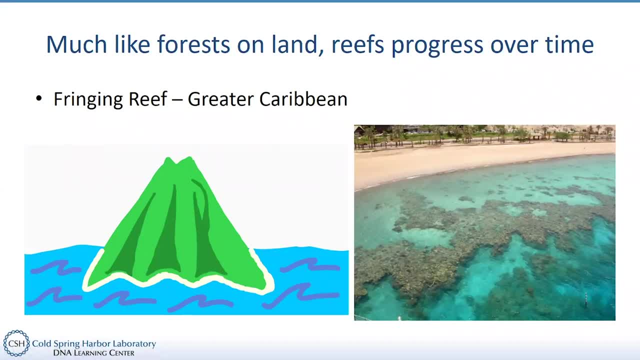 reefs progress. over time, they change in both their structure and the biodiversity that they support. i just may take them a lot longer period of time to do so, and so we start off traditionally as a what's known as a fringing reef, and essentially these occur around volcanic or seismically active islands and uh or land. 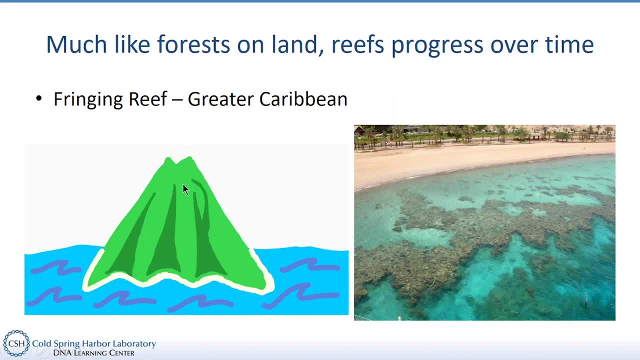 sources where you have igneous rock and nutritious material coming down the island and basically settling around the waters of that island, just off the coast and just off the the land, the shore actually, rather- and what winds up happening is all this nutritious material will attract and allow for the colonization of different critters around the circumference of the island. 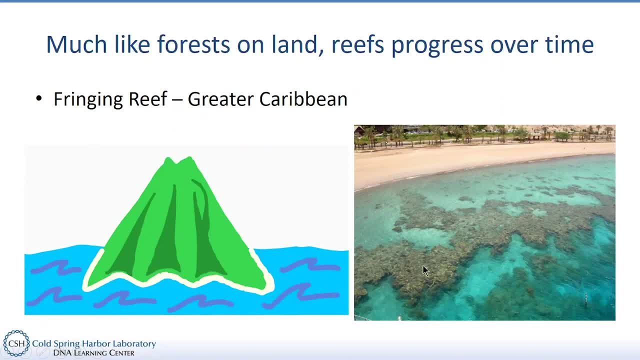 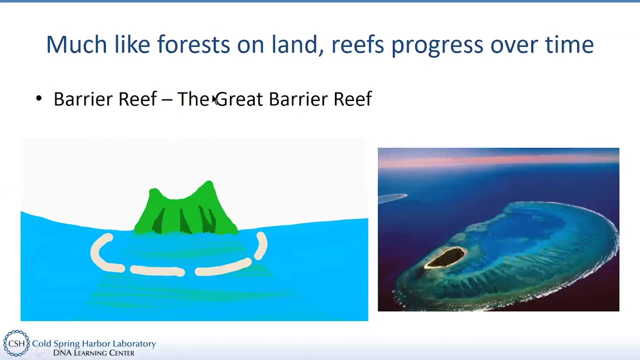 and this is what will establish, or begin to establish, a reef, and so there's a lot of these, for instance, in the caribbean. so a lot of the land masses there have fringing reefs, and so, over thousands of years, though the reef will, the island will eventually sink. it'll eventually. 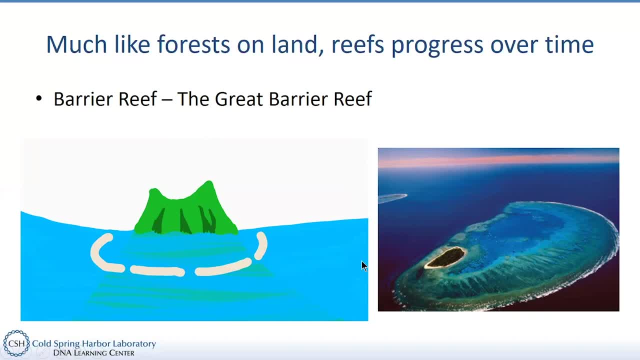 retract back into the sea or recede back into the sea and all of those little, those reef colonies that that began to grow around the perimeter of the island, will remain where they are and over many generations they'll grow and die and lay down their calcium carbonate. 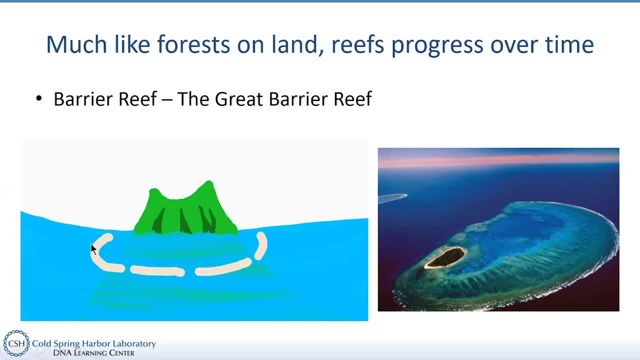 skeletons which are concrete and compact, and what will be left behind after the island recedes? is this barrier structure that might be a solid barrier? um, like this, in the image it almost looks like a solid structure. it might be a little fragmented area, but what will be left behind? 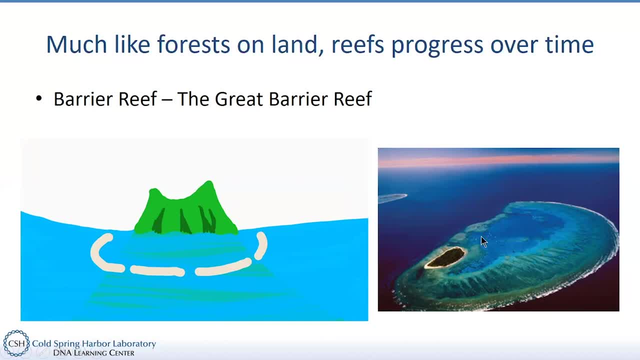 is a barrier, and it's a barrier that will be left behind, and it's a barrier that will be left behind with the island still sticking out of the middle, and so this is what we call a barrier reef, and an example: obviously would be one of the largest reefs in the world, the largest reef in the world. 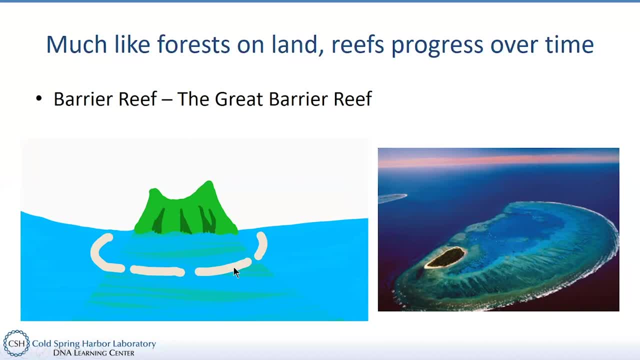 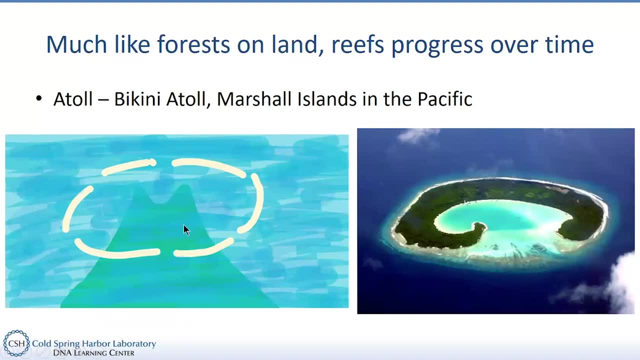 the great barrier reef, but this will will- uh, this will will progress even further until the island will be completely submerged in the sea, and now you will no longer see this island, and what will be left behind is this little lagoon in the middle, and so around here we still have that barrier layer. 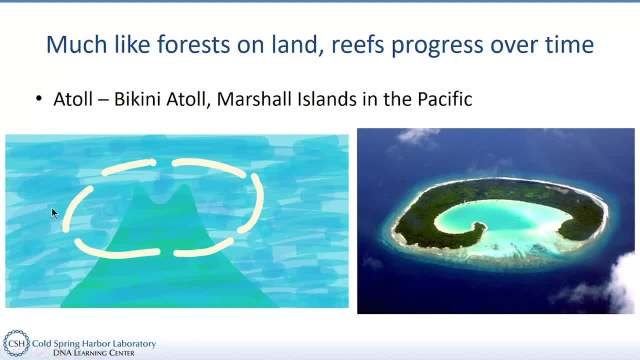 but um, the barrier itself winds up serving as a protective layer from from uh storms and the currents, and so softer, more delicate species can start establishing on the inside, and we call this type of reef an atoll uh. so, for instance, the south in the southeastern uh eastern asian islands in. 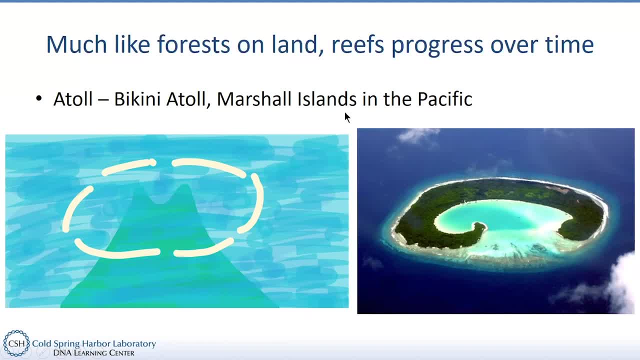 the pacific ocean. there's the bikini atoll and the marshall islands. there are tons of these atolls and they all kind of have this: look to them. where it's that? we have the atolls that are the barrier that's been left behind the island. the middle has receded and disappeared and you. 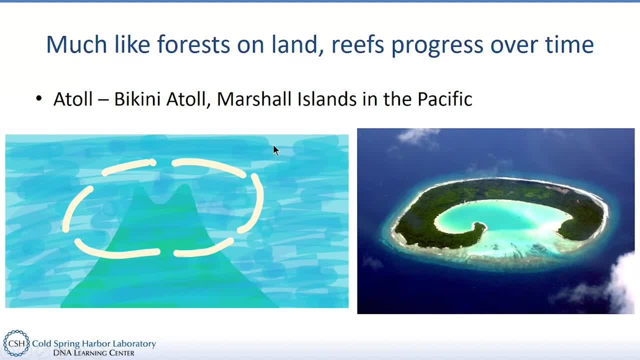 have this little lagoon in the middle, and that's essentially the progression, and this can occur over hundreds of thousands of years, so it's a lot longer than a terrestrial forest, but it does shape the type of biodiversity that uh, that can, that can use the reef as its habitat. 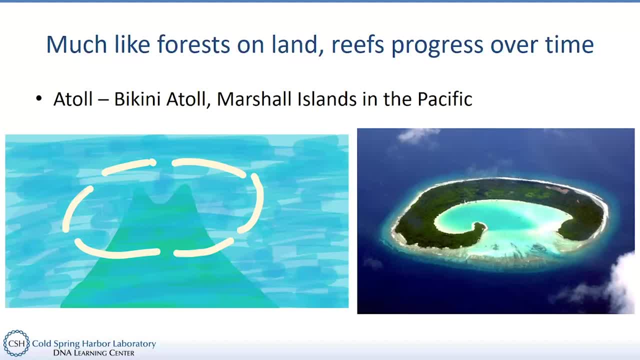 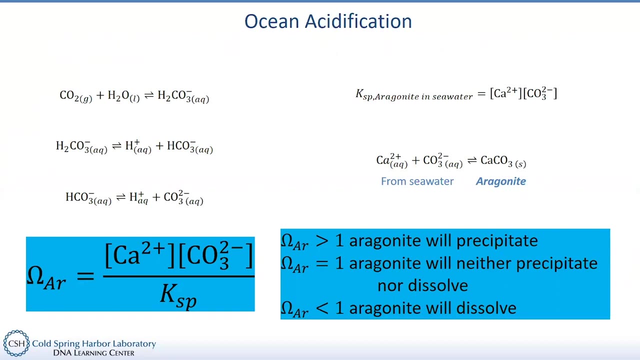 and so you know that's one of the reasons that makes these really advanced uh reefs throughout the world such biodiversity hot spots and unfortunately, they are at risk, and a lot of the reasons that they are at risk have to do with ocean chemistry and factors that, honestly, we may be contributing to with the production of greenhouse gases, and 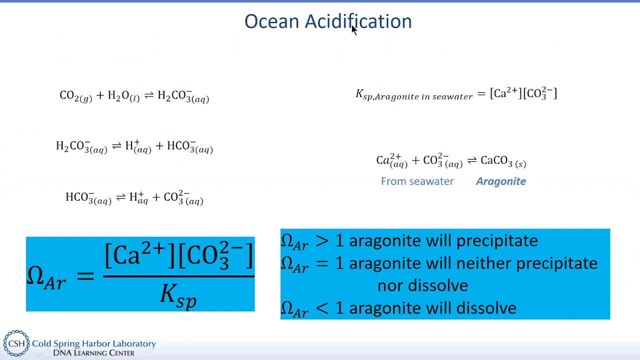 the acceleration of climate change, and so ocean acidification is one of the first first ones, and ocean acidification means exactly what it sounds like. so we have the acidification of the ocean and i wanted to return to this, uh, chemical set of chemical reactions i talked about before, because i 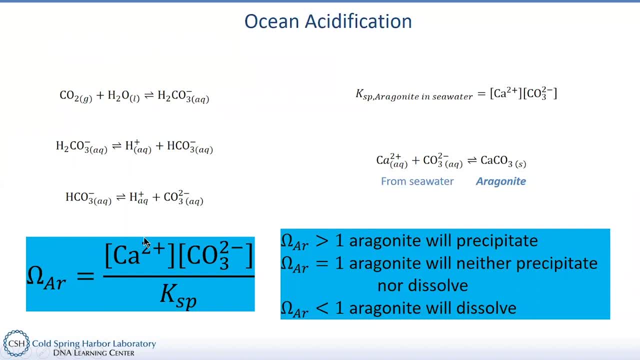 wanted to apply something that you may have learned in high school chemistry, known as Le Chatelier's principle. so that's when you manipulate the one of the the conditions of a certain chemical reaction in equilibrium and you can push the reaction in one direction or the other, and it's a good, a good time to use that as an example to explain ocean acidification. 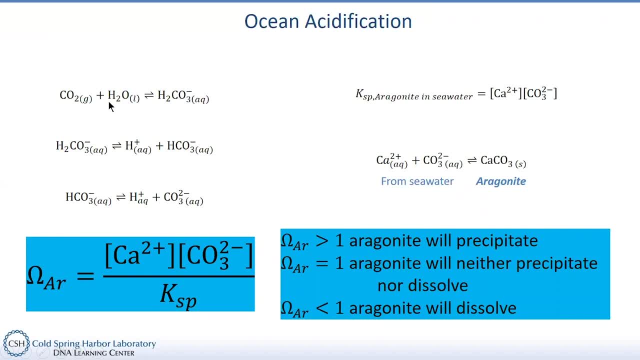 so recall that carbon dioxide dissolves in seawater to form this carbonic acid. so as atmospheric carbon dioxide increases with human activities um or or whatever the reason may be, if that or that atmospheric carbon dioxide increases, it will push this reaction. an increase in this reactant will push. 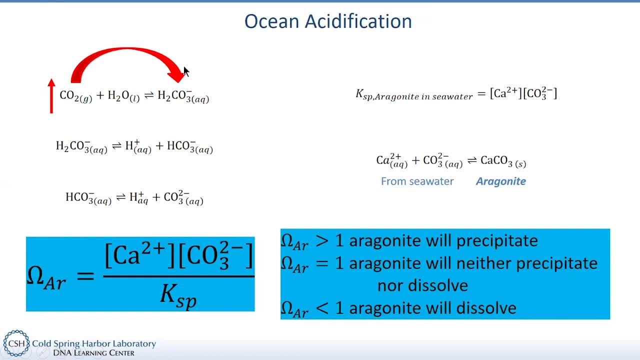 the reaction in the forward direction, producing more carbonic acid. the production of more carbonic acid means that the second reaction here will be pushed in this direction and you'll have a greater production of h plus and h co3 minus, with an increased h co3 minus. uh, that should push the. 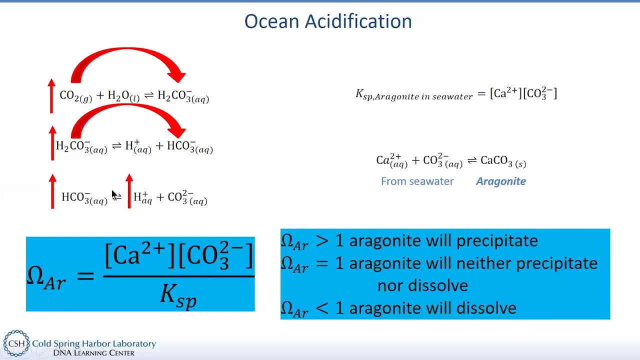 reaction in this direction, but notice that we also had an increase in the production of h plus, so this reaction kind of stays put. in fact, if anything it might go in this direction, it might actually be pushed to the left, and so we will have less carbonate production in the sea and 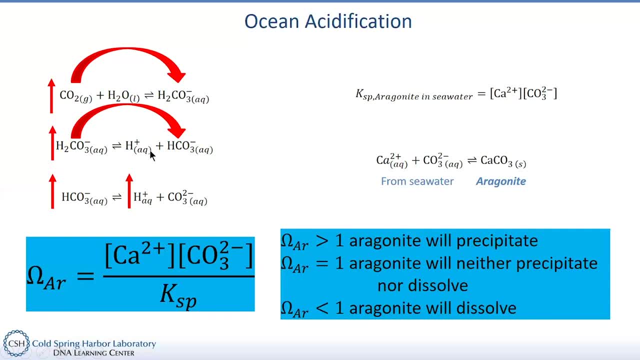 we'll be stuck in this, this sort of middle area here with high h plus concentration and high bicarbonate ion, and so high h plus is directly correlated to ph and acidity, and so the lower the, the higher the acidity and the higher the concentration of uh, hydrogen ions or hydronium. 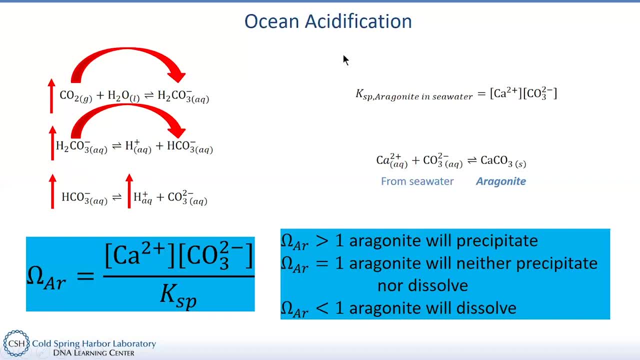 ions, h3o plus, and so this is where that term ocean acidification comes from. now you might be telling yourself: oh okay, well, whatever that's, that's fine. what's the big deal? they can still- corals can still, uh, produce carb calcium carbonate skeletons which ate with h3o. h, co3 minus, but unfortunately that 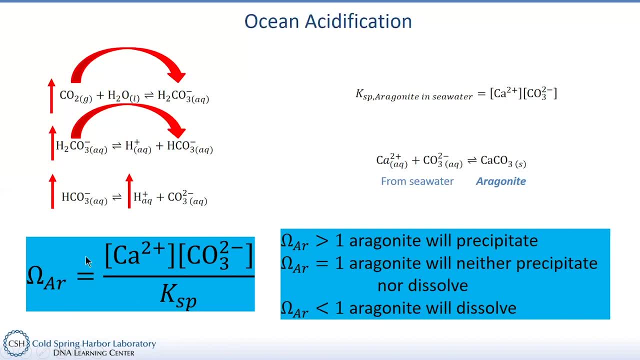 is not the case. they have a much more difficult time with that, and that has to do with the saturation content of the ocean acidification, and so that's where the term ocean acidification comes from. if you decrease the- uh, the solubility, uh, i'm sorry, if you decrease the concentration of carbonate ions, 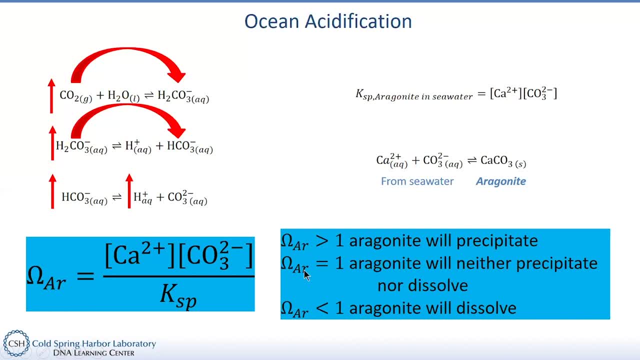 here. that's going to bring down our saturation constant. remember that our saturation constant below one or as you get closer to one, the likelihood of aragonite to precipitate or solid in solution will decrease and you'll start the. an aragonite will the, the will begin to. 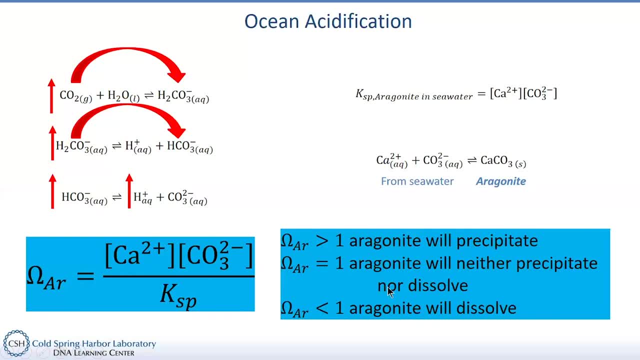 dissolve, or calcium carbonate will begin to dissolve and that's going to bring down the solubility of the ocean acidification and that's going to bring down the solubility of the ocean acidification. so those conditions favor the dissolution or the breakup of calcium carbonate. so what that means, 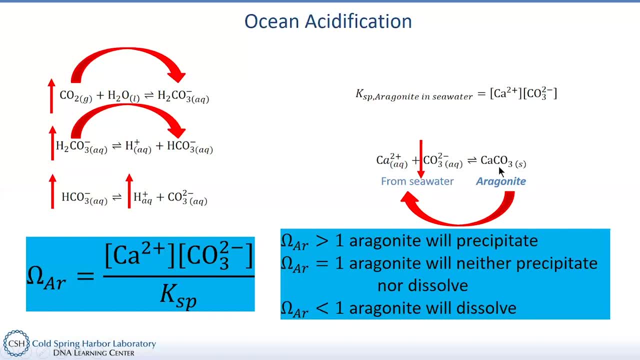 is we are going to have less calcium carbonate, we're going to have calcium carbonate dissolve and wanting to dissolve back to its constituent ions and so the uh, which is not good and because, because you have these conditions in place, it's not going to proceed and want to precipitate. 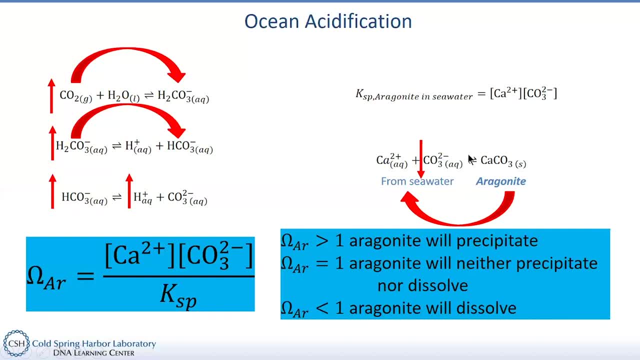 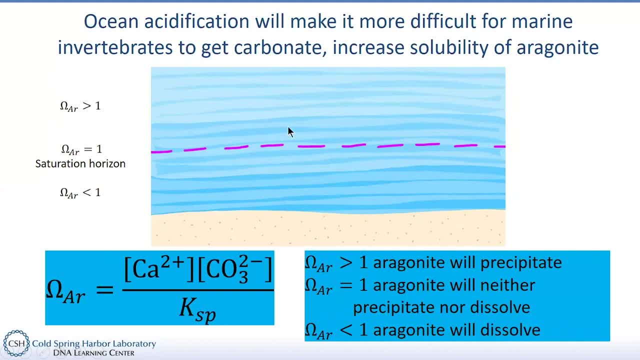 much. uh, I there. so, if you think able and Ra tell you how depths here we could think that at the surface, the saturation constant of aragonite tends to be greater than one. The saturation constant tends to be less than one the closer you get to the. 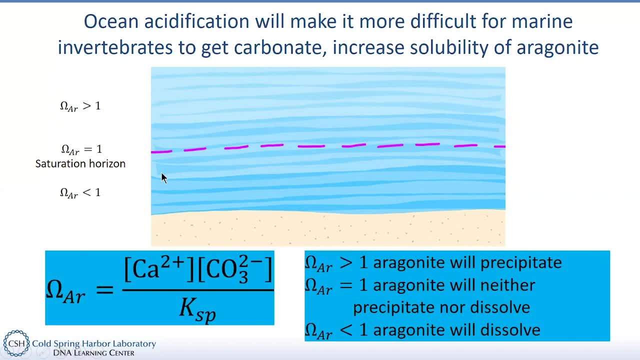 C4. That's actually because the solubility of calcium carbonate will increase with decreasing temperature, counterintuitively. Now, right in the middle here there is this line, and that's where the saturation constant is equal to one, and we call that the saturation horizon, And so corals. 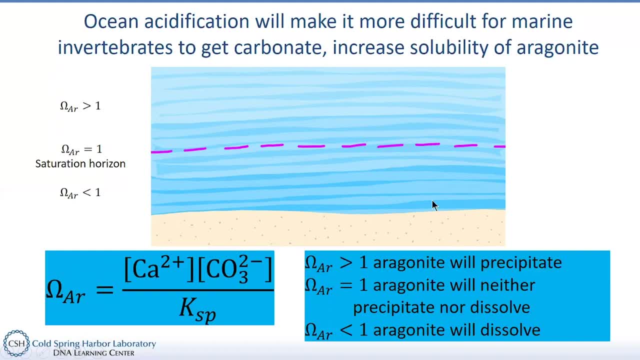 ideally want to be up here somewhere. So you can imagine that this is obviously a simplified drawing, but you can imagine that corals would be living on a depth up here, somewhere above the saturation horizon, hopefully somewhere, probably around between like two, I don't know, it might. 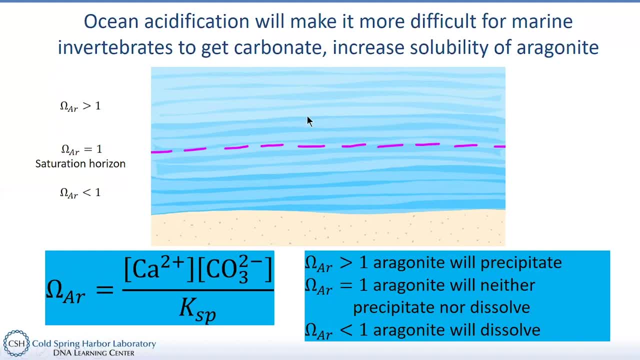 be low, but like three and four and a half for the saturation constant. And so if ocean acidification is equal to one, then the saturation constant is equal to one. And so if ocean acidification occurs, what's going to wind up happening is it's going to drive the saturation. 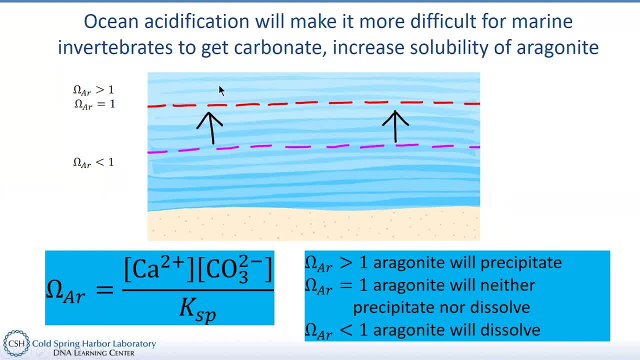 horizon up in depth, So it's going to basically decrease the depth at which the saturation horizon will be, meaning that the habitat, the potential habitable regions for certain types of coral and obviously a lot of other oceanic invertebrates, it's going to be much more limited And so 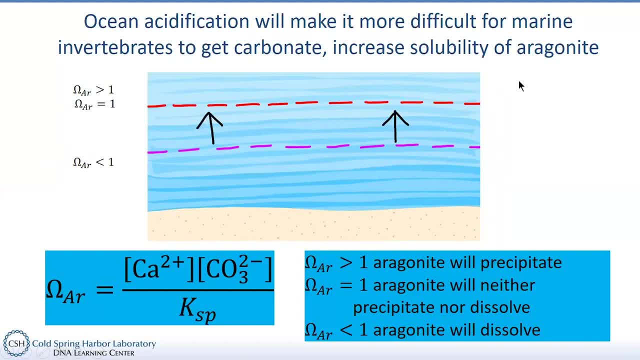 essentially what this is doing is it's making these invertebrates, like coral, have a much more difficult time getting carbonate out of ocean water and keeping that calcium carbonate skeleton strong and healthy. And, what's more, what that's going to do is it could lead to things like coral. 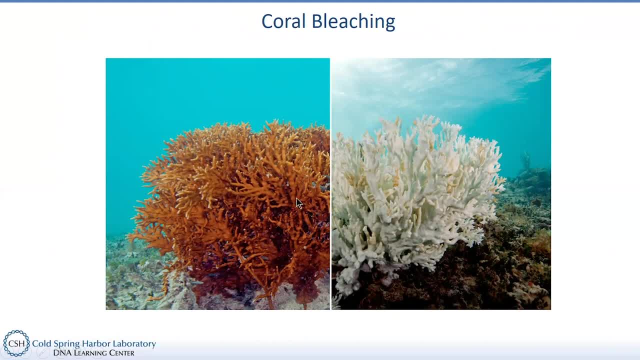 bleaching, And so the coral bleaching is essentially so. here's a before and after of coral. and you have the zooxanthellae that live in coral, quite happily under certain conditions, including temperature and acidity, And when the acidity or the pH, I guess I should say when pH- changes. 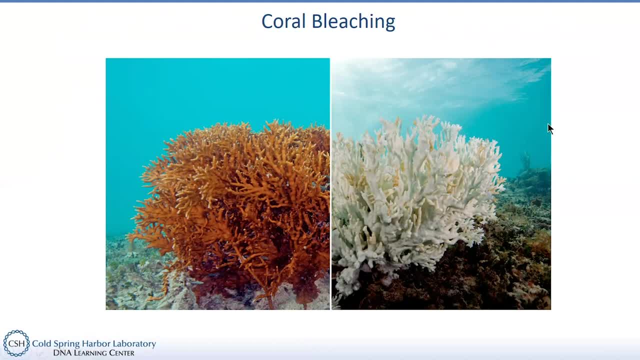 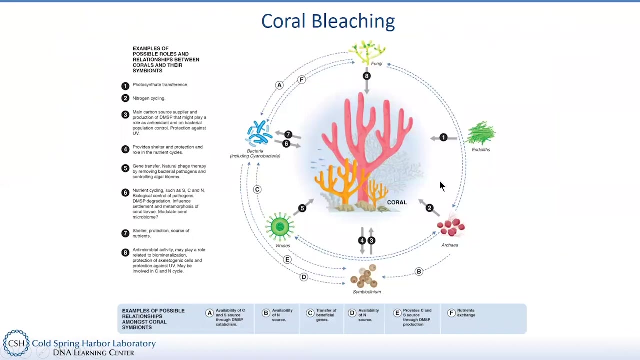 or temperature changes, those zooxanthellae will simply vacate their coral symbiotes and go out and find a new location where conditions are favorable, leaving the coral to fend for itself, which is definitely not a healthy situation for the coral. As it turns out, the symbiodinium that 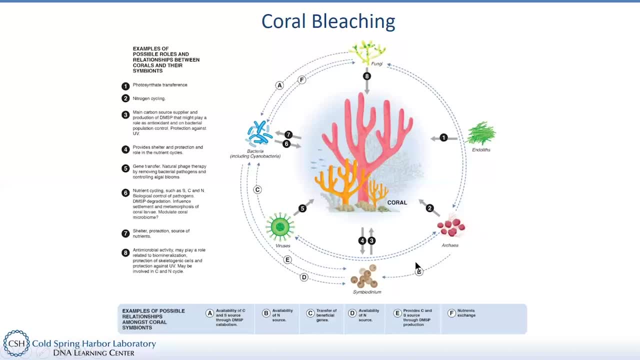 I mentioned earlier the zooxanthellae. they're not the only symbiont inside coral. In fact, there's a mucus layer surrounding coral and there's a huge microbiome of different microorganisms that coexist with coral, And each of them have a particular symbiotic relationship. 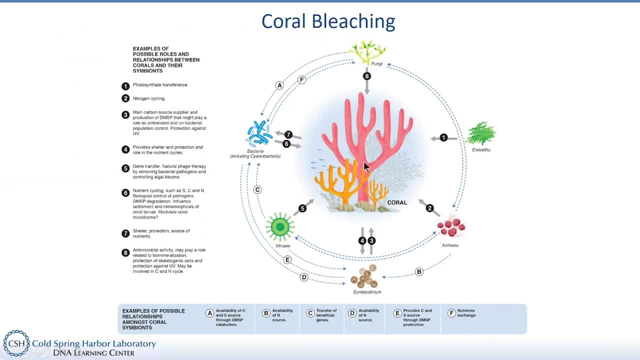 with a particular coral species, And it's been shown that even slight increases in temperature of seawater by about a degree Celsius or so can cause the profile, the diversity of the microbiome of a coral to dramatically shift, meaning that those corals might be very sensitive. 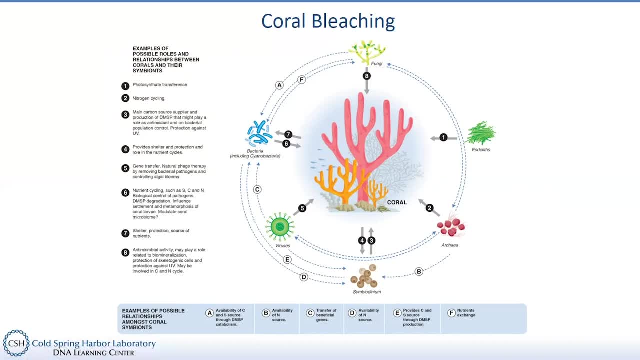 to even a small, a perceptively small, increase in temperature, And all of that leads to destruction and reef destruction. Those biodiversity hotspots, those huge centers of life wind up being strangled in the oceanic environment due to these fluctuating conditions, And so 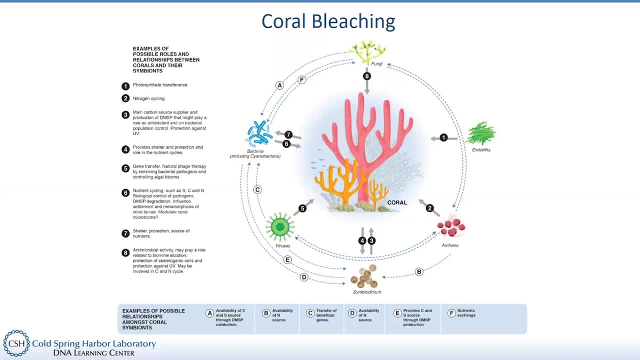 that leads to The idea of conservation. So how is it best? how best can we prevent these vital ecosystems from disappearing? Let's take a look. As we've seen, reefs are biodiversity hotspots And, unfortunately, due to things like ocean. 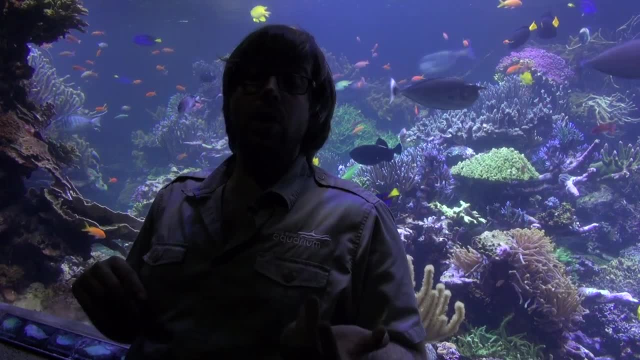 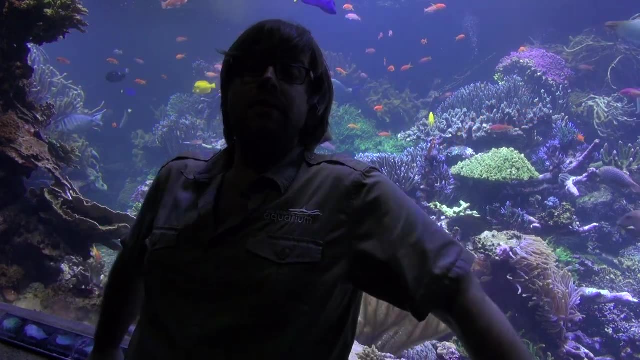 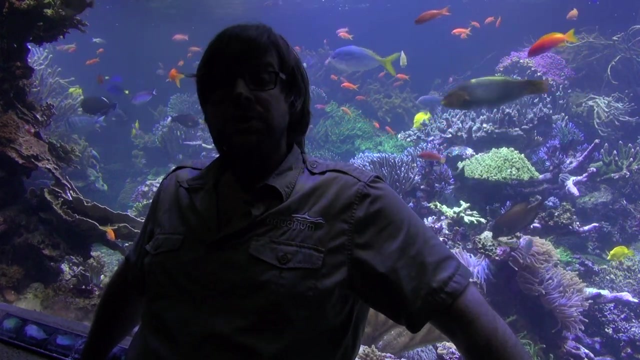 acidification and coral bleaching, the ecosystem as a whole is at risk, at serious risk, And so when we're talking about coral conservation, one of the important concepts to understand is how to actually propagate and grow coral. And so let's go to Joe so he can show us what. 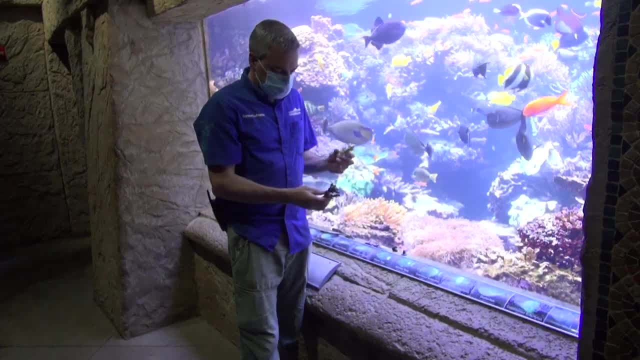 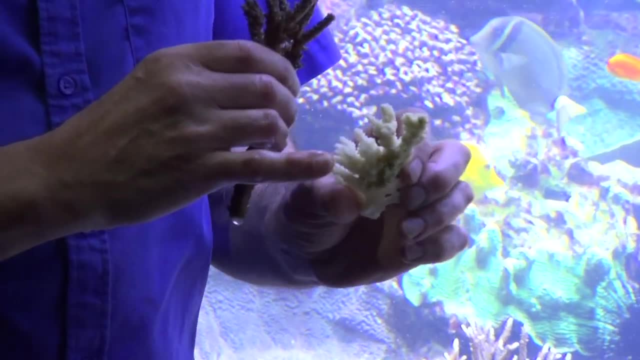 it looks like to grow a frag of coral. Uh, I'm holding in my hand two pieces of coral. One is not alive and one is alive. So the white one here that you're seeing is the dead coral skeleton. It's a calcium carbonate. 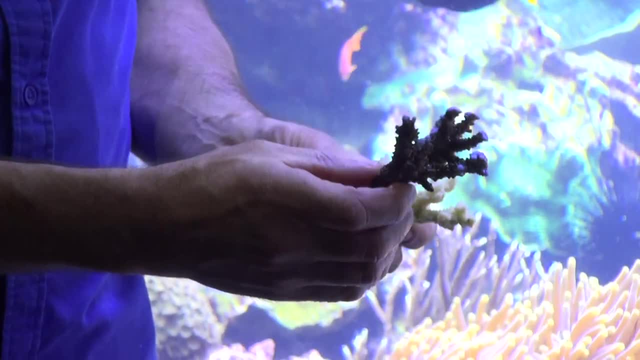 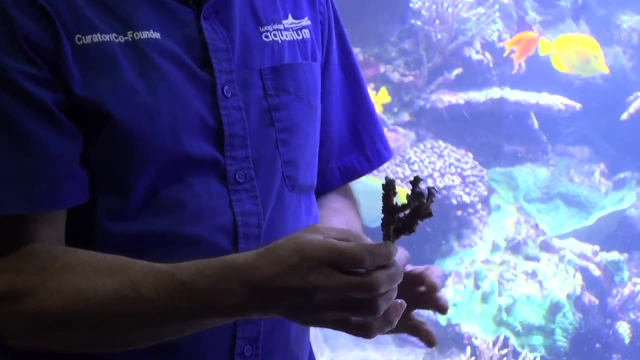 That's what the white is. When the coral is alive, it has a thin layer of tissue living over it. Now, when you're diving, you don't want to be touching or handling corals at all, but we can handle the corals during this demonstration. 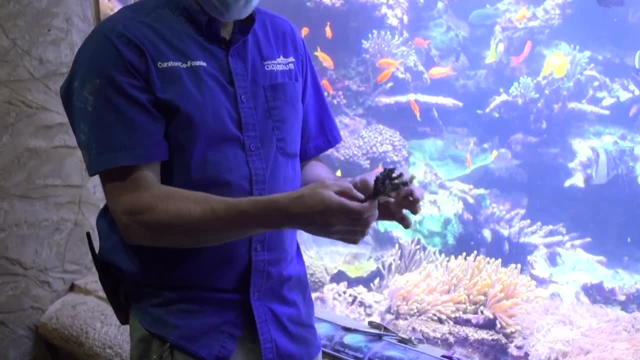 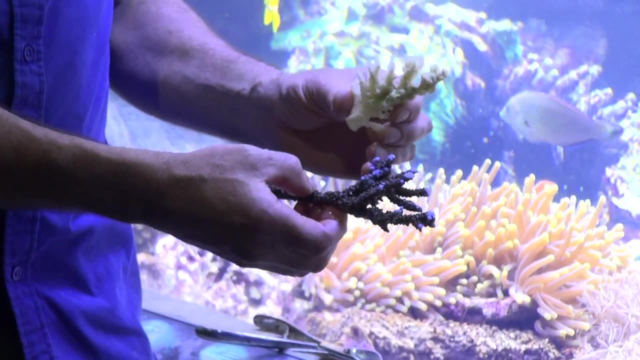 So when corals bleach, they lose that zooxanthellae, they lose that algae in their tissue, And then you're looking through the coral tissue and you're seeing the white skeleton. So that white skeleton looks like the coral has actually been dunked in bleach. 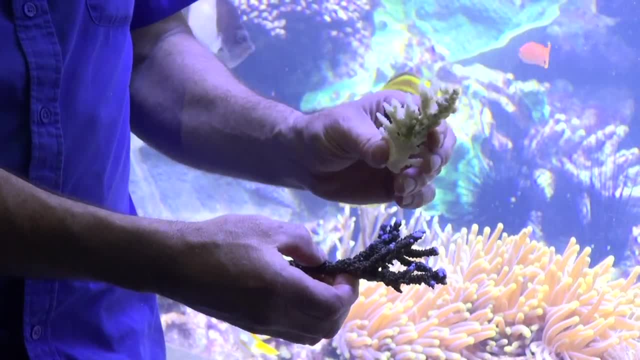 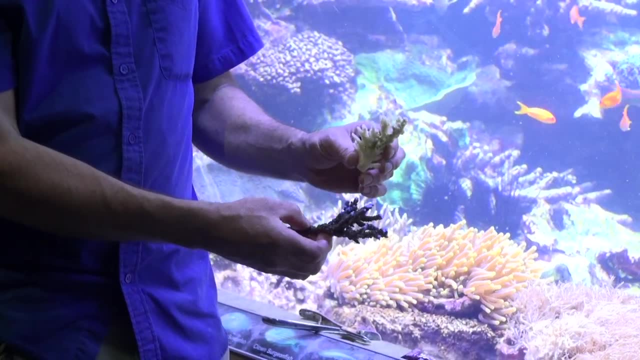 So this is a very hard calcium carbonate skeleton. This is often what you see people use for decorations in their homes and things. It's really not a great thing to do because it's a dead coral And some of these corals are being harvested at alarming rates just for decorative purposes. 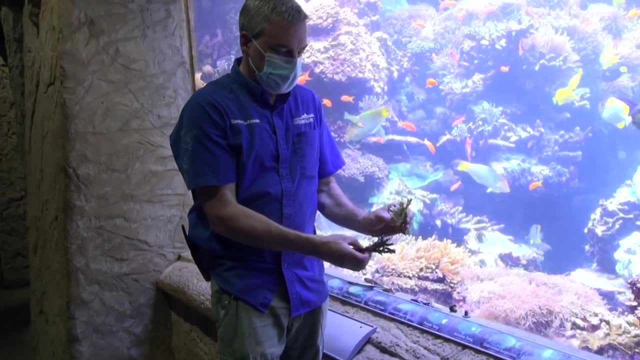 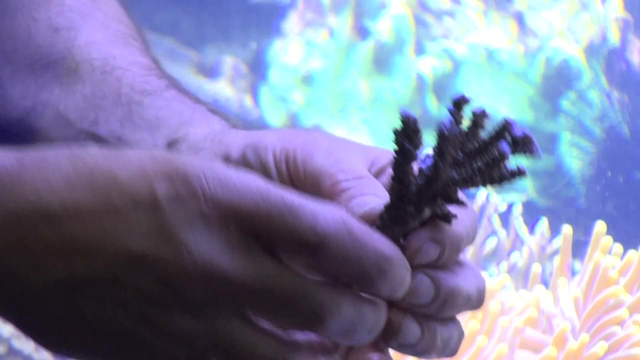 which isn't great, But this is a dead piece of coral. So now you can see the white calcium carbonate skeleton. This is a live Acropora here. We call this one Stuber Acropora, where we talk about those blue tips. 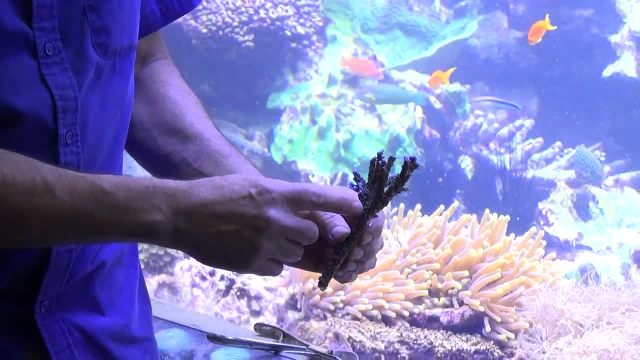 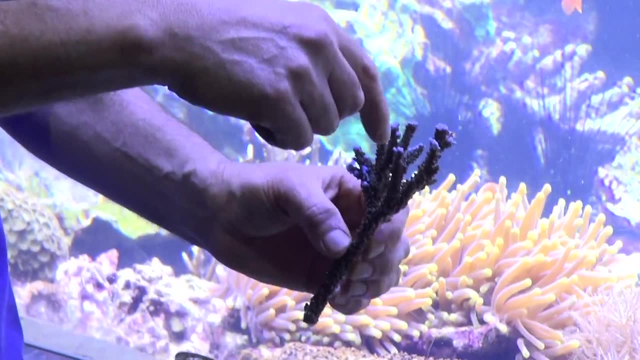 So this was the original branch growing here. And then it split, And then it split, And then it grew, And it split, And it grew, And it split, And it grew. And these are the radial polyps And the axial polyp is that colored polyp on the tip there? 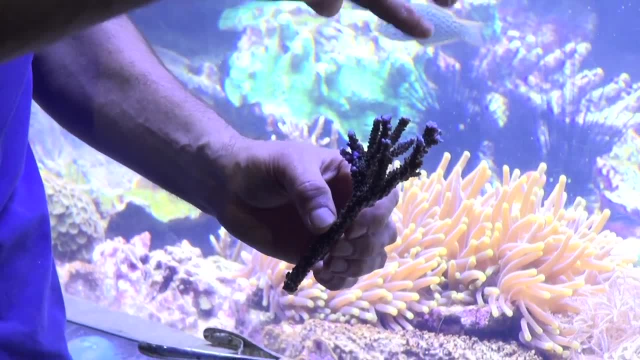 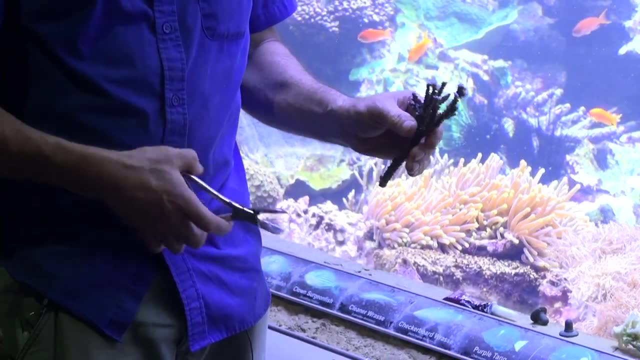 And they actually generate their own sunscreen, which is pretty cool to protect the new growth, because they're growing in these really intense lights. So what I'm going to do right now is actually propagate a coral. So they have a hard calcium carbonate skeleton. 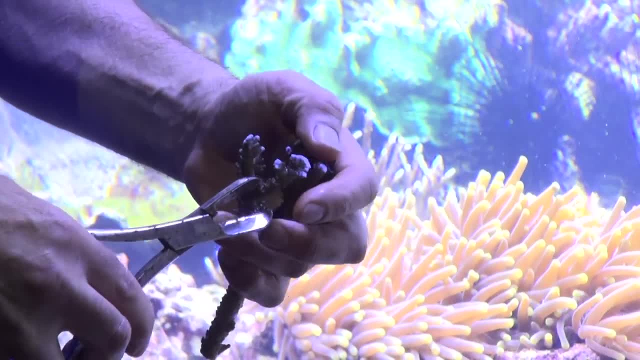 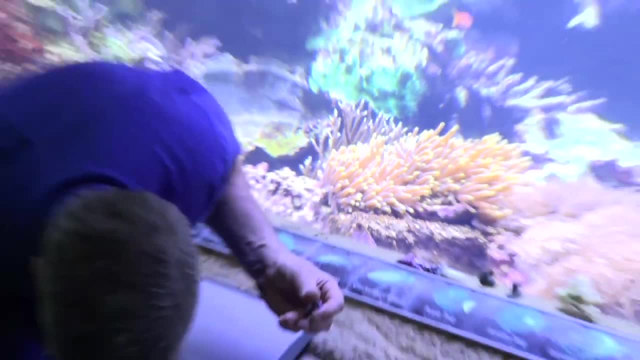 So what we're going to do is we're going to take these clippers and just gently give it a little bit of a snip, And then I'm going to put the main colony just back into a bucket of water. here And now we have a colony. 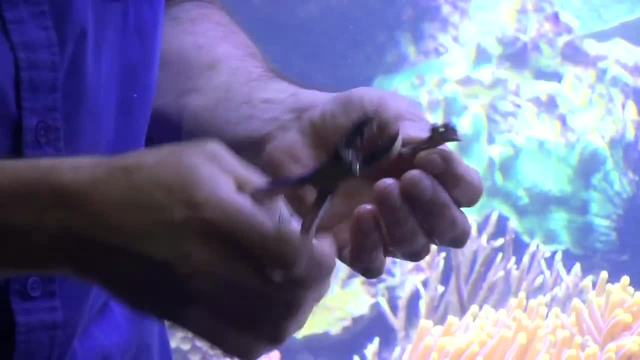 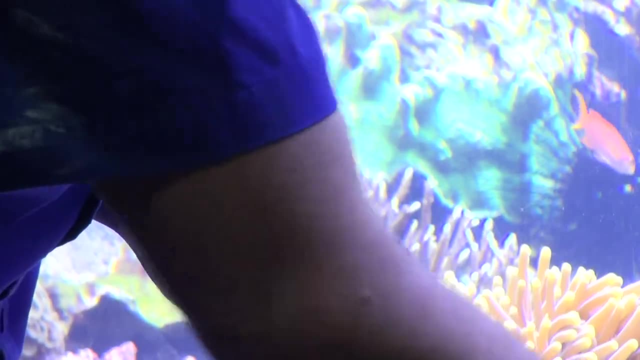 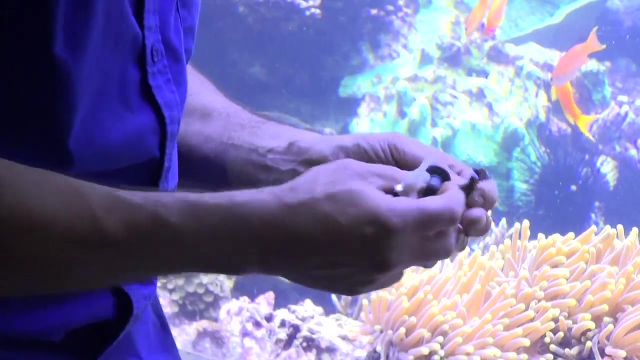 We have a little piece of coral Now. we did damage a few polyps at the part where the coral was actually clipped, But that's OK, And then what we're going to do now is take some glue And it's basically like a thickened crazy glue. 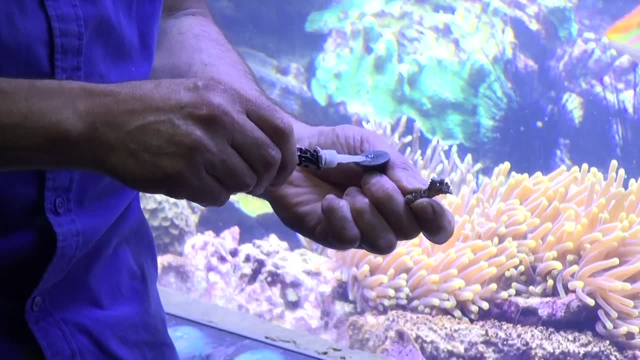 And then we have these frag plugs here And we're going to put a little glue in here, And then we're going to put a little glue in here, And then we're going to put a little glue in here, And then we're going to put a little glue on this frag plug. 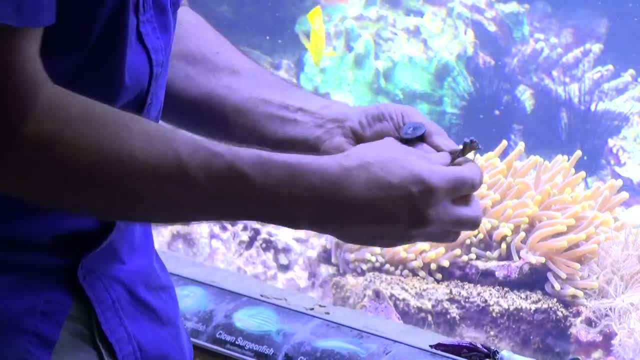 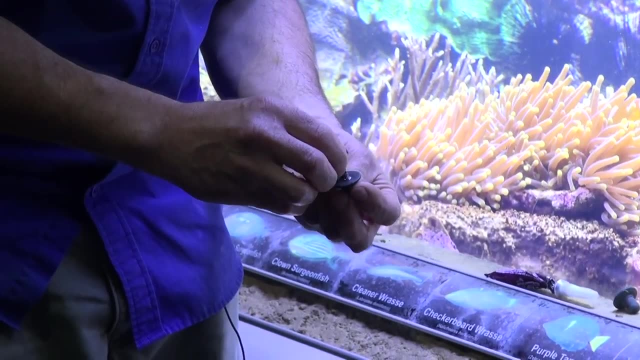 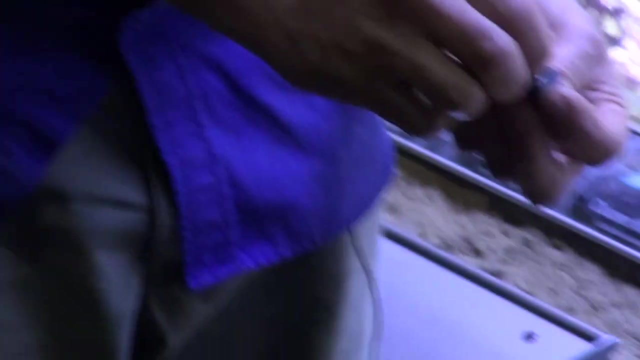 And then we're going to take this coral And we're going to glue it onto this, what we call a frag plug. It takes a few seconds for the glue to set, So I'm just going to kind of gently, yet firmly, hold it in place. 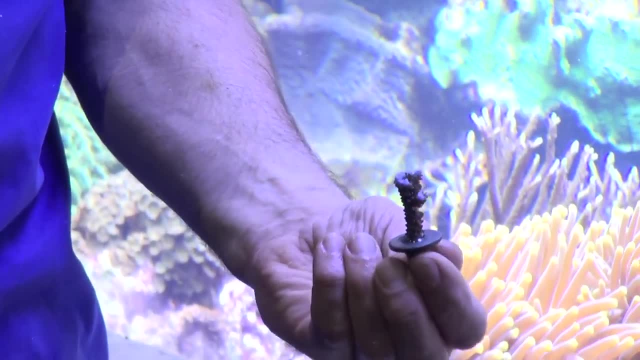 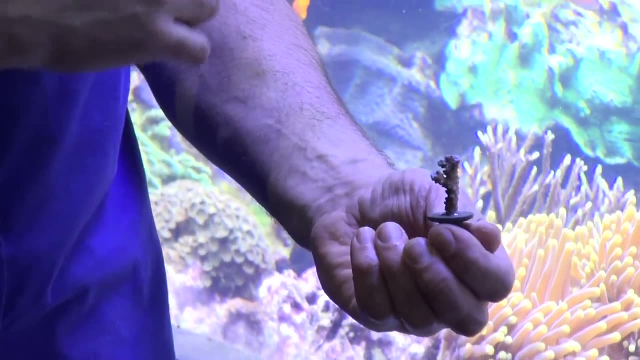 And it'll take a little bit longer to set, But now we have a little coral colony. Now this is a little coral colony that can easily grow into one of the big colonies that you see here in the tank, In fact, a lot of the colonies that you do see in this tank. 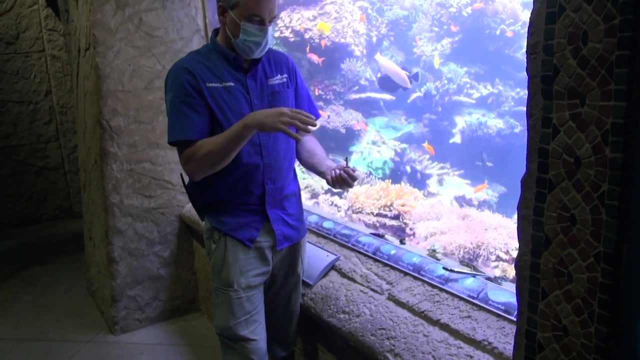 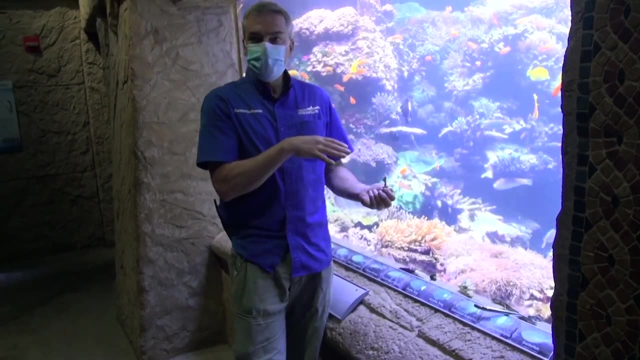 did start out as small little fragments like these and that have grown in through the years. And what's great about this is now I can propagate this coral. I can take a coral, cut it up into a bunch of pieces and then grow entire new colonies out of it. 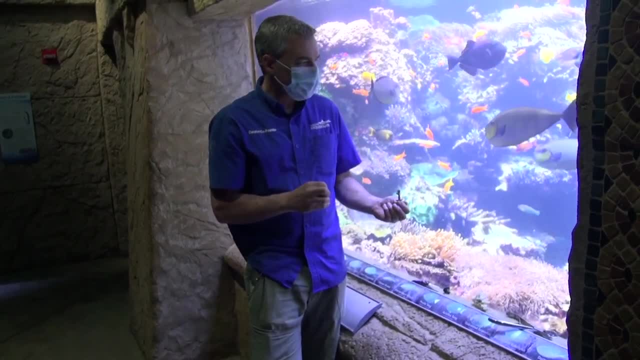 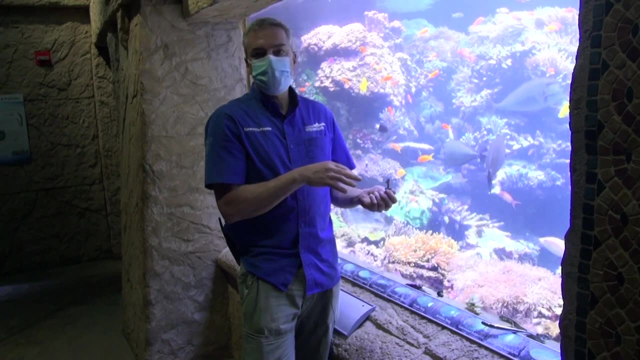 And what we figured out in the aquarium industry and the hobby, like 30 years ago, is how to figure out how to keep them alive in the beginning and then to grow and propagate them. Corals will propagate themselves by fragmentation. A big storm comes through. 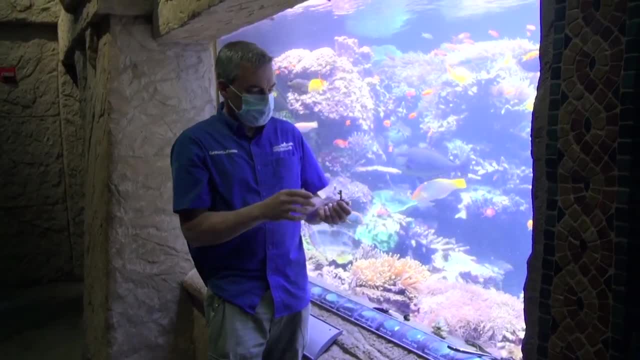 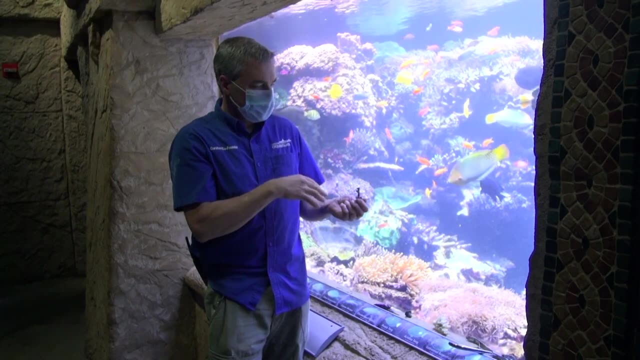 These branching corals get hit by waves and they break apart, And if that little fragment lands in a good spot, it's going to grow into an entire new colony. So that's one of their methods of reproduction is self-fragmentation. 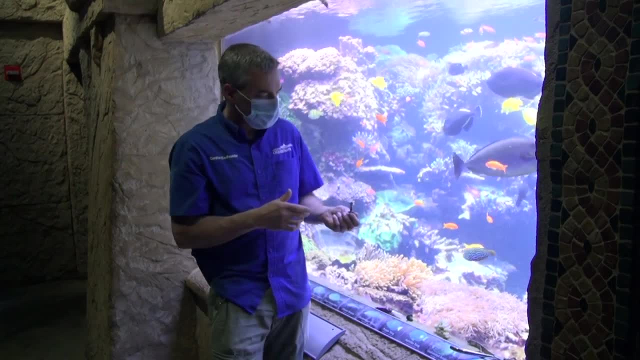 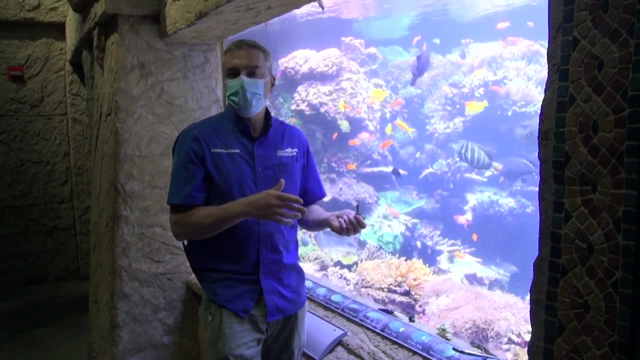 A big fish swimming in, We'll break it into pieces, also Us as humans. that's why you don't want to be dropping your anchors and things like that, because you could really break up a lot of corals. That's bad fragmentation. 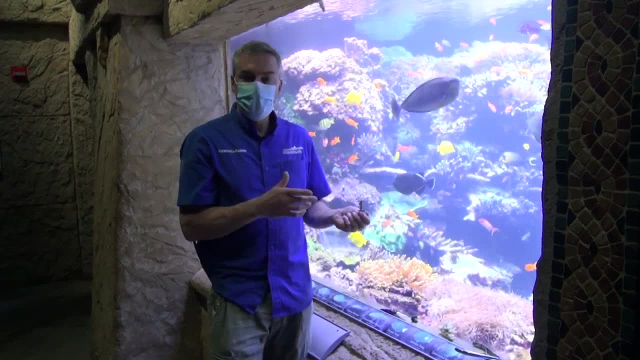 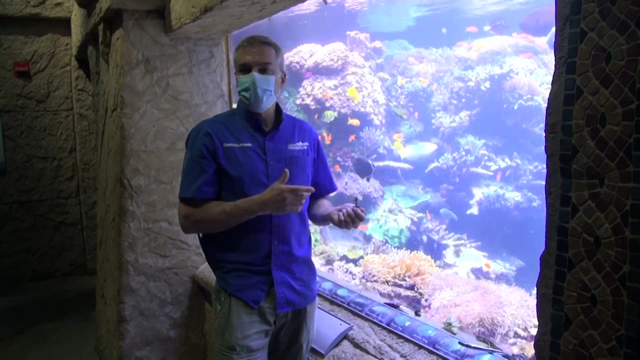 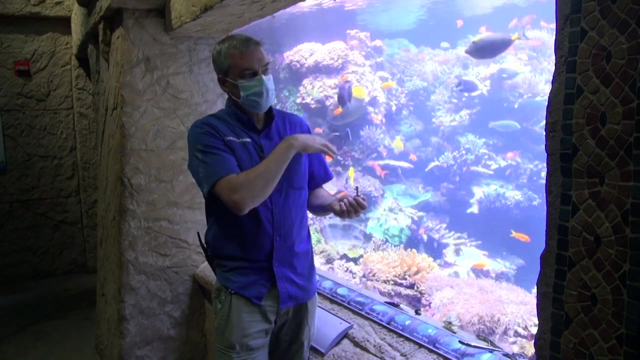 But within the world now, with the ocean temperatures rising, corals are facing huge amounts of stress, both from ocean temperatures, human pollution, different things like that, And what's been interesting through the years of figuring out how to do this stuff within a habitat like this. 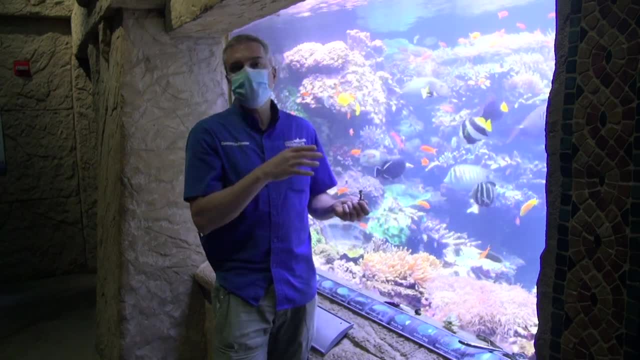 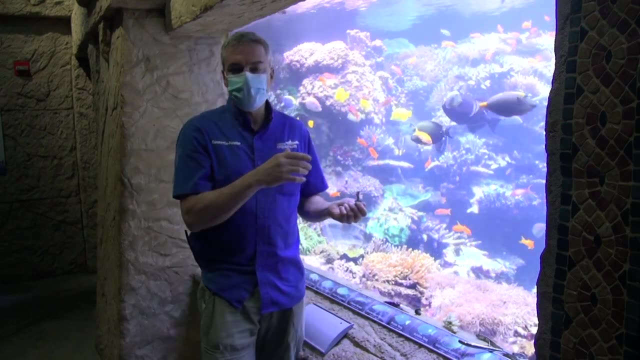 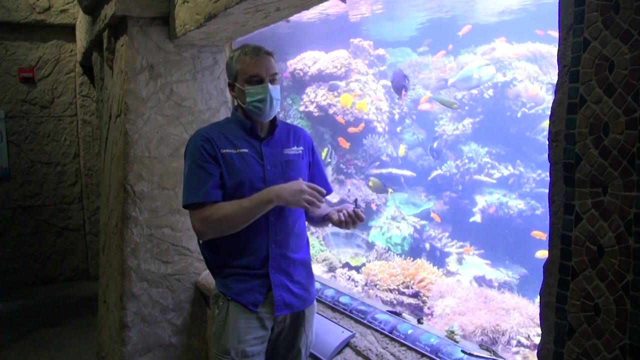 is now. all those things that we've learned in tanks are now being applied to reef restoration. So there's great programs out there down in Florida, the Coral Reef Foundation, the C-Corps International Group- So they'll go out. They'll actively propagate corals, both asexually and sexually. 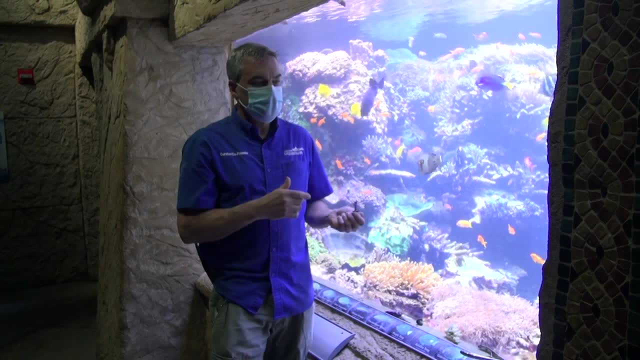 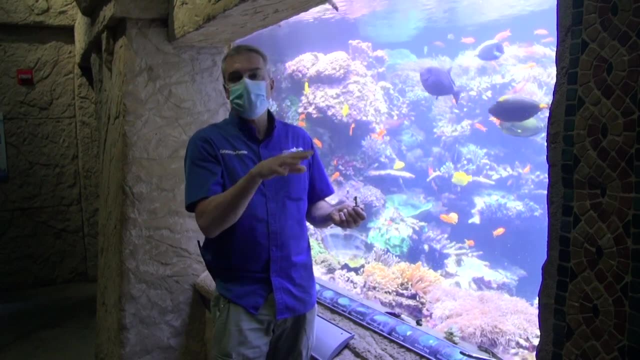 They go out and they will capture the coral spawns, the eggs and the sperm And they'll have the corals settle out. They have a planula stage where they'll swim around And then you can get them to settle out onto little tiles or little plugs like this. 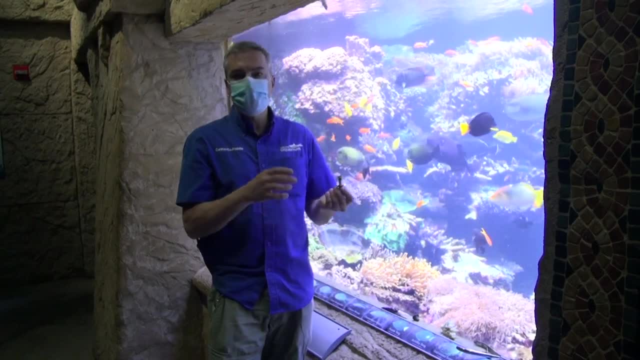 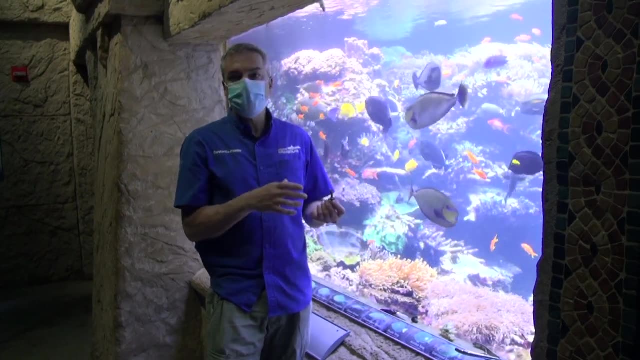 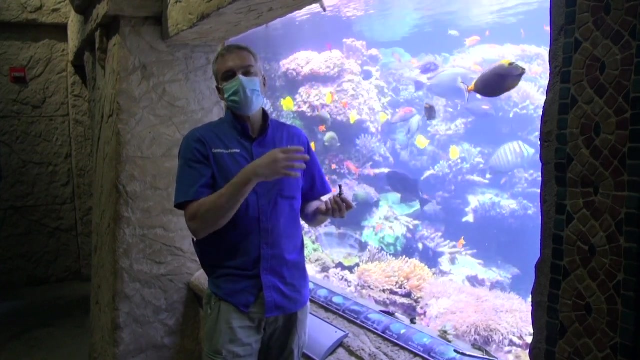 grow them out and then take these and then transplant these back onto the reefs and have the corals grow. So a lot of conservation work has come out of and reef restoration work. The ocean temperatures are rising And, within the same species of coral, certain specimens of those corals. 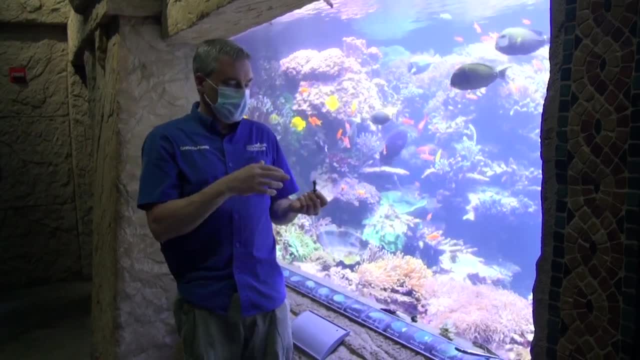 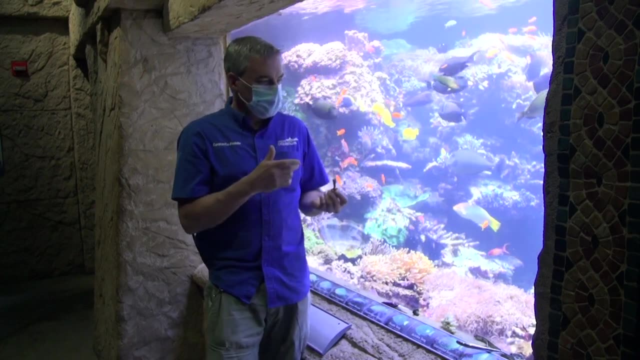 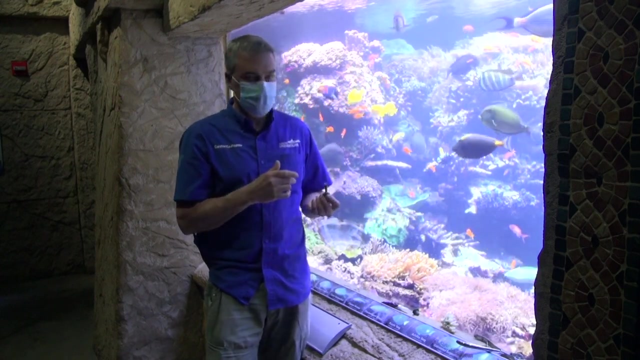 acclimate much better to higher temperature water. So, depending on the algae that's growing in their tissue, some of the algae is more heat tolerant. So now the researchers and scientists are growing and propagating corals that are more heat tolerant, Because independent of your political views, shall we say. 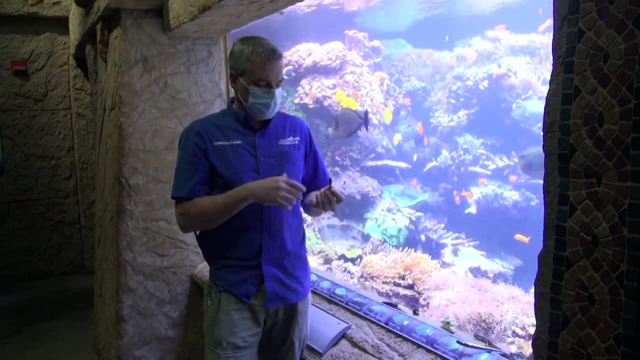 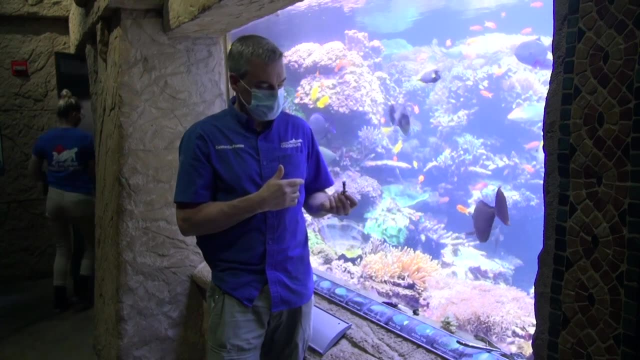 ocean temperatures are on the rise. There's no way around it. So if we can grow corals that are much more heat tolerant, that's much better for the reefs. if it's better for the reefs, then it's better for us. So this is a baby coral. 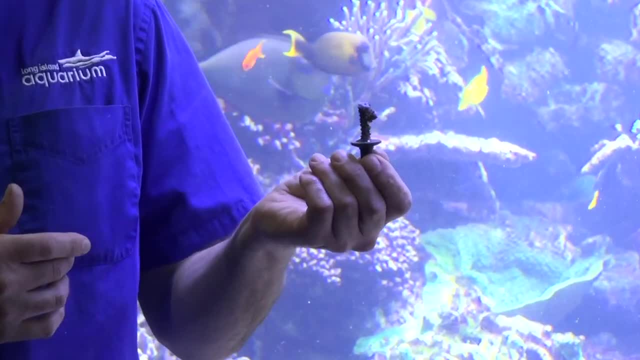 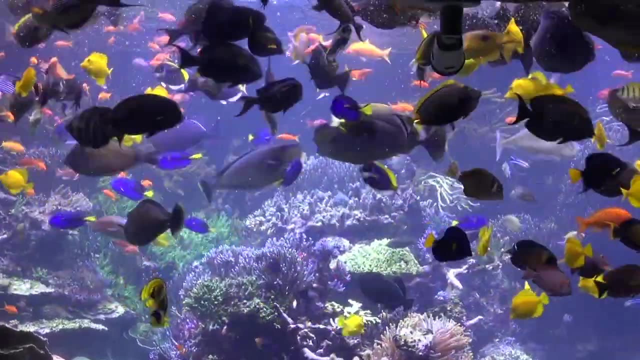 This will grow into a huge colony. So that's how you can fragment a coral. It's that simple. Thank you so much for watching today's episode of our invertebrate biology series. Check it out as Joe feeds the fish in our reef tank- one of the coolest.